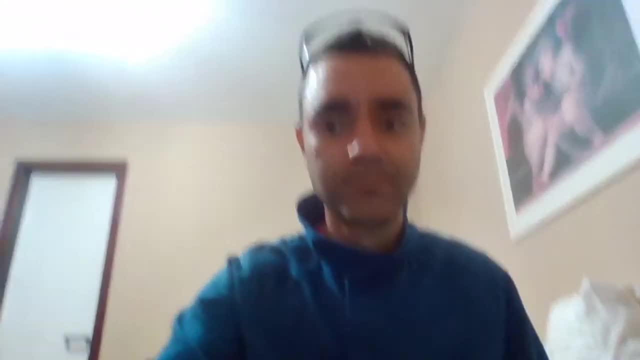 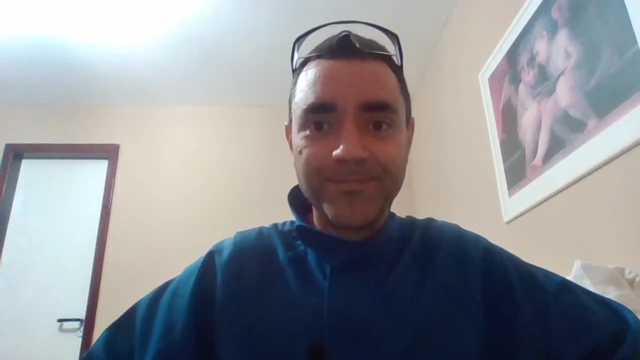 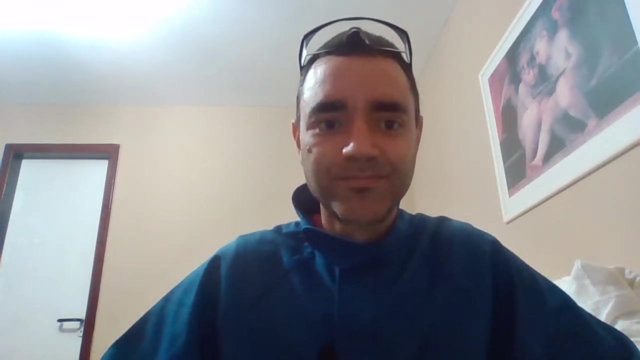 Hello guys, I'm back. My name is Jefferson. I'm a chemical process engineer with expertise in plant design. I will start the live session in some minutes. I just need to share the link to the live session in my telegram channel in my Linkedin. 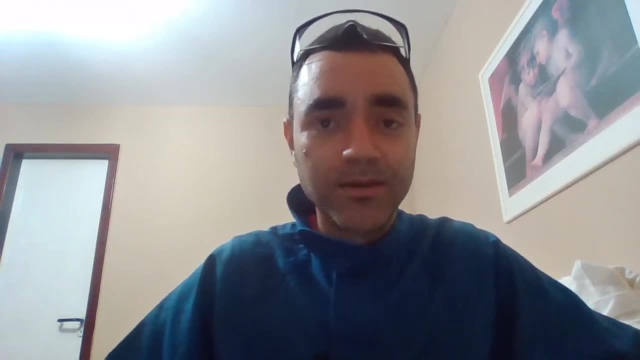 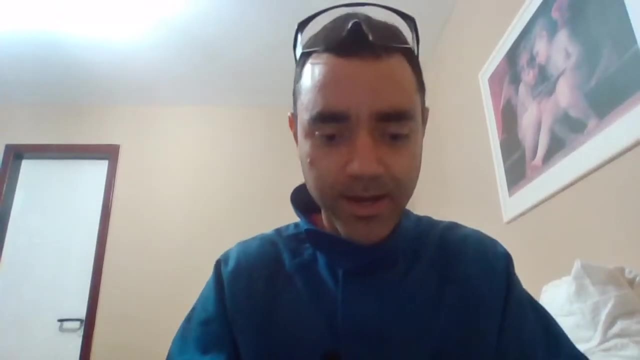 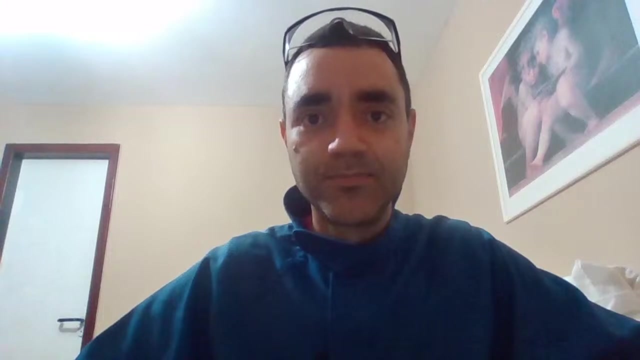 and also in the Facebook. until I do that, please let me know where are you from? I always like to know where are you from usually. usually I have people from India, I have people from Brazil and people from middle and Middle East, and it's very, very nice to know. 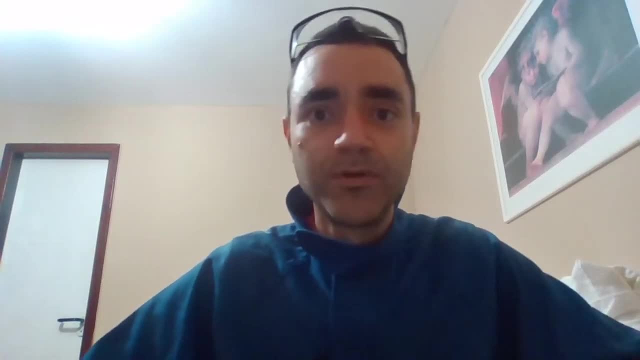 where are you from and you can see if you already follow me in the in the in the live sessions in the social media. I'm not at my home right now. I am at the hotel because I'm doing some field activities. in fact, this live session was. 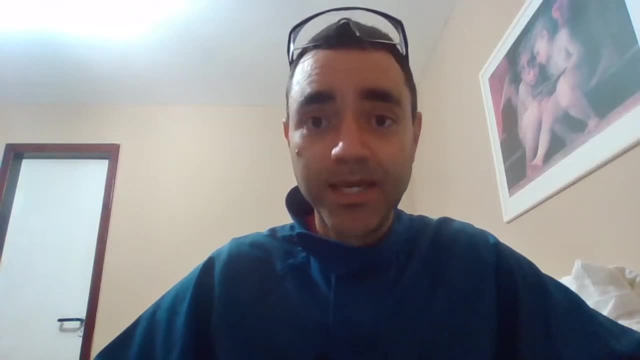 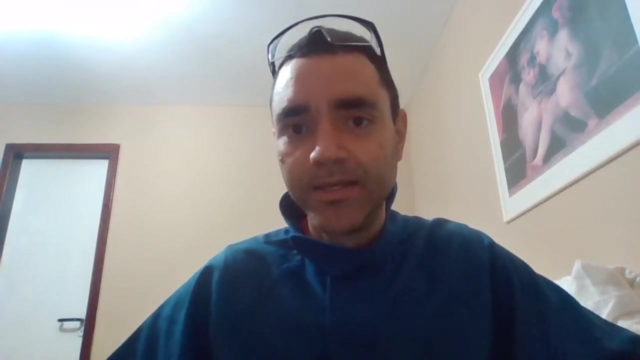 supposed to be at 8: 8, 30 pm here in Brazil, but I stayed at the, the, the field in the Industrial Facility, up to 8 pm, 8 pm, and after that i, i left the, i left the, the plant and, uh, i bought a pizza and i talked. 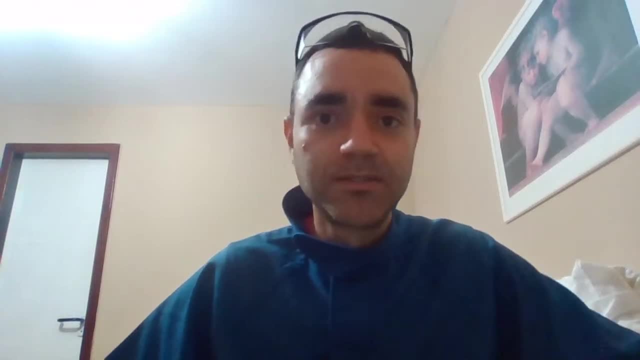 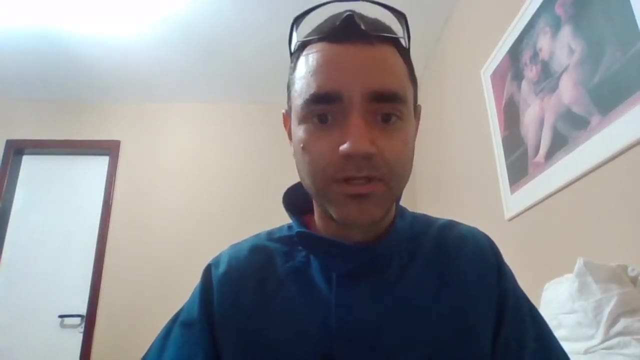 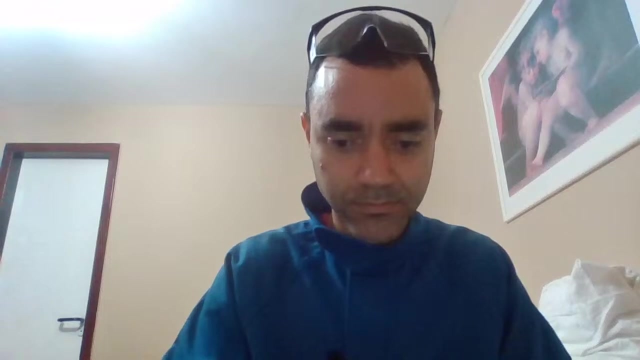 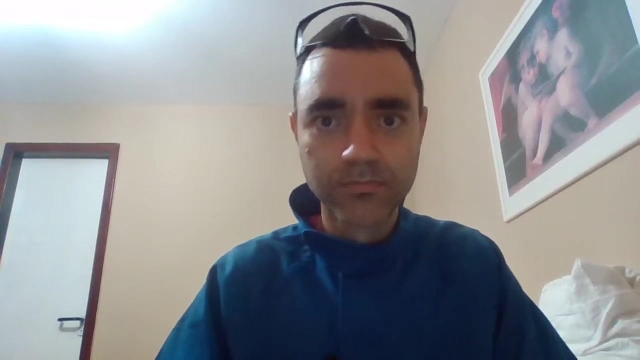 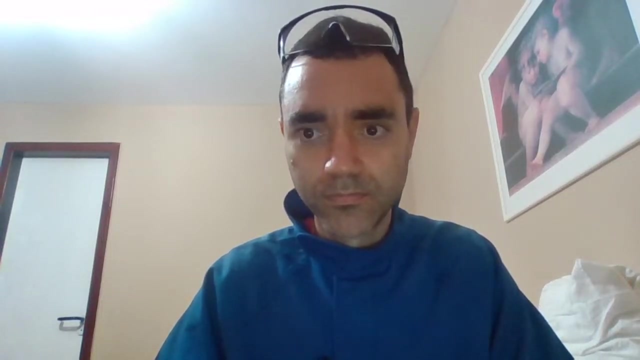 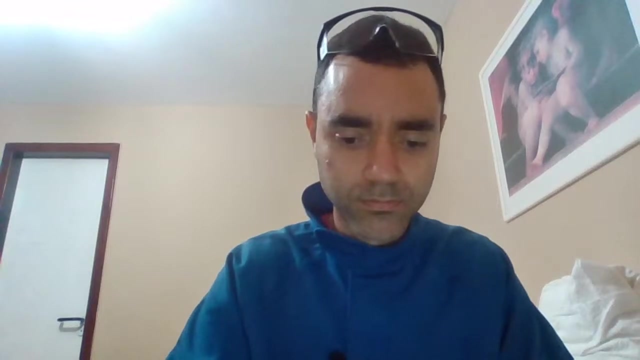 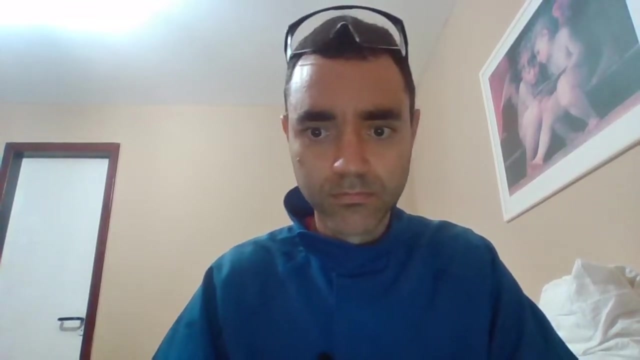 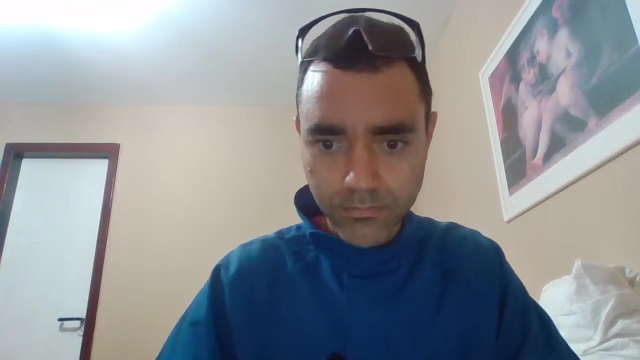 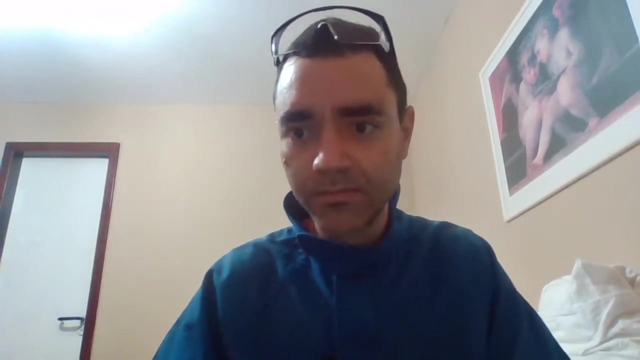 a little bit with my wife and, as i have promised to do this live session, i'm here today and i'm here now, so let me share the links for other people. so, so, so, so, so. okay, i already shared the link to the live. so okay, i already shared the link to the live. 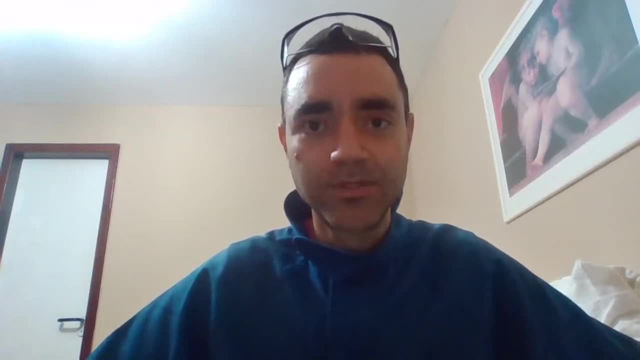 so, okay, i already shared the link to the live session in my facebook, in my linkedin, and session in my facebook, in my linkedin and session in my facebook, in my linkedin and also in my telegram channel, also in my telegram channel, also in my telegram channel, and what i will do here is share some. 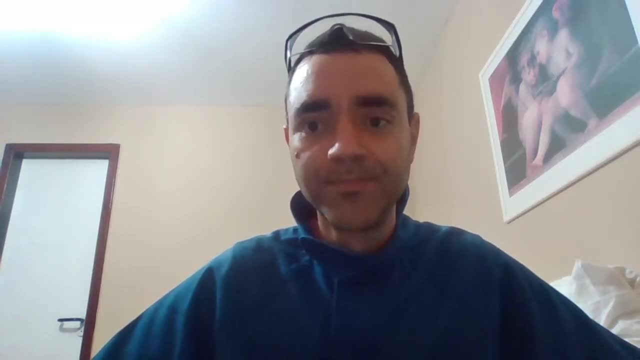 and what i will do here is share some. and what i will do here is share some, some my experience with some, my experience with some, my experience with pressure control, and we'll talk a little pressure control and we'll talk a little pressure control and we'll talk a little bit about that. what i'm doing in the 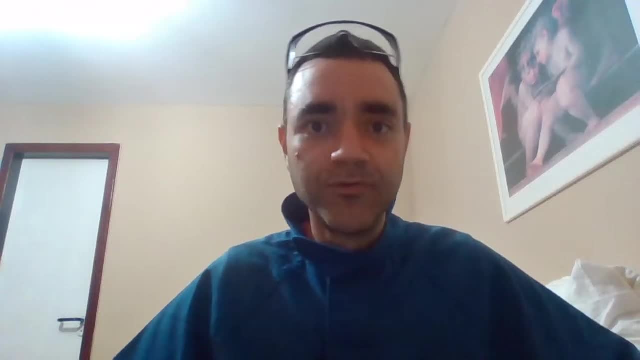 bit about that, what i'm doing in the bit about that, what i'm doing in the field, and this is a little bit different field. and this is a little bit different field, and this is a little bit different than i'm doing every saturday, because on 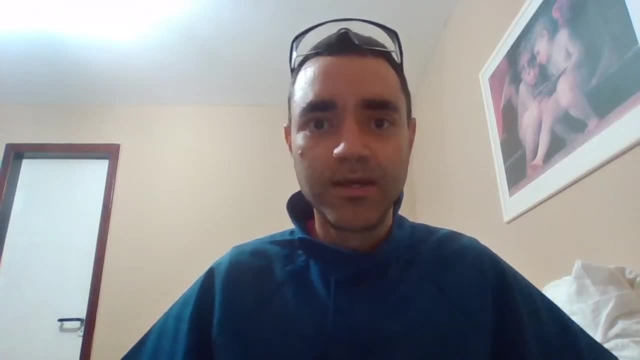 than i'm doing every saturday, because on than i'm doing every saturday? because on every saturday i have a guest where i, every saturday i have a guest where i, every saturday i have a guest where i talk, talk, talk, uh, about a subject related to chemical. 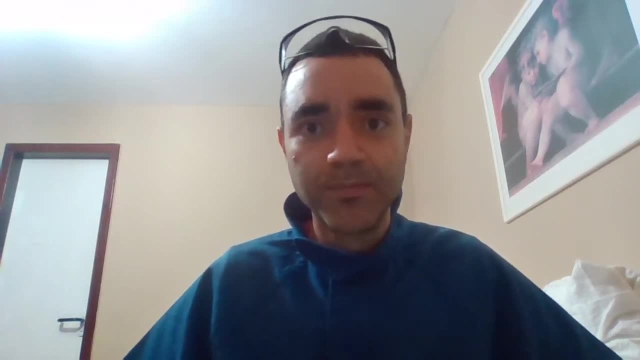 uh about a subject related to chemical? uh about a subject related to chemical process engineering plan: design, process engineering plan design process engineering plan design. and today i'm i'm here alone and you can, and today i'm i'm here alone and you can, and today i'm i'm here alone and you can see that i'm still in the suit. 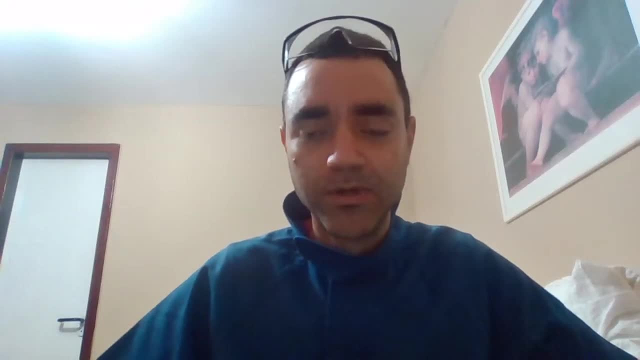 see that i'm still in the suit. see that i'm still in the suit. i didn't take a shower because it was. i didn't take a shower because it was. i didn't take a shower because it was my commitment to you to not lose this. 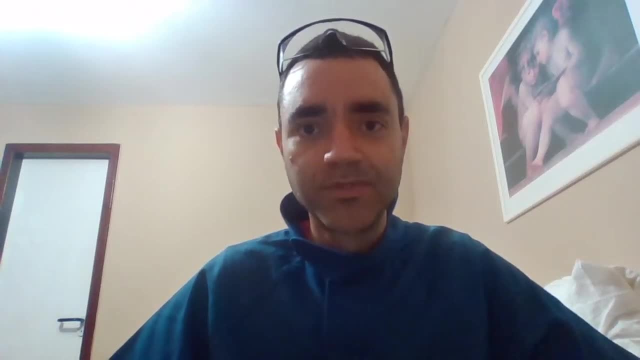 my commitment to you to not lose this, my commitment to you to not lose this, this live session, because i left this live session, because i left this live session, because i left later than i supposed to to be left in, later than i supposed to to be left in. 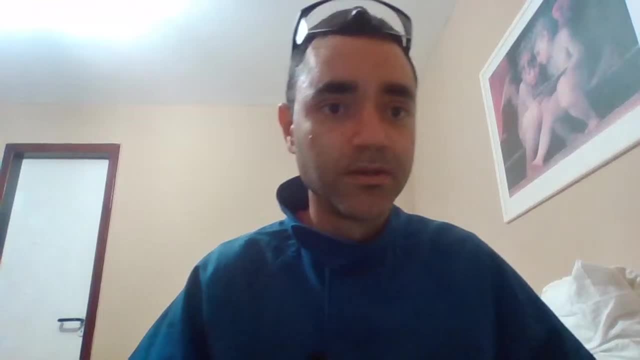 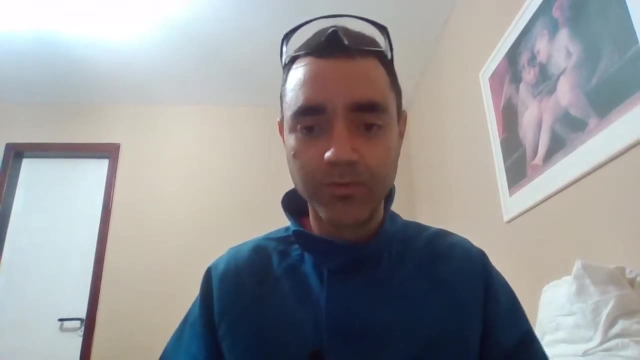 later than i supposed to, to be left in the, the industrial plant, the, the industrial plant, the, the industrial plant, so so, so i will try, i will try, i will try to to to. i'm today, i'm only with one screen and i'm. i'm today, i'm only with one screen and i'm. 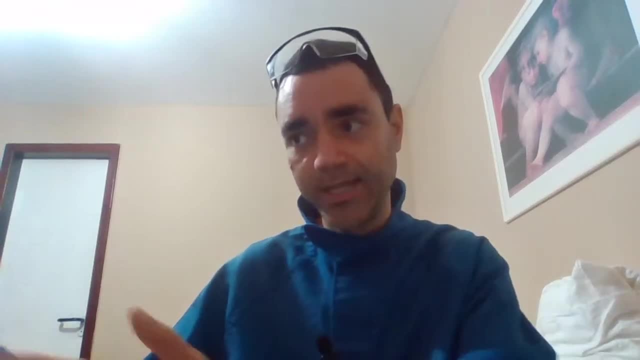 i'm today, i'm only with one screen and i'm only with my notebook. usually i have only with my notebook. usually i have only with my notebook. usually i have another screen at my right side, another screen at my right side, another screen at my right side when i'm doing the, the live session at 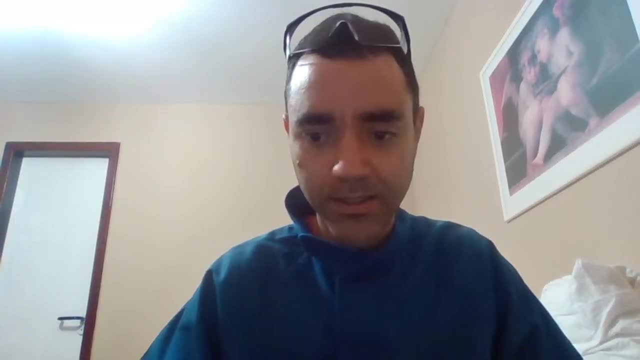 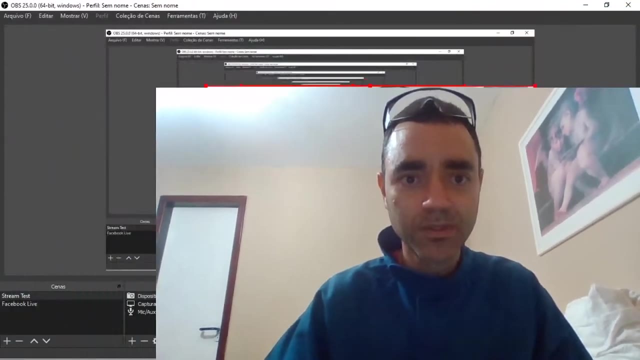 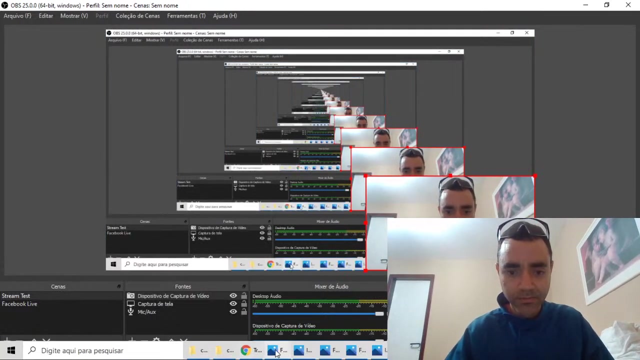 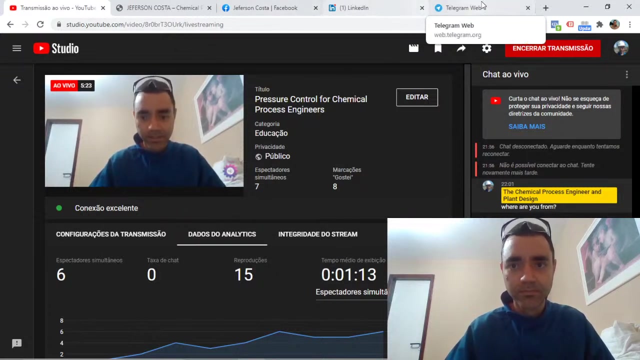 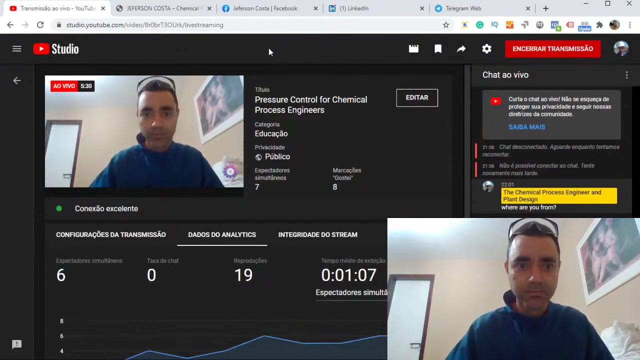 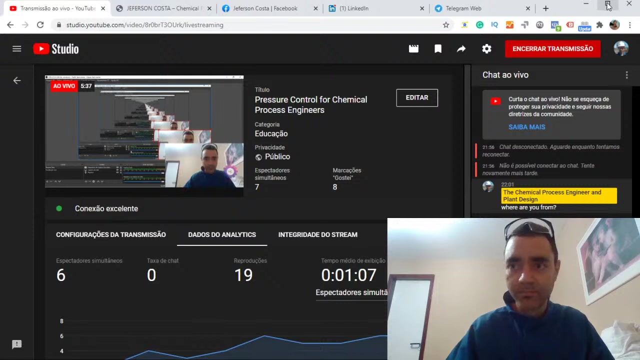 when i'm doing the the live session at, when i'm doing the the live session at home, home, home. so let's see how i can, so let's see how i can, so let's see how i can start sharing content with you. okay, okay, i wanna see. 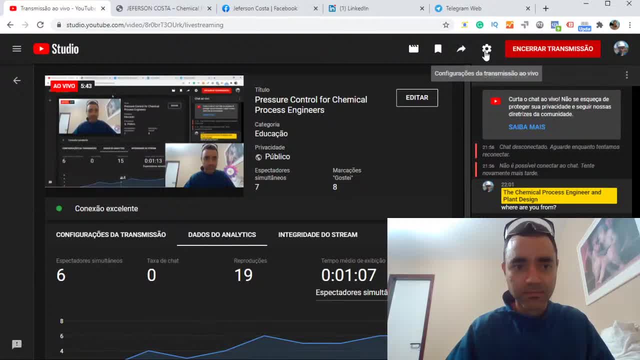 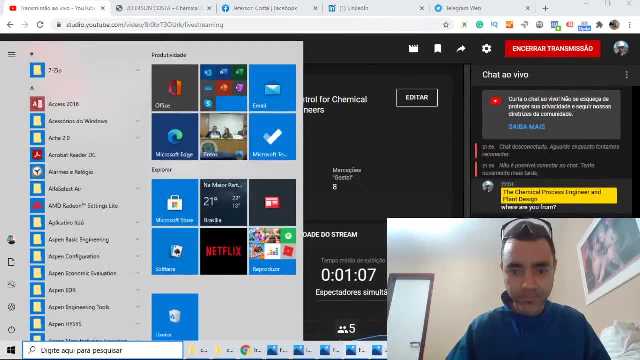 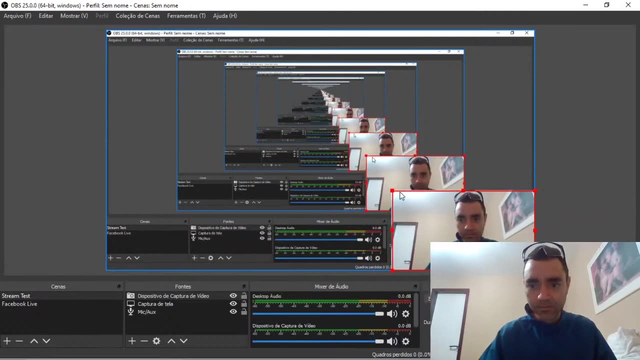 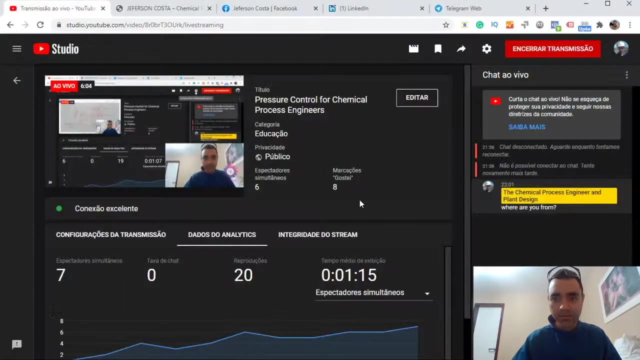 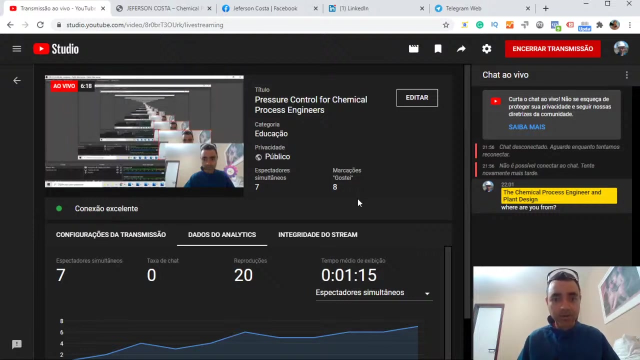 i wanna see, i wanna see my now okay, now okay, now okay, so, now okay. so i will follow the chat. i will follow the chat. i will follow the chat by my cell phone, by my cell phone, by my cell phone. okay, sorry for this disturbance, but guys, no. 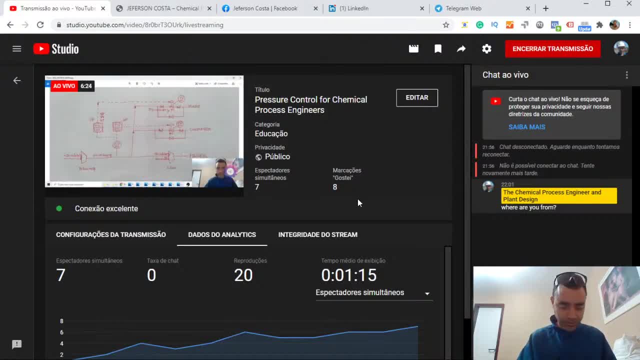 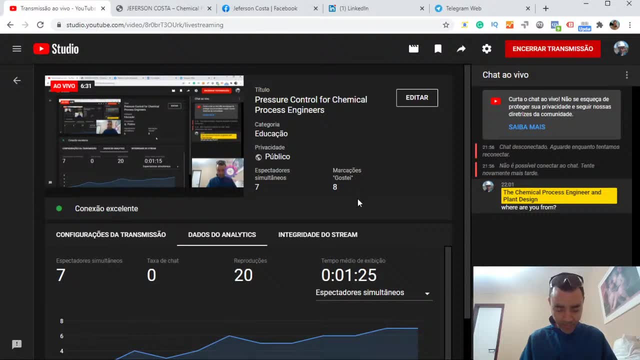 sorry for this disturbance, but guys, no, sorry for this disturbance, but, guys, no one, one one told me where are you from. so please told me, where are you from. so please told me where are you from. so please interact with me, interact with me, interact with me. it is 10 pm in brazil and i would 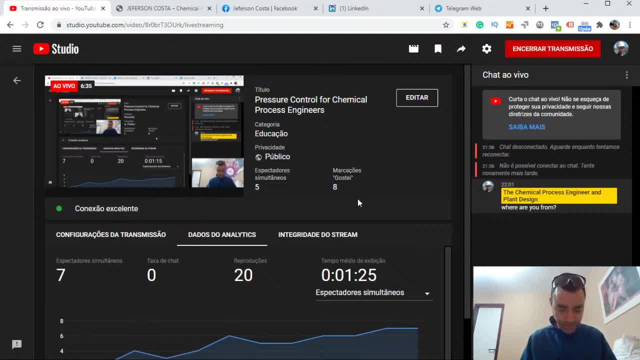 it is 10 pm in brazil and i would- it is 10 pm in brazil and i would appreciate to have some kind of appreciate, to have some kind of appreciate, to have some kind of interaction to with you, interaction to with you, interaction to with you, because, uh, 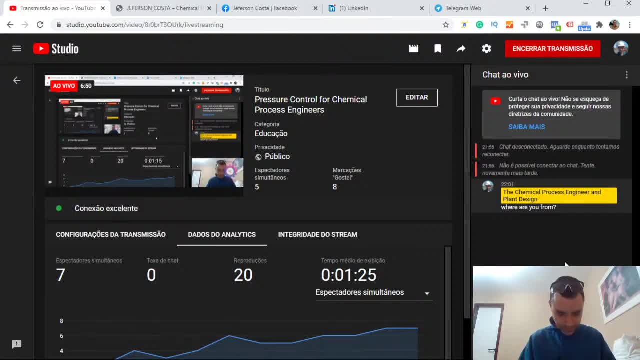 my chat is not working. my chat is not working. my chat is not working, okay, okay. so now i'm with the, so now i'm with the. so now i'm with the. the cell phone, and it will be easy to me, the cell phone, and it will be easy to me. 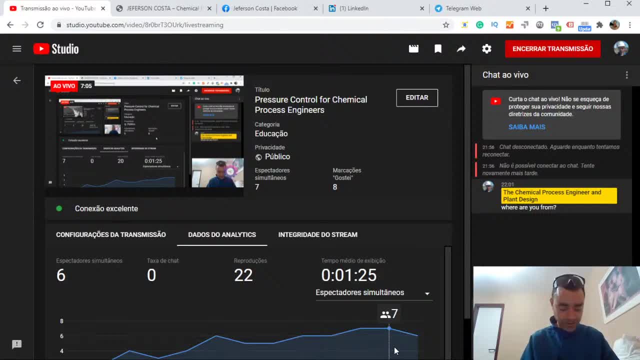 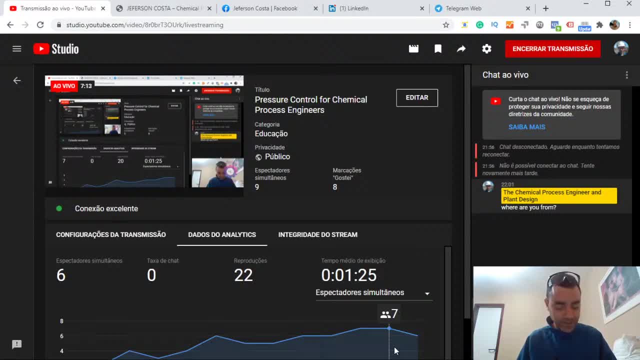 talking to me. so i have everton and have it from atibaya, sao paulo, brazil, have it from atibaya, sao paulo, brazil. have it from atibaya, sao paulo, brazil, and everton. i think this everton and everton, i think this everton. 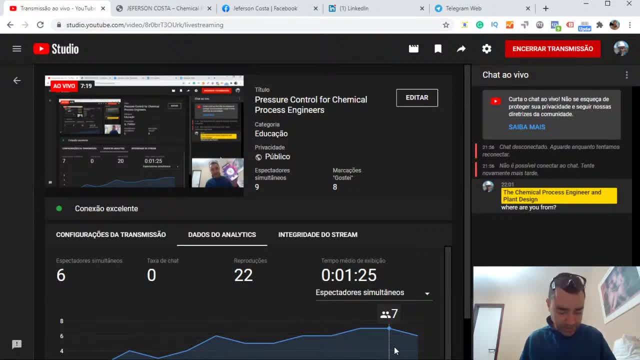 and everton. i think this everton i'm not so sure if he is my friend, i'm not so sure if he is my friend, i'm not so sure if he is my friend, because it is abbreviated here i have. because it is abbreviated here i have. 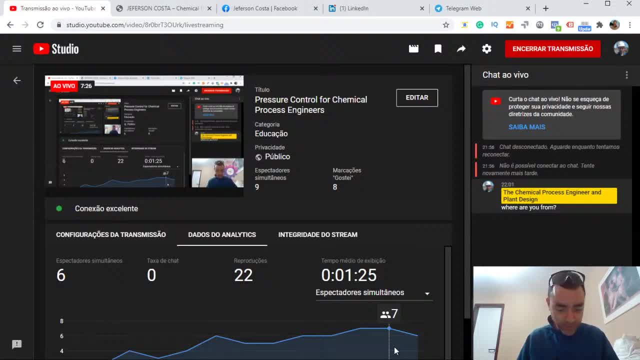 because it is abbreviated. here i have also also also joshuel cordova, carlos. hi guys here from joshuel cordova, carlos. hi guys here from joshuel cordova, carlos. hi guys here from lima, peru, lima, peru, lima, peru. uh nice, nice to have you here, just. 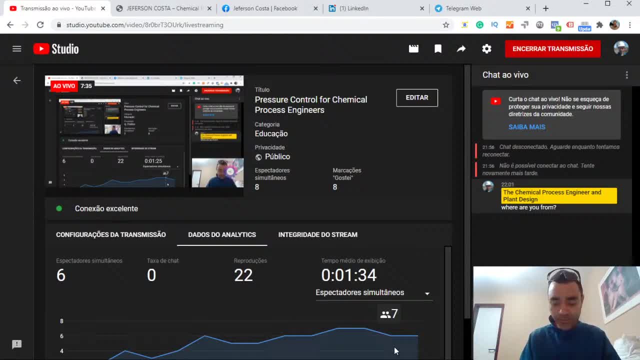 uh, nice nice to have you here. just uh nice nice to have you here. just just mail, i just mail, i just mail. i expand some some months in in lima, peru. expand some some months in in lima, peru. expand some some months in in lima, peru. in fact it was in. 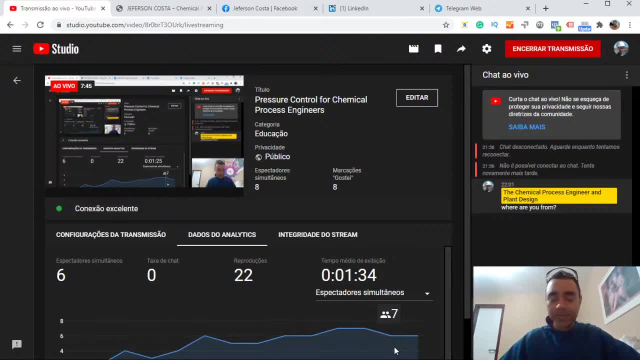 in fact it was in. in fact it was in in calhau starting up a hydrogen plant in calhau, starting up a hydrogen plant in calhau, starting up a hydrogen plant in calhau for for repsoul. so i spent in calhau for for repsoul, so i spent. 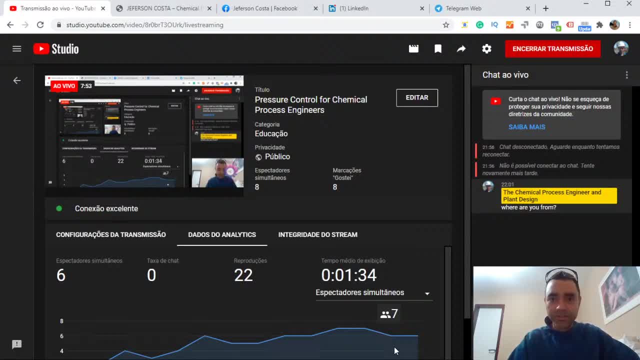 in calhau for for repsoul. so i spent some, some, some, some months there, and mira flores is very, very months there and mira flores is very, very months there, and mira flores is very, very beautiful, beautiful, beautiful. i have actually partio from india and 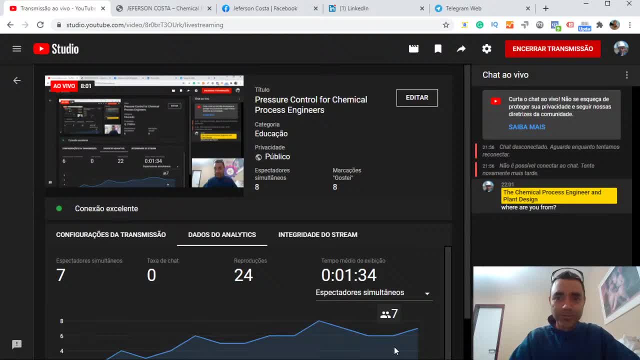 i have actually partio from india and i have actually partio from india and thanks a lot, thanks a lot, thanks a lot actually for being here. actually is one of actually for being here. actually is one of actually for being here. actually is one of my students in the. 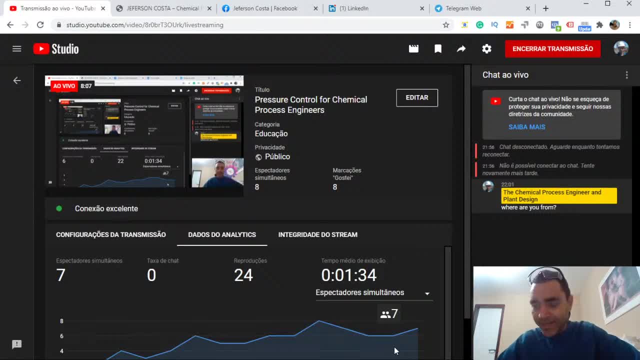 my students in the, my students in the in-process booster training program and in-process booster training program and in-process booster training program and my dear friend chemical engineering guy, my dear friend chemical engineering guy, my dear friend chemical engineering guy is he also thanks for giving a. 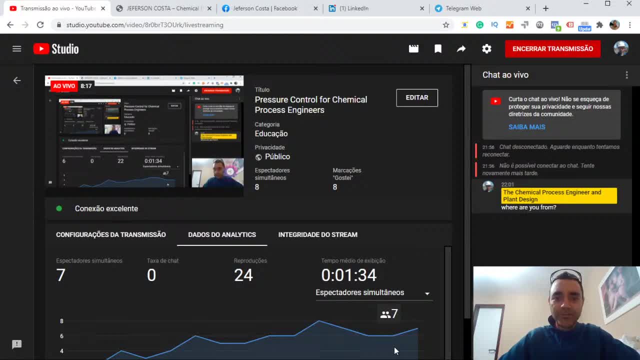 is he also thanks for giving a? is he also thanks for giving a? hi, hi, hi, emmanuel, and if you, emmanuel, and if you, emmanuel, and if you want to know more about aspen plus, want to know more about aspen plus, want to know more about aspen plus. and the chemical engineering guy is the. 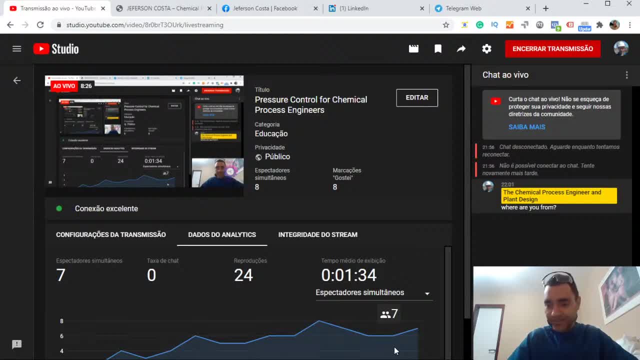 and the chemical engineering guy is the. and the chemical engineering guy is the best guy that i know to help you with, best guy that i know to help you with. best guy that i know to help you with that. that that, ah, everton, thanks, everton. everton is a. 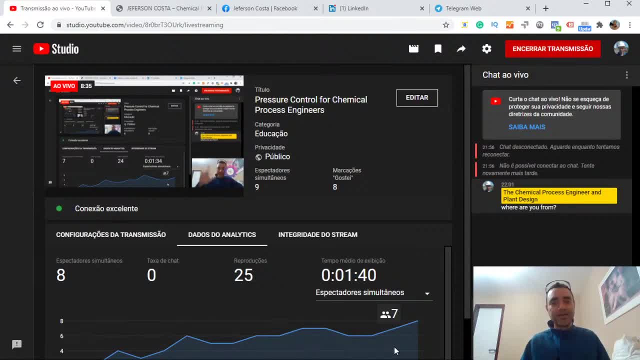 ah everton, thanks everton. everton is a. ah everton, thanks everton. everton is a friend of mine. he was one of my guests. friend of mine. he was one of my guests. friend of mine. he was one of my guests in a previous, in a previous. 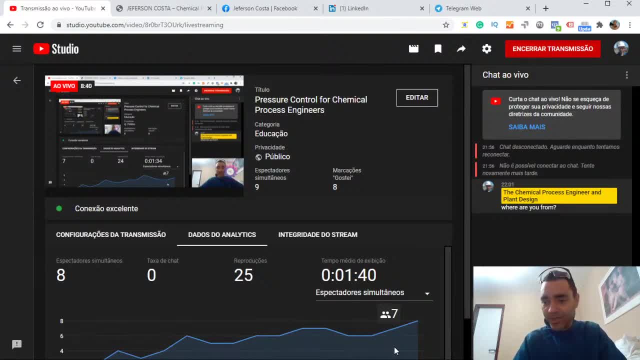 in a previous, webinars that i did online and it's very webinars that i did online and it's very webinars that i did online and it's very nice to have you here. nice to have you here, nice to have you here with me. so, guys, let me share. 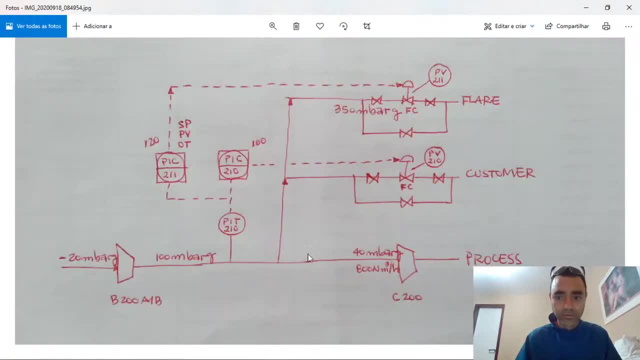 with me. so, guys, let me share with me. so, guys, let me share what let me, starting with i want to, what let me, starting with i want to, what let me starting with i want to, to say to you so what i i to say to you, so what i i. 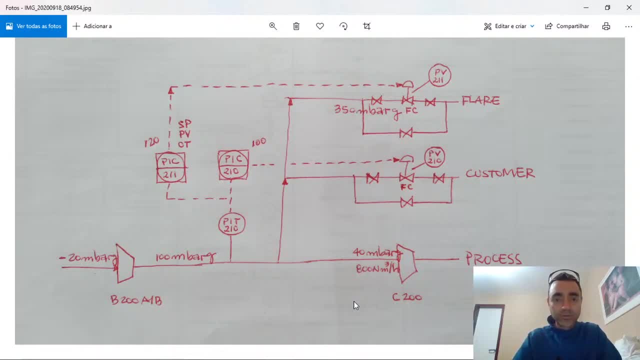 to say to you: so what i i will discuss with you today is about, will discuss with you today is about: will discuss with you today is about control loops and and pressure control control loops and and pressure control control loops and and pressure control, or something like that. so we 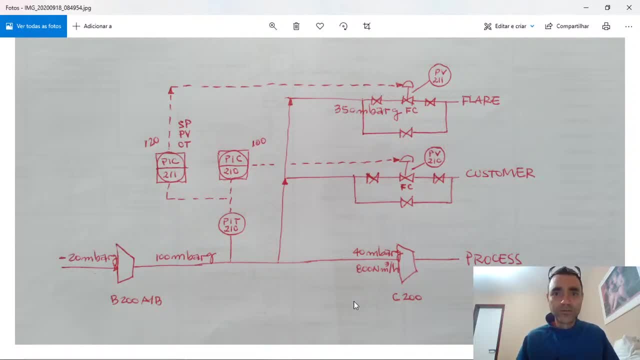 or something like that, so we, or something like that, so we, i will do. i will talk to you about some. i will talk to you about some. i will talk to you about some general information about that. what kind general information about that? what kind general information about that? what kind of information we? 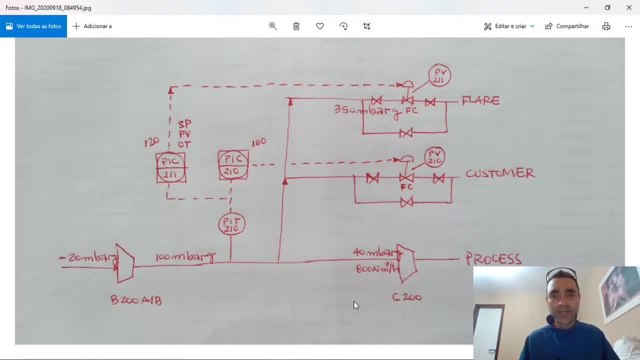 of information, we of information, we we need why we do that and what kind of we need, why we do that and what kind of we need, why we do that and what kind of deliverables is involved, and with that deliverables is involved and with that deliverables is involved, and with that, my plan is that to get more familiar. 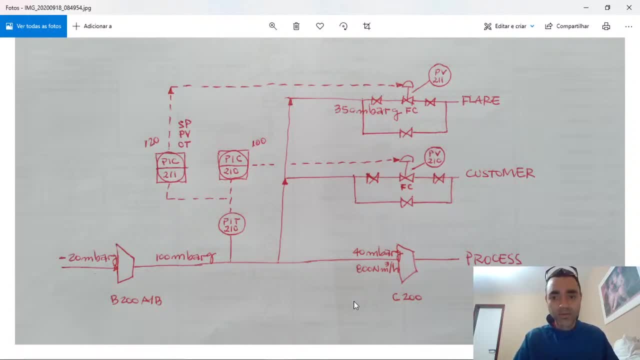 my plan is that to get more familiar. my plan is that to get more familiar with this kind of control, with this kind of control, with this kind of control, and let's see how it's it's will will go, and let's see how it's it's will will go. 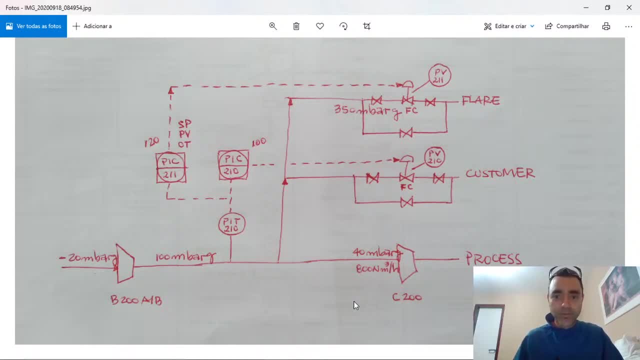 and let's see how it's it's will will go, so so. so the first thing is: uh, let's start with. the first thing is: uh, let's start with. the first thing is: uh, let's start with the problem that i have here and what i'm. 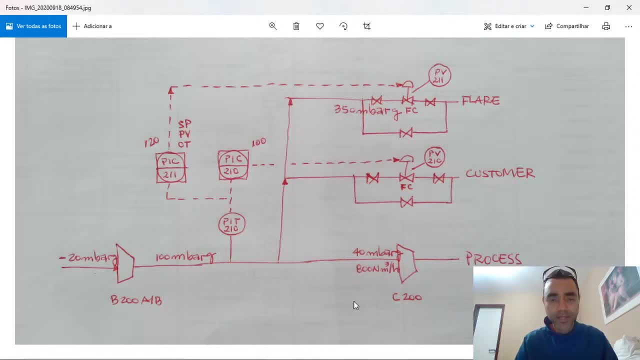 the problem that i have here and what i'm the problem that i have here and what i'm working on, working on, working on here in the field. i spending more than one here in the field. i spending more than one here in the field. i spending more than one week. 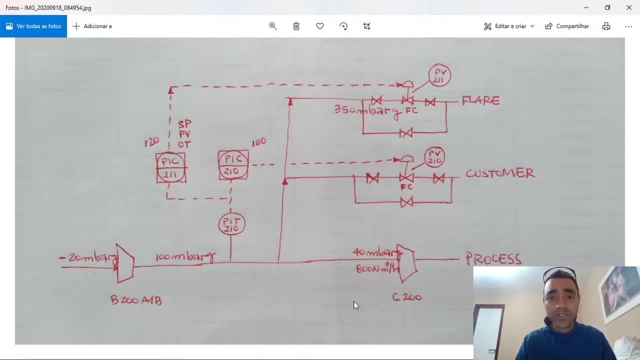 week week, here in, in, here in, in, here in in in rio de janeiro, to rio de janeiro, to rio de janeiro, to to do the commissioning of a new, to do the commissioning of a new, to do the commissioning of a new pipeline to the customer. 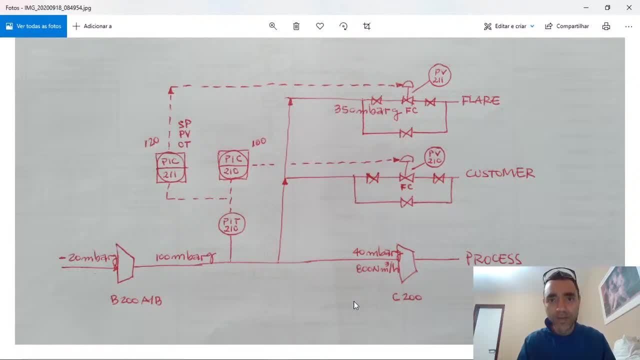 pipeline to the customer, pipeline to the customer, and there there is not much issues, uh, and there there is not much issues, uh, and there there is not much issues, uh, about this new pipeline. um, but we need, uh, the team needs to do, um, but we need, uh, the team needs to do. 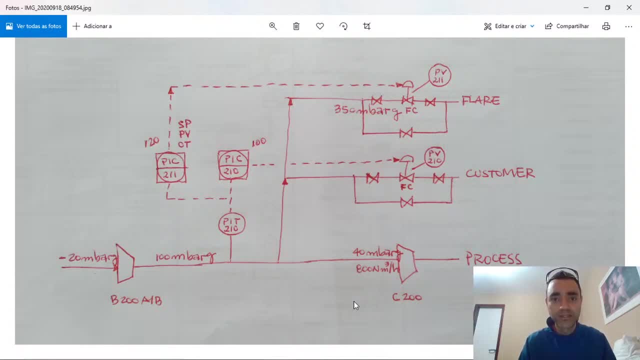 um, but we need, uh, the team needs to do the, the tuning of the control valves and the, the tuning of the control valves and the, the tuning of the control valves, and that's depending on the, the control that's depending on the, the control that's depending on the, the control that the customer is doing at his side. 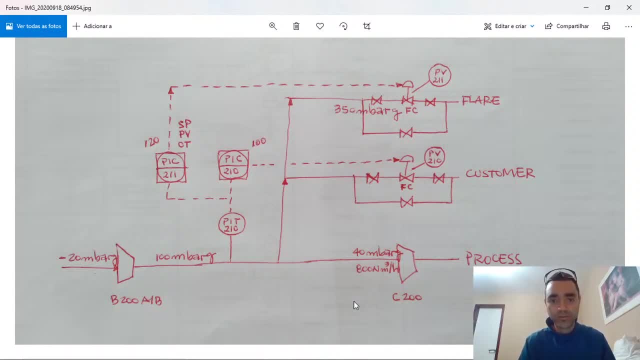 that the customer is doing at his side, that the customer is doing at his side, and the the big challenge is to and the the big challenge is to and the the big challenge is to is to integrate that, because once he is to integrate that, because once he 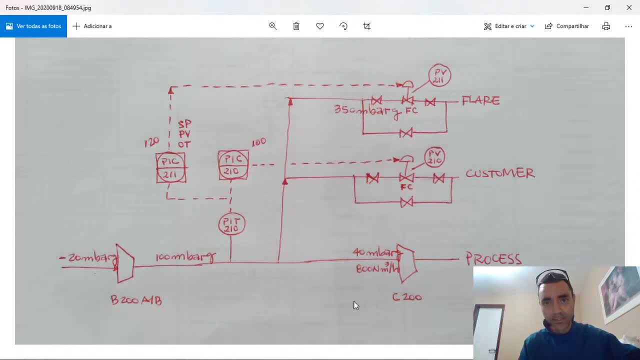 is to integrate that, because once he has a blower at his side at the battery, has a blower at his side at the battery, has a blower at his side at the battery limit of limit of limit of of his and one the blower, his and one the blower. 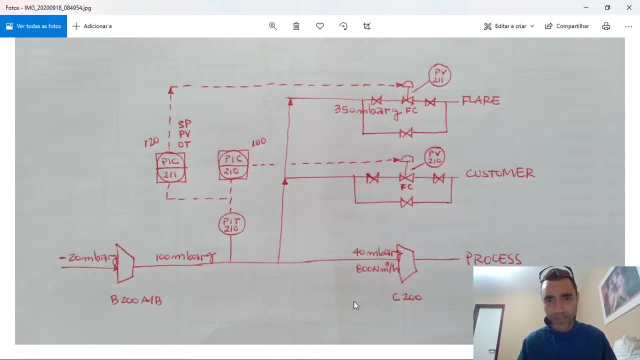 his and one, the blower, uh uh, uh, loads and unload. it affects my plant. so loads and unload. it affects my plant. so loads and unload, it affects my plant. so the uh, the main issue today. the uh, the main issue today. the uh, the main issue today. that's why i left so so late from the. 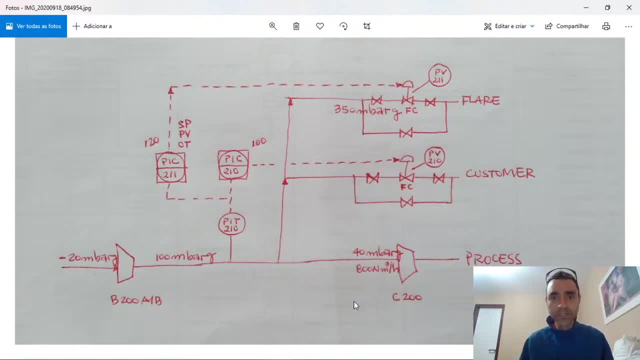 that's why i left so so late from the. that's why i left so so late from the. from the plant, from the plant, from the plant. but in general terms, what is this process? but in general terms, what is this process? but in general terms, what is this process? i have a, a blower that. 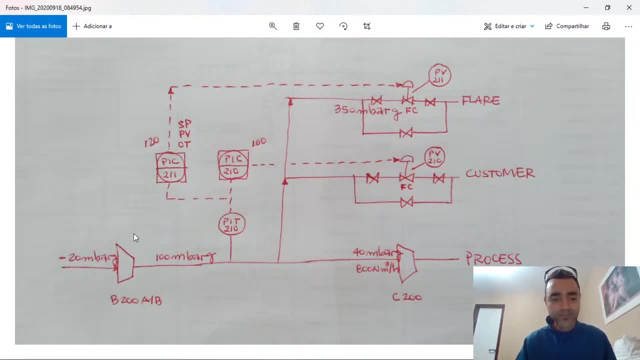 i have a a blower that i have a a blower that that gets. that gets biogas from the landfill and this biogas from the landfill and this biogas from the landfill and this biogas- biogas from the landfill- and this biogas is compressed in order to give the 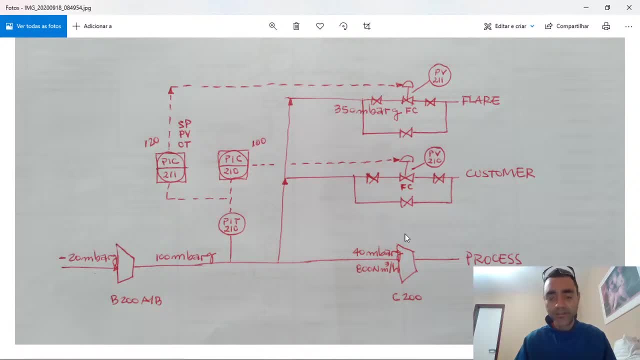 is compressed in order to give the is compressed in order to give the minimum pressure at the compressor. that minimum pressure at the compressor, that minimum pressure at the compressor, that will compress that to around seven bar g, will compress that to around seven bar g, will compress that to around seven bar g and send it to the process plant and in 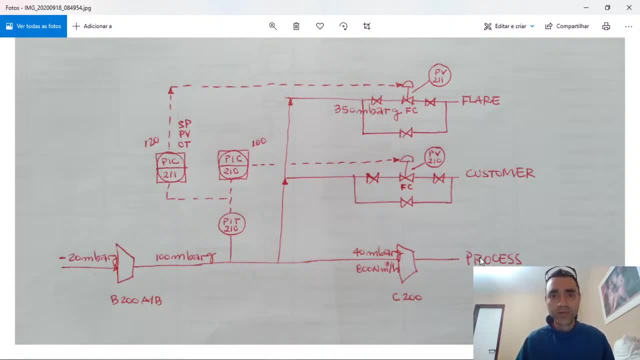 and send it to the process plant and in and send it to the process plant and in this process plant i will remove the co2. this process plant, i will remove the co2. this process plant, i will remove the co2, i will remove hos and in the end i will. 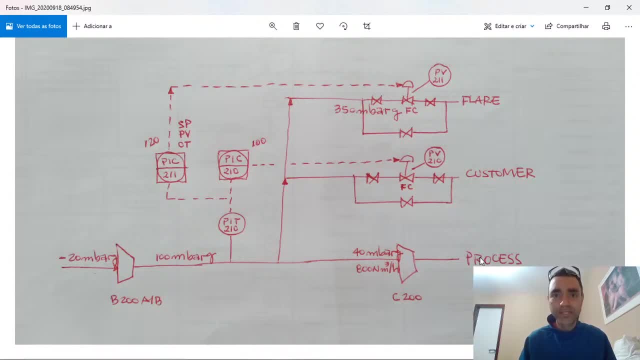 i will remove hos and in the end i will. i will remove hos and in the end i will be able to have be able to have be able to have biomethane ready to fuel trucks to the, biomethane ready to fuel trucks to the biomethane ready to fuel trucks to the to the market. 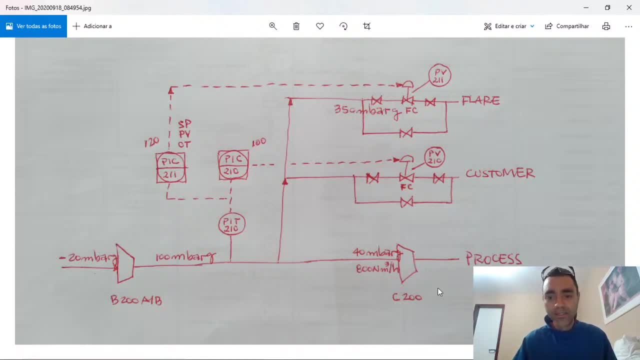 to the market, to the market and, and, and eventually, when, the, eventually, when, the, eventually, when the the compressor stops and there are some the compressor stops and there are some the compressor stops and there are some events that stops not only the compressor events that stops not only the compressor. 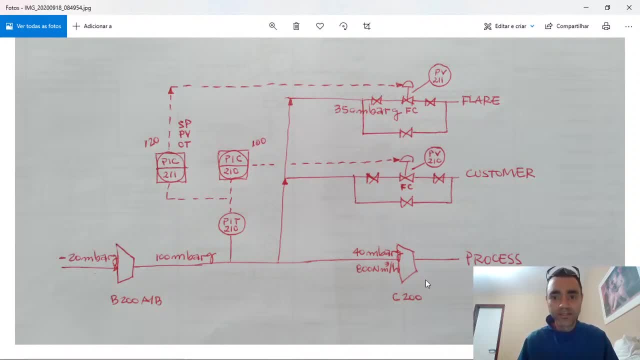 events. that stops not only the compressor, but also, but also, but also, the, the purification plant, and the, the purification plant, and the the purification plant, and in the, in the, in the. in this unit, i need to, in this unit, i need to, in this unit, i need to- to release these, these gas to. 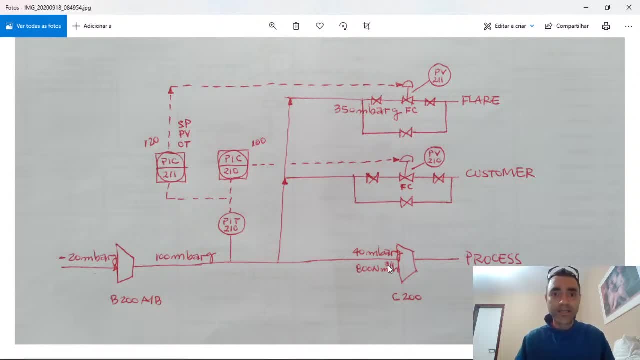 to release these, these gas to, to release these, these gas to atmos, atmos, atmos. i, i need to release this gas. i cannot, i, i need to release this gas. i cannot, i, i need to release this gas. i cannot just shut down the blower and just shut down the blower and 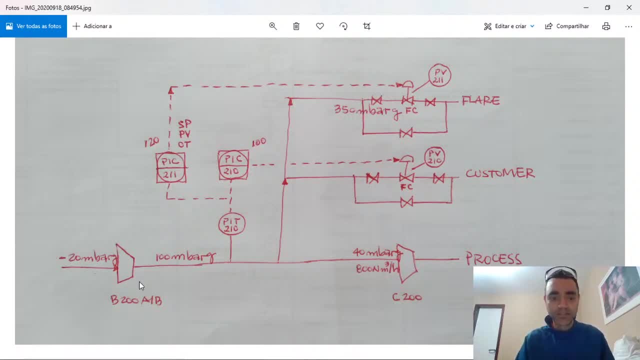 just shut down the blower and prevent from taking the gas from the, prevent from taking the gas from the, prevent from taking the gas from the landfill. because landfill, because landfill, because in the landfill the biomethane is in the landfill, the biomethane is in the landfill, the biomethane is produced by 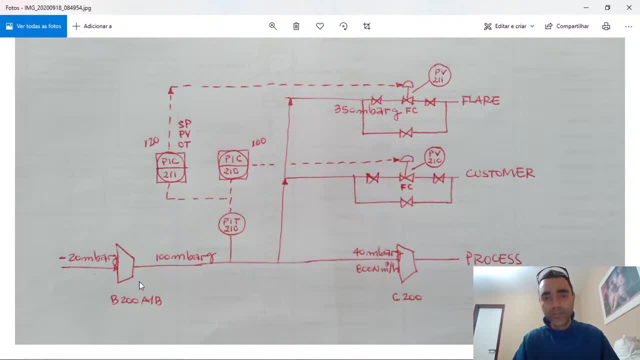 produced by, produced by microorganisms and the. if the pressure microorganisms and the, if the pressure microorganisms and the, if the pressure there there there, increases, it affects the efficiency of increases. it affects the efficiency of increases. it affects the efficiency of the landfill. so, because of that, 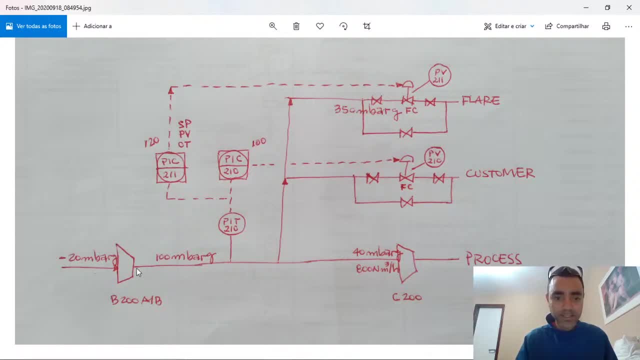 the landfill. so, because of that, the landfill. so because of that, if my compressor stops, i instead of if my compressor stops, i instead of if my compressor stops, i, instead of sending the gas to the, sending the gas to the, sending the gas to the compressor, i need to send this gas to the. 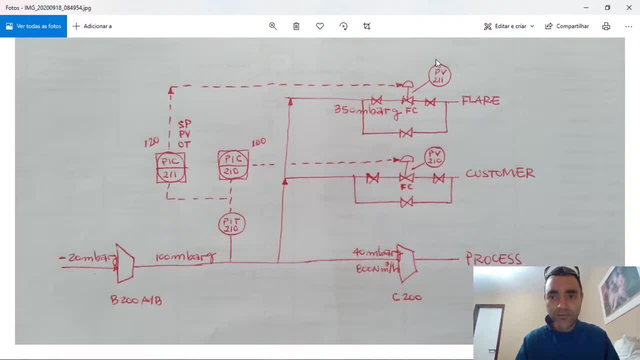 compressor. i need to send this gas to the compressor. i need to send this gas to the flare, flare, flare, and that's why i have a pv here, and that's why i have a pv here, and that's why i have a pv here, why i have a pv and not. 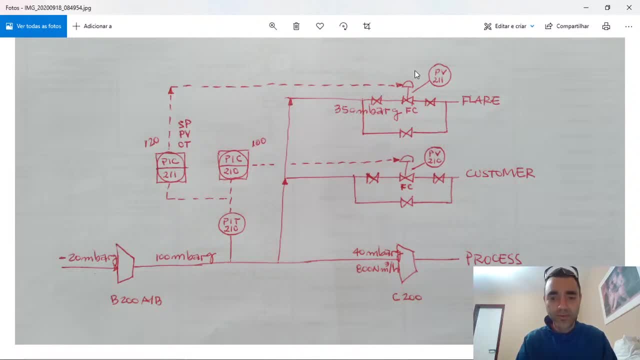 why i have a pv and not why i have a pv and not a tv or not a tv, or not a tv or not fv. so the first thing to that we fv. so the first thing to that we fv. so the first thing to that we that you should get familiar is with the 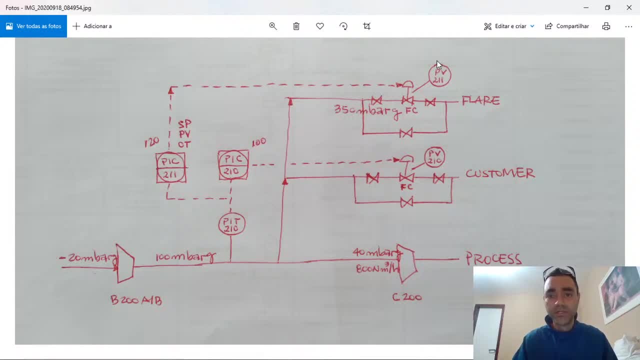 that you should get familiar is with the that you should get familiar is with the nomin nomenclature that we use during. nomin nomenclature that we use during nomin nomenclature that we use during in control. so the the main source of in control. so the the main source of. 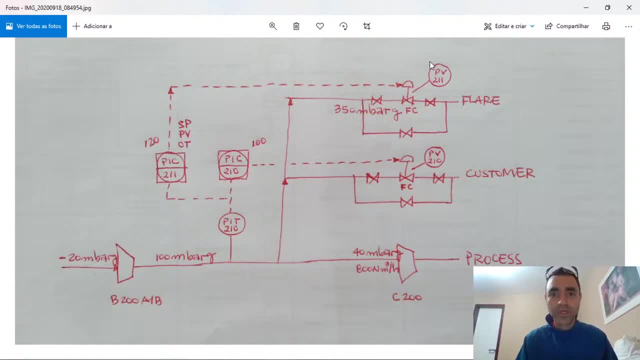 in control. so the, the main source of uh uh uh, the main source of information to you, will the main source of information to you, will the main source of information to you will be the, the pnid, be the, the pnid, be the, the pnid symbol chart. but we can. 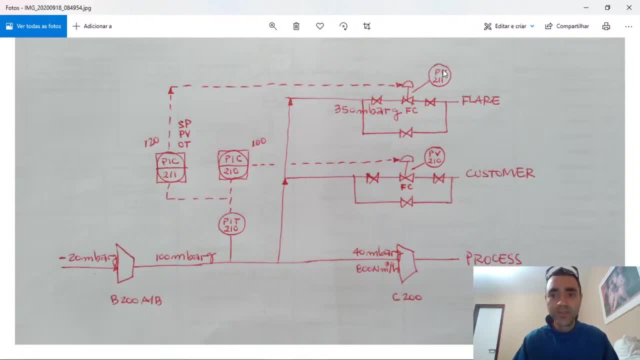 symbol chart. but we can symbol chart, but we can, we can evaluate and we can predict that we can evaluate and we can predict that we can evaluate and we can predict that pv means pv means pv means pressure valve and this pressure valve, pressure valve and this pressure valve. 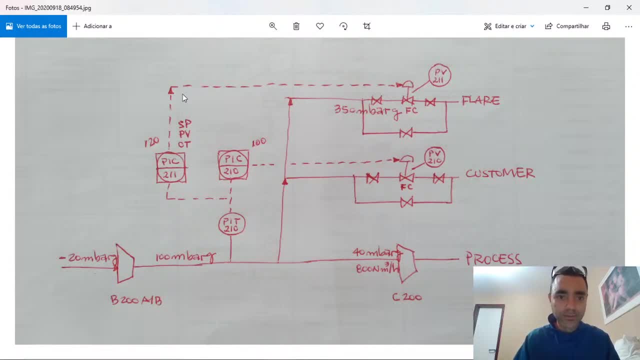 pressure valve and this pressure valve is named pressure valve because is named pressure valve, because is named pressure valve? because it is associated with a pic. it is associated with a pic. it is associated with a pic and the pic in this case is pressure and the pic in this case is pressure. 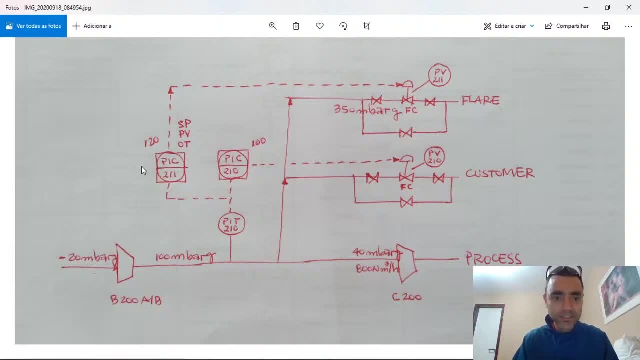 and the pic in this case is pressure indication control, indication control, indication control. it is my controller, so to have a, it is my controller, so to have a, it is my controller, so to have a control loop, i need to have a source of control loop. i need to have a source of. 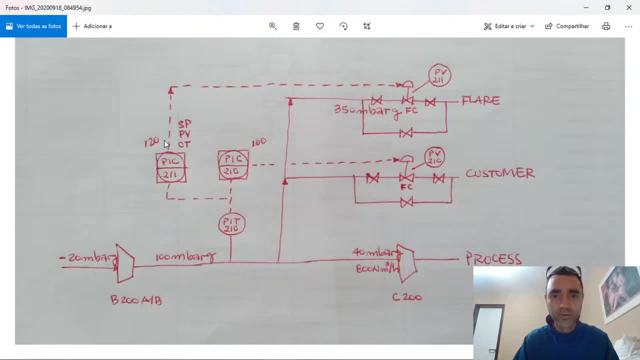 control loop. i need to have a source of measurement, measurement, measurement. i need to have a control, i need to have a control, i need to have a control, control and i need to have a control, and i need to have a control and i need to have a, a final device that will take. take the. 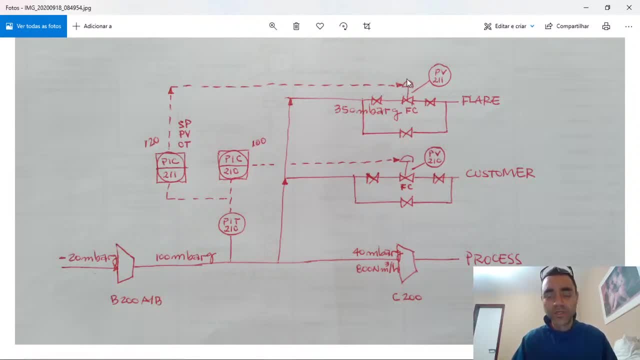 a final device that will take, take the, a final device that will take. take the action to action to action to to change or to control the the process to change or to control the the process to change or to control the the process. so if i didn't have the automatic 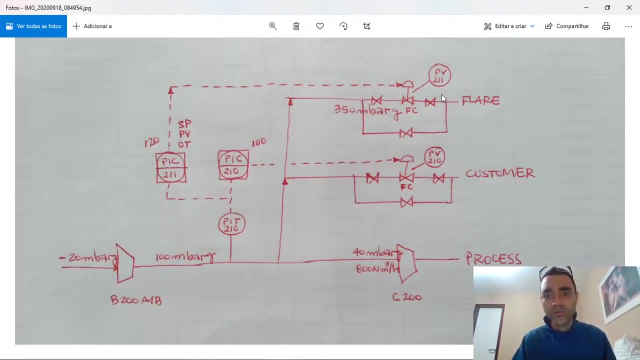 so if i didn't have the automatic? so if i didn't have the automatic control, or if i didn't have the control control, or if i didn't have the control control, or if i didn't have the control, what i could do is open or close. 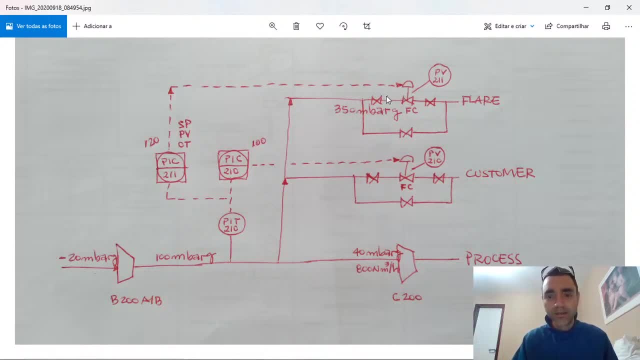 what i could do is open or close. what i could do is open or close dpv manually or in the other hand in the dpv manually or in the other hand in the dpv manually or in the other hand, in the other case i could. other case i could. 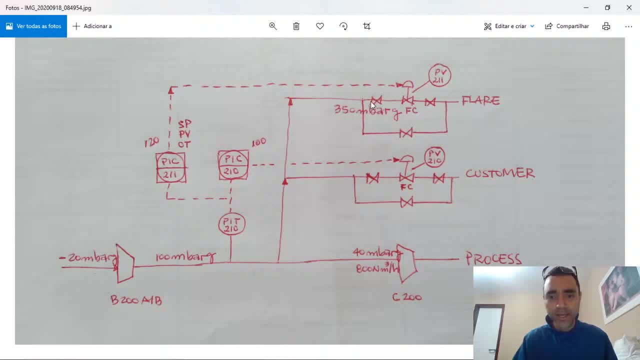 other case, i could block, block, block, isolate dpv, isolate dpv, isolate dpv at the downstream and out and at the at the downstream and out and at the at the downstream and out and at the upstream and at the downstream, upstream and at the downstream, downstream and out and at the downstream. and i could have, and i did this. 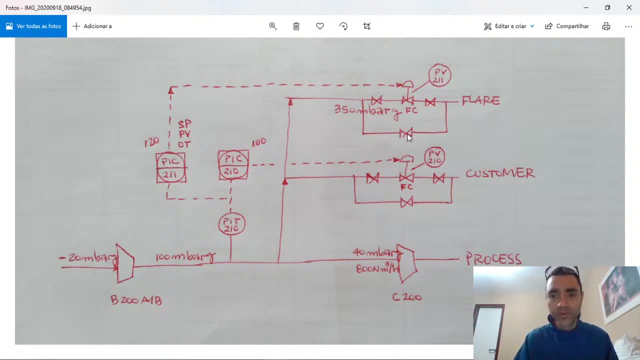 and i could have and i did this, and i could have and i did this sometimes today, during in the field. i sometimes today, during in the field, i sometimes today, during in the field, i could open the bypass of the control, could open the bypass of the control. 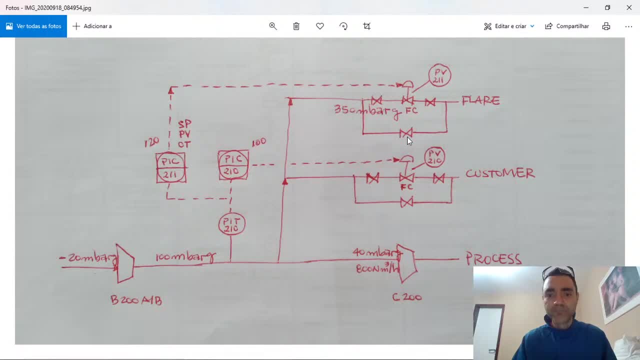 could open the bypass of the control valve more or less, more or less valve more or less, more or less valve more or less, more or less. and this is in this manual manual and this is in this manual manual and this is in this manual manual actions. i would be doing the 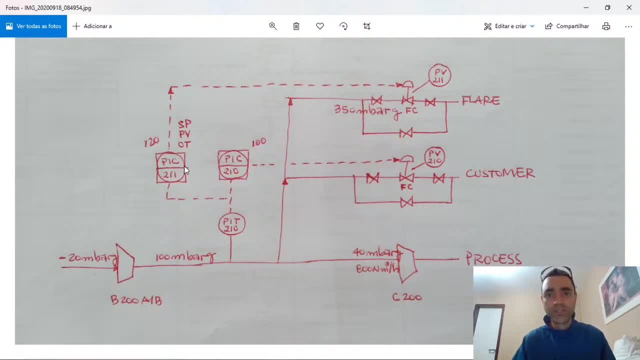 actions. i would be doing the actions. i would be doing the: the work of the controller, the work of the controller, the work of the controller, because what the controller do, in fact, because what the controller do in fact, because what the controller do in fact is automate. automate an action that could. 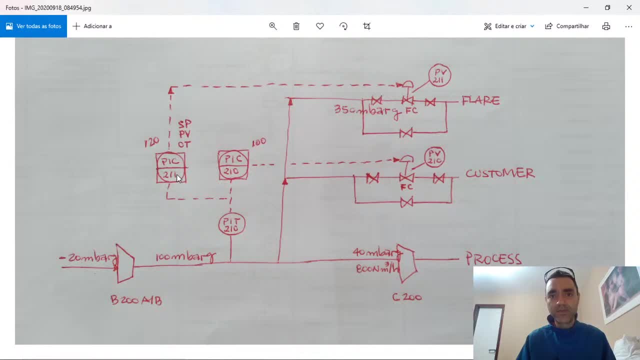 is automate. automate an action that could is automate. automate an action that could be done manually. so, instead of having be done manually so, instead of having be done manually so, instead of having someone to regulate the pressure at the someone, to regulate the pressure at the someone, to regulate the pressure at the discharge of the blower manually, we have 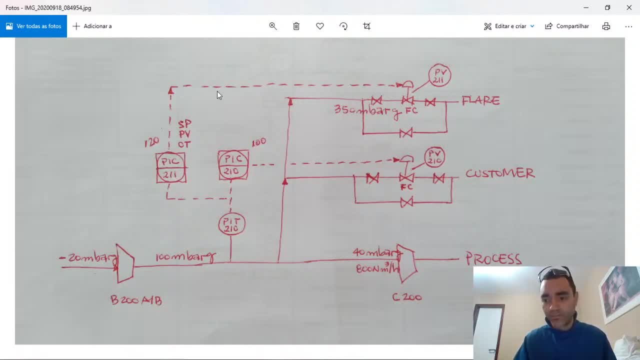 discharge of the blower manually. we have discharge of the blower manually. we have the control that will do this text, for the control that will do this text, for the control that will do this text for us, us, us, ah, we have sergio manuel maita paucara. 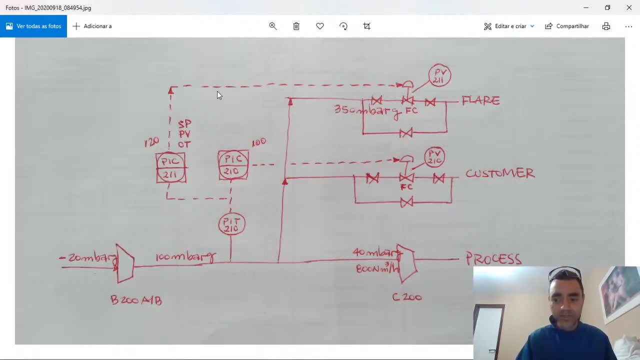 ah, we have sergio manuel maita paucara. ah, we have sergio manuel maita paucara. i believe that it is brazil because of. i believe that it is brazil because of. i believe that it is brazil because of the sergio. 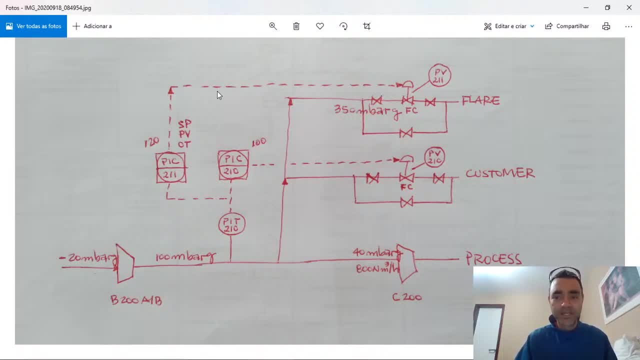 the sergio, the sergio, samuel mayata. it's. it seems to be a samuel mayata. it's. it seems to be a samuel mayata. it's. it seems to be a brazilian name. and thank you, emmanuel. brazilian name and thank you, emmanuel. 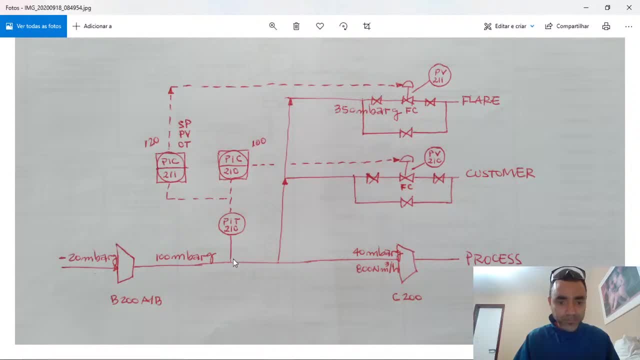 brazilian name and thank you, emmanuel, thank you, sergeant, for being here. and so thank you, sergeant, for being here. and so, thank you, sergeant, for being here. and so, uh, i will share with you the some kinds. uh, i will share with you the some kinds. uh, i will share with you the some kinds of pressure pressure measurement. 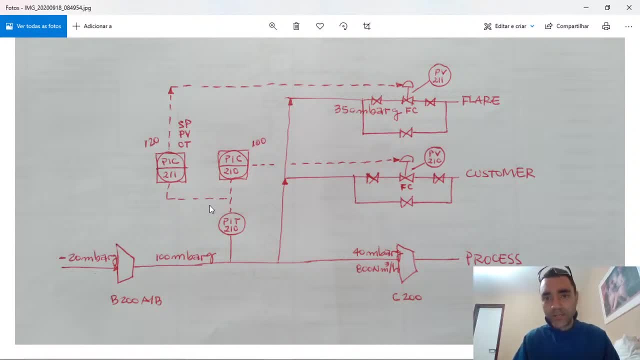 of pressure pressure measurement, of pressure pressure measurement, and and and now that i have a new customer, i need- now that i have a new customer, i need, now that i have a new customer, i need to guarantee, to guarantee, to guarantee the, the, the, the minimal pressure for my. 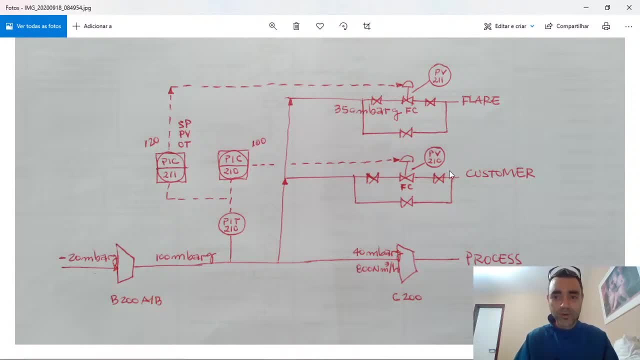 the minimal pressure for my, the minimal pressure for my. my compressor because my compressor, because my compressor, because, before having the customer, my only before having the customer, my only before having the customer, my only issue was when i stopped the compressor. issue was when i stopped the compressor. 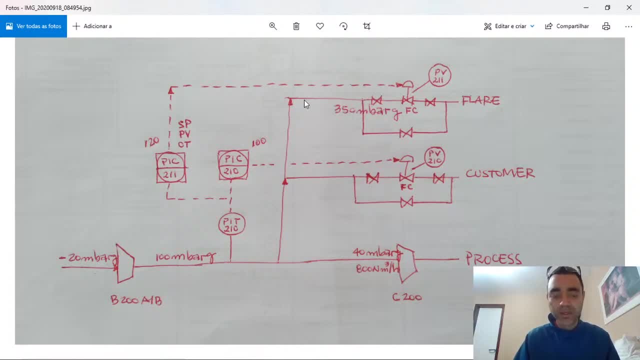 issue was when i stopped the compressor. i should release the. i should release the. i should release the, the, the, the. i should release the biogas to the flare. i should release the biogas to the flare. i should release the biogas to the flare and that. 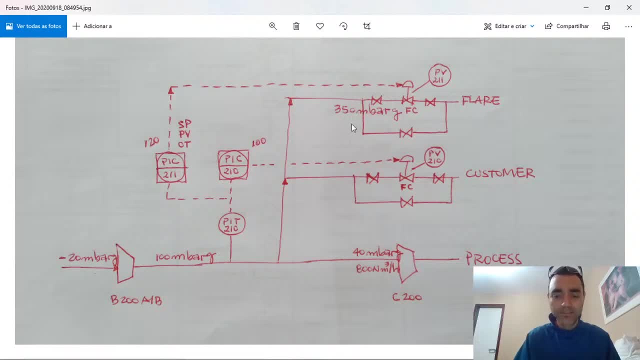 and that and that. how i could do that automatically. how i could do that automatically. how i could do that automatically when the, when the, when the. i have minus millibar g at the suction of. i have minus millibar g at the suction of. i have minus millibar g at the suction of the blower. 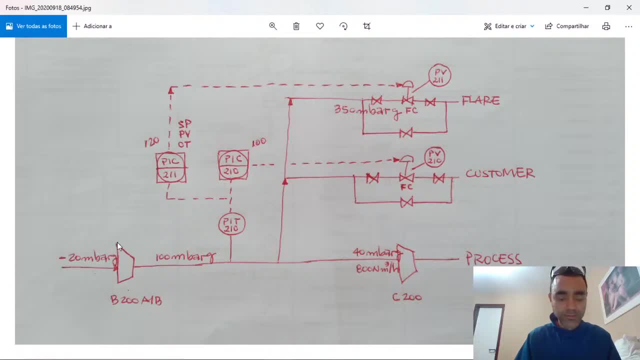 the blower. the blower it is, it is. it is designed to, designed to, designed to, to. designed to to deliver the the the bio the biogas, to deliver the the the biogas. to deliver the the the biogas at 100 millibar g. at 100 millibar g. at 100 millibar g and because of the pressure drop in the and because of the pressure drop in the and because of the pressure drop in the pipeline, it will reach the compressor pipeline. it will reach the compressor pipeline. it will reach the compressor around 50 millibar g at 800 normal. 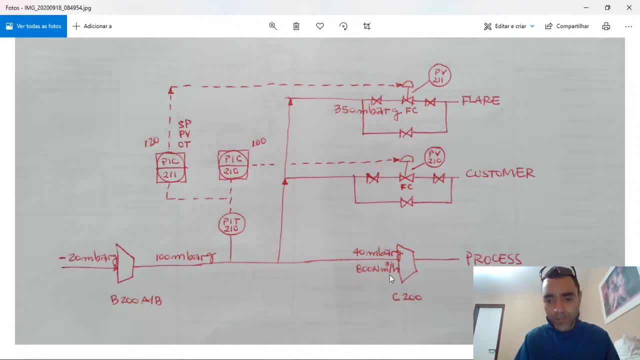 around 50 millibar g at 800 normal. around 50 millibar g at 800 normal cubic meter per hour. cubic meter per hour. cubic meter per hour. but when i stop the compressor, but when i stop the compressor, but when i stop the compressor i will not taking the, the gas. so the 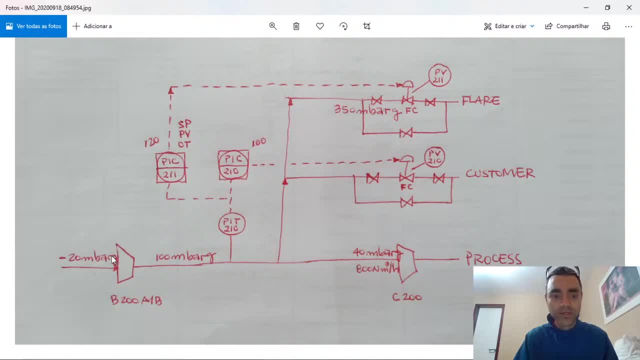 i will not taking the the gas, so the. i will not taking the the gas. so the gas that is in the suction of the blower gas, that is in the suction of the blower gas, that is in the suction of the blower will be compressed, but as it doesn't, 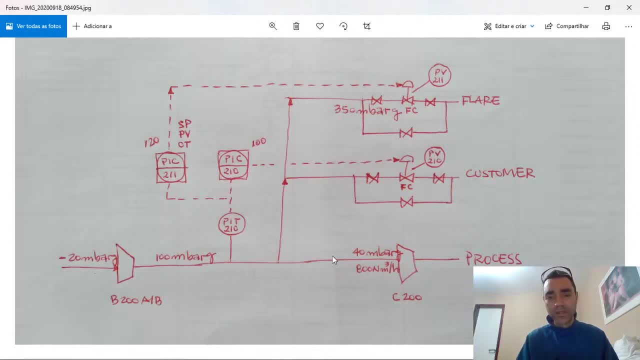 will be compressed, but as it doesn't, will be compressed, but as it doesn't, doesn't have to, doesn't have to, doesn't have to. where to go? it will where to go, it will where to go. it will build pressure at the system and the build pressure at the system and the. build pressure at the system and the pressure will increase it to prevent any pressure will increase it to prevent any pressure will increase it to prevent any kind of damage in the pipeline and or kind of damage in the pipeline and or kind of damage in the pipeline and or in the suction of the compressor. i. 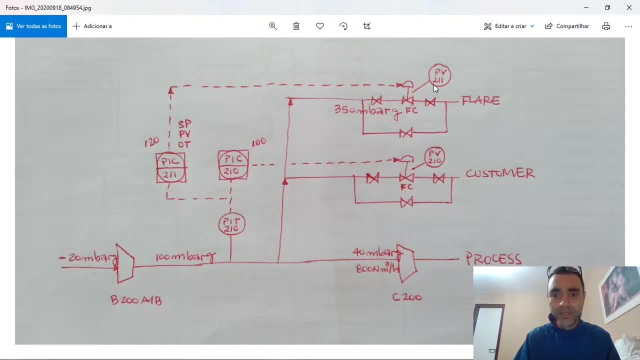 in the suction of the compressor, i, in the suction of the compressor, i release this pressure, release this pressure, release this pressure, opening the pv. and to do that, i need to opening the pv, and to do that, i need to opening the pv, and to do that, i need to set. 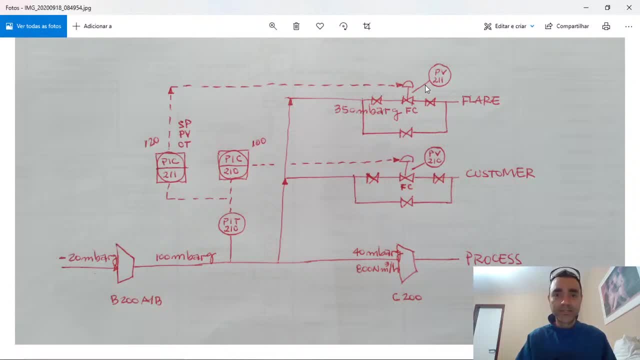 set set. i need to define a set point that best. i need to define a set point that best. i need to define a set point that best fits to my process in the end in this fits to my process in the end in this fits to my process in the end in this case. 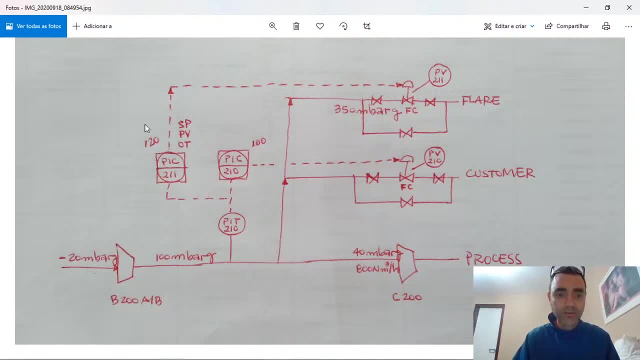 case case. i set the set point as 120 millibar g. i set the set point as 120 millibar g. i set the set point as 120 millibar g. so it means that i run in my process. so it means that i run in my process. 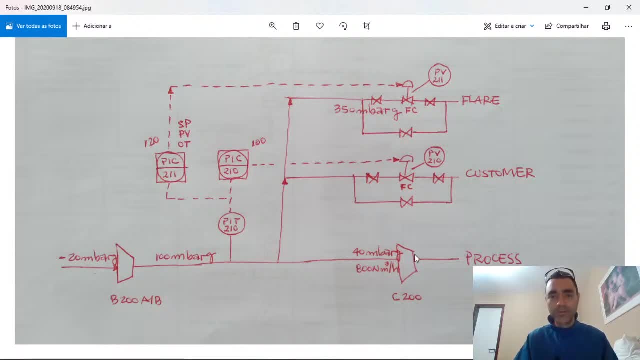 so it means that i run in my process with 100 millibar g, with 100 millibar g, with 100 millibar g, and my compressor is running also, and, and my compressor is running also, and, and my compressor is running also and because of the pressure drop at the. because of the pressure drop at the, because of the pressure drop at the pipeline, pipeline, pipeline. in the suction of the compressor i have in the suction of the compressor i have in the suction of the compressor i have 40 to 50 millibar g, 40 to 50 millibar g. 40 to 50 millibar g, but once the compressor is stopped. but once the compressor is stopped. but once the compressor is stopped, the the pressure will build up and when the the pressure will build up. and when the the pressure will build up and when it reaches 120. 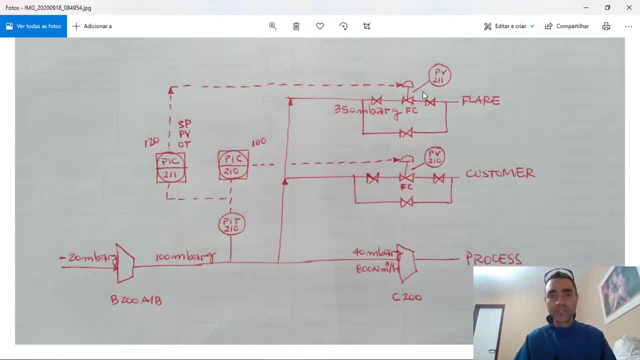 it reaches 120. it reaches 120 millibar g, my millibar g, my millibar g, my pv will start opening and one and once it pv will start opening and one and once it pv will start opening and one and once it starting opening. 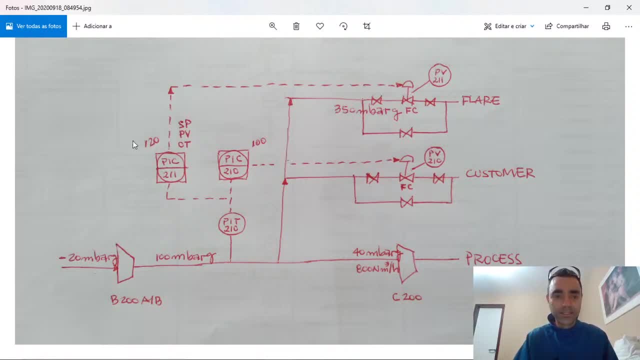 starting opening, starting opening. the pressure will be controlled in this. the pressure will be controlled in this. the pressure will be controlled in this, in this set point, in this set point, in this set point, if i have too much flow, if i have too much flow, if i have too much flow, my pressure will open more. if i have 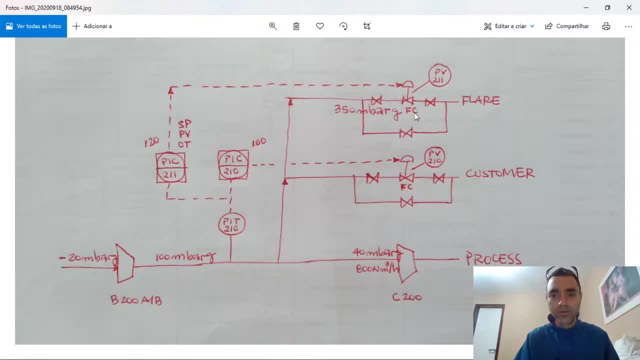 my pressure will open more. if i have, my pressure will open more. if i have a small flow- my, a small flow, my, a small flow- my pressure valve will open less pressure valve will open less. pressure valve will open less, and this and this and this, it is important to you understand what. 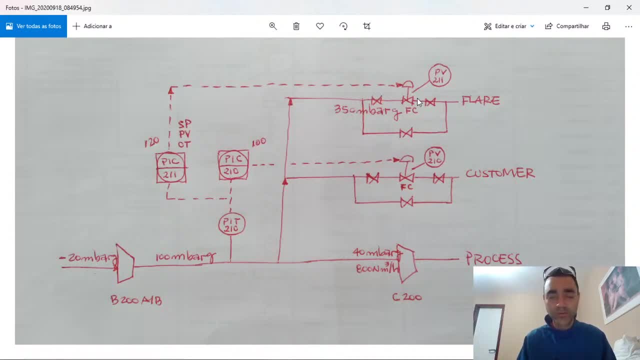 it is important to you understand what. it is important to you understand what is the kind of action that we have in is the kind of action that we have in, is the kind of action that we have in the control valve, the control valve, the control valve, because 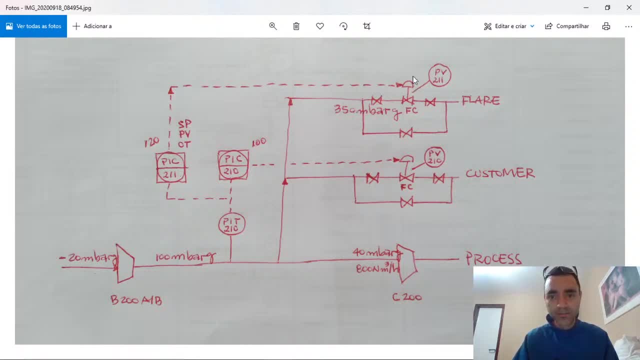 because because the the controller will send a signal, the the controller will send a signal, the the controller will send a signal to the control valve and to the control valve and to the control valve. and i need to know if, if i, if. i need to know if, if i, if. 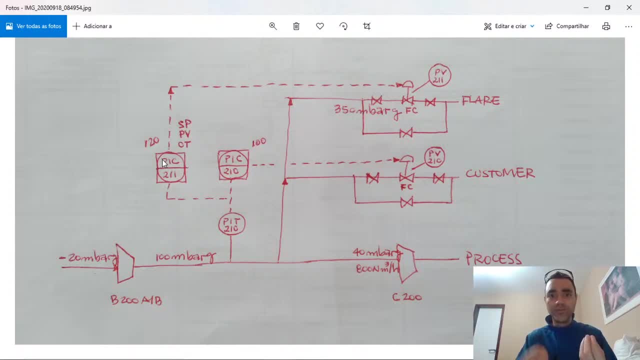 i need to know if, if i, if, if i increase the signal, my valve should. if i increase the signal, my valve should. if i increase the signal, my valve should increase the opening also. or it should increase the opening also, or it should increase the opening also, or it should decrease the opening, and there is two. 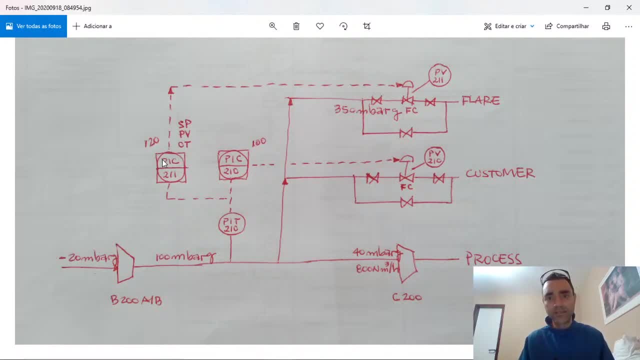 decrease the opening. and there is two- decrease the opening. and there is two kinds of kinds of kinds of control actions and the the first one control actions, and the the first one control actions. and the the first one is the direct action. it means that if i is the direct action, it means that if i 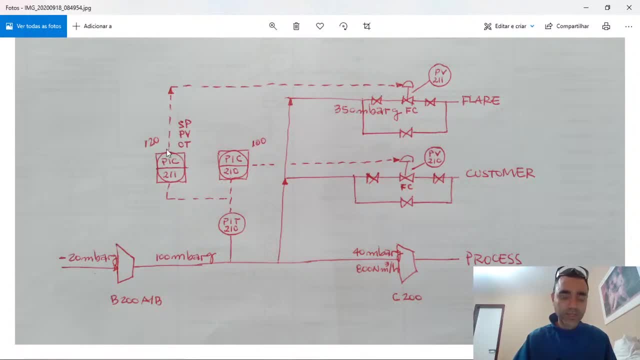 is the direct action. it means that if i increase the signal that comes out from, increase the signal that comes out from, increase the signal that comes out from the pic, the pic, the pic to the actuator of the valve, it should. to the actuator of the valve: it should. 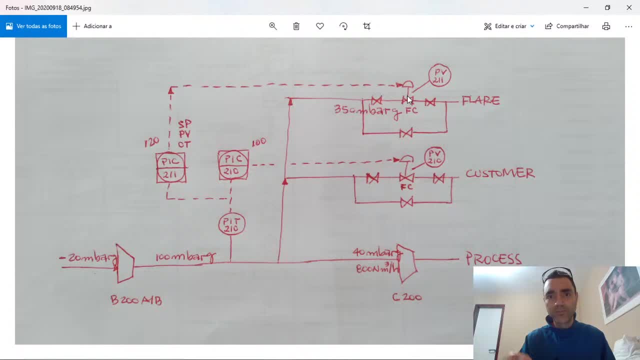 to the actuator of the valve, it should also increases it opening, and i'm also increases it opening and i'm also increases it opening and i'm talking, i will talk more about that, talking, i will talk more about that, talking, i will talk more about that. and in the opposite side, i have the 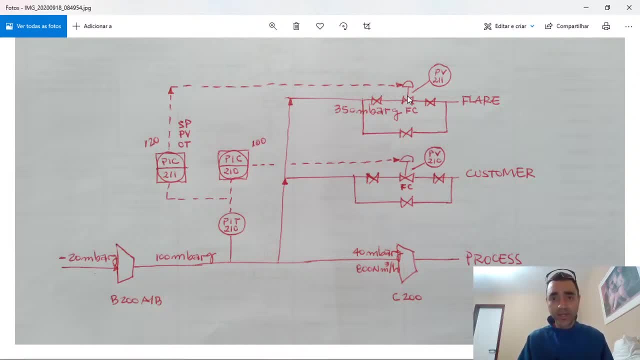 and in the opposite side i have the, and in the opposite side i have the reverse action, and in the reverse action, reverse action, and in the reverse action, reverse action and in the reverse action. when i increase the signal of the, when i increase the signal of the, 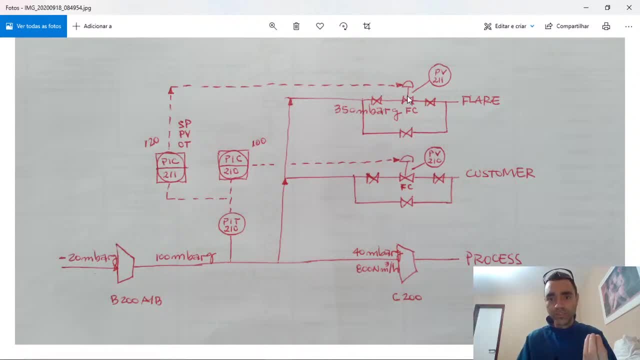 when i increase the signal of the controller, my valve should close controller. my valve should close controller. my valve should close and it this kind of of, and it this kind of of, and it this kind of of this kind of this kind of of this kind of of hassle scene or this kind of working. 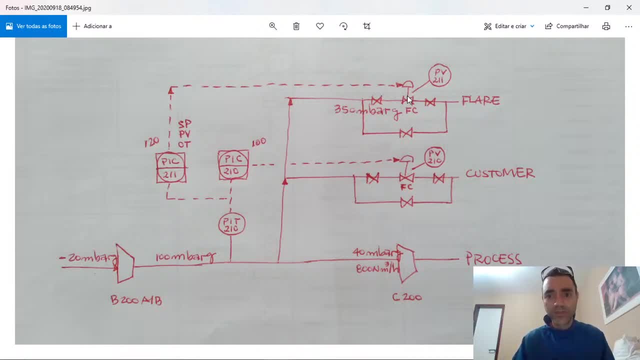 hassle scene or this kind of working hassle scene or this kind of working. uh, it is possible to associate that. uh, it is possible to associate that. uh, it is possible to associate that because we are, because we are, because we are talking about a fail close valve, talking about a fail close valve. 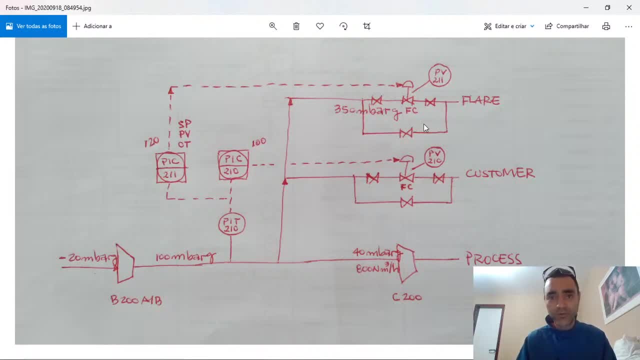 talking about a fail close valve, and this is uh another kind of, and this is uh another kind of and this is uh another kind of information that you should know about, information that you should know about, information that you should know about the about control valves, the about control valves. 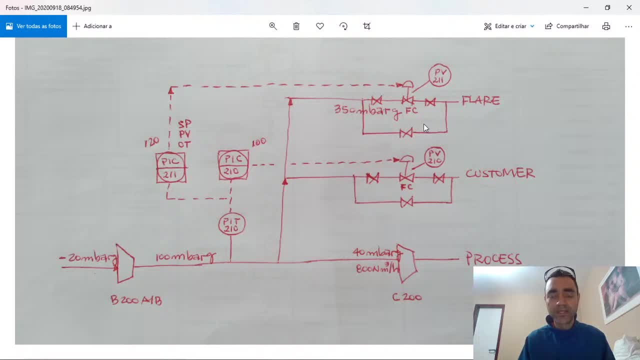 the about control valves is the. what is the safe position in a? is the. what is the safe position in a? is the. what is the safe position in a case, if i case, if i case, if i cut off this, the power supply of in the cut off this, the power supply of in the? 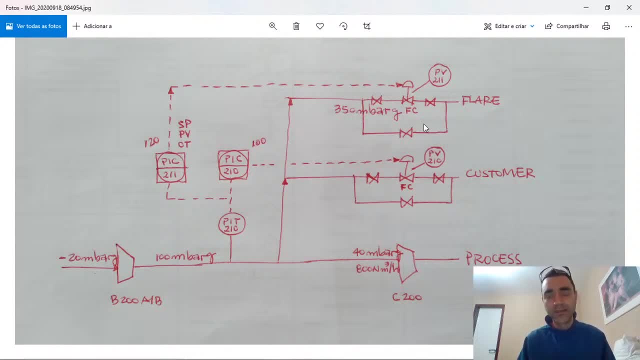 cut off this, the power supply of in the valve, and the power supply could be valve, and the power supply could be valve and the power supply could be instrument air could be electricity. could instrument air could be electricity. could instrument air could be electricity. could be, be be something hydraulic or something like. 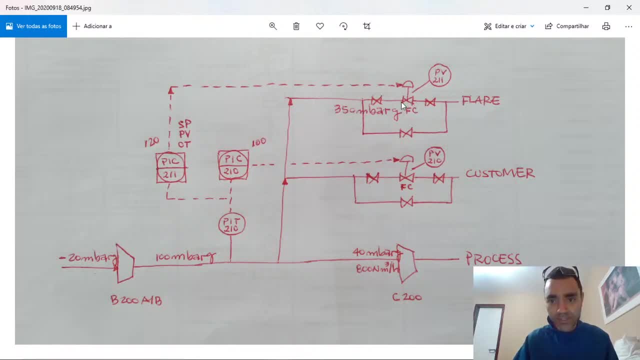 something hydraulic or something like something hydraulic or something like that. so that, so that. so when i my fc here below the control, when i my fc here below the control, when i my fc here below the control valve means that if i lose the valve, means that if i lose the 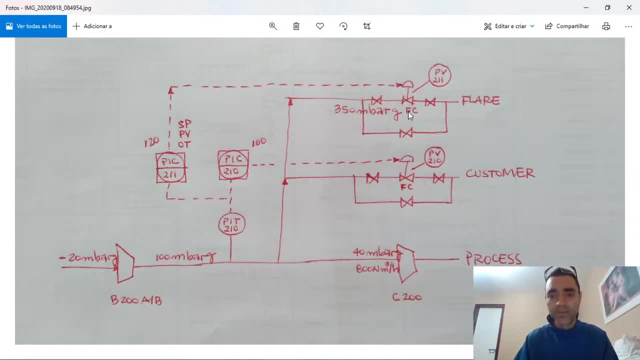 valve means that if i lose the the power to to actuate the valve, my the power to to actuate the valve, my the power to to actuate the valve, my valve will, valve will, valve will, will go to the closed position. will go to the closed position. 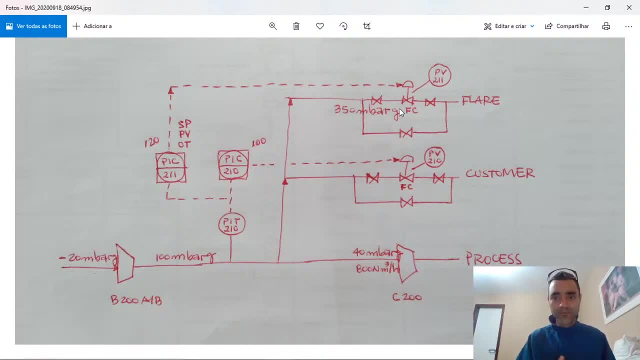 will go to the closed position. so it means that. so it means that. so it means that, uh, if it is a valve that has a signal of uh, if it is a valve that has a signal of uh, if it is a valve that has a signal of 4 to 20 milli milliampere. 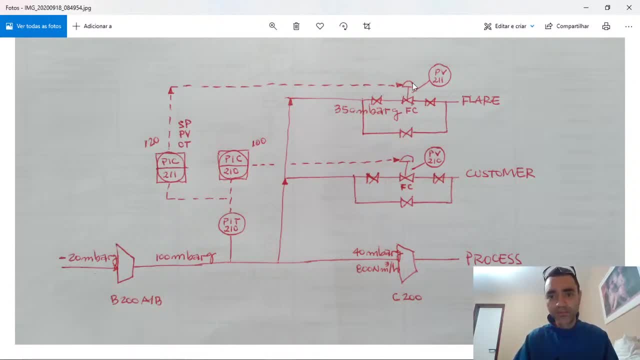 4 to 20 milli milli ampere. 4 to 20 milli milli ampere. if i send a signal of 4 milliampere to, if i send a signal of 4 milliampere to, if i send a signal of 4 milliampere to this valve, it means that it should be. 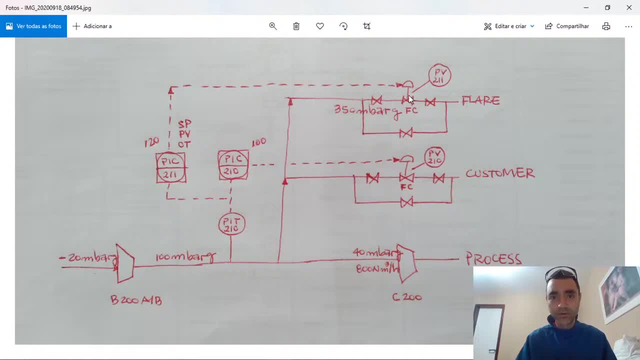 this valve. it means that it should be this valve. it means that it should be: uh zero. it should be closed, zero opening, uh zero. it should be closed, zero opening, uh zero. it should be closed, zero opening. in the other hand, if my controller, in the other hand, if my controller. 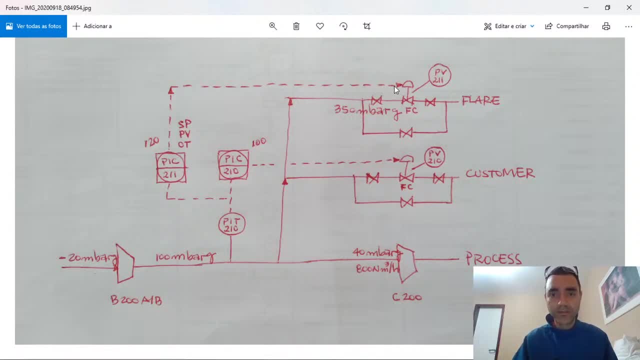 in the other hand, if my controller sends a signal of 20 milli bar g milli, sends a signal of 20 milli bar g milli, sends a signal of 20 milli bar g milli milliampere to the controller of the. 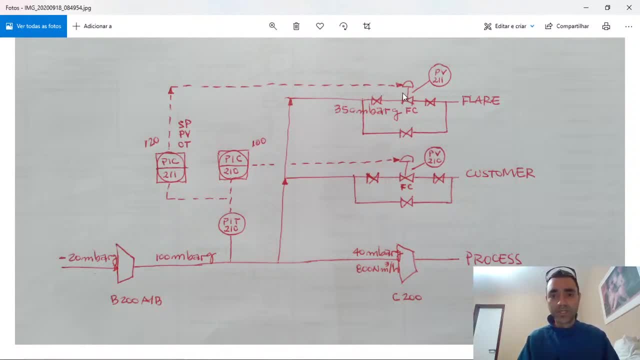 milliampere to the controller of the milliampere, to the controller of the valve. it should be 100 valve. it should be 100 valve. it should be 100 percent opening. and this is the way, percent opening, and this is the way, percent opening, and this is the way that it is. if it, 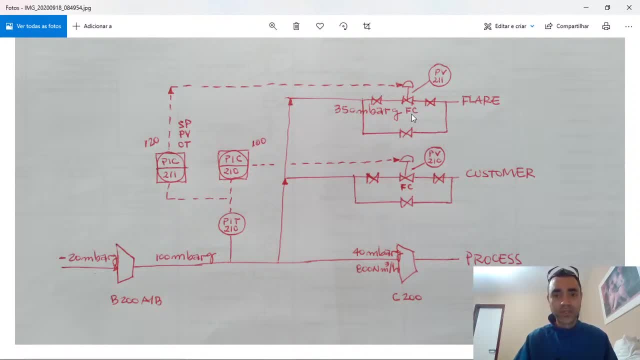 that it is. if it that it is. if it was a fail opening valve was a fail opening valve was a fail opening valve. it should be the the opposite. my, it should be the the opposite. my, it should be the the opposite. my four, four, four millibar milliampere would be 100. 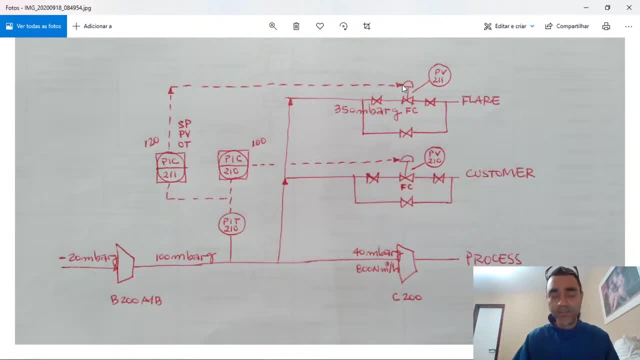 millibar milliampere would be 100 millibar milliampere would be 100, opening and my 20 milliampere should be opening and my 20 milliampere should be opening and my 20 milliampere should be zero. but 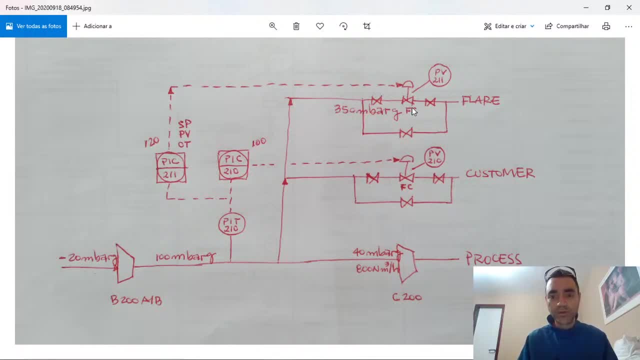 zero, but zero, but and but everton knows, and the automation, and, but everton knows, and the automation, and, but everton knows, and the automation knows that is possible, although knows that is possible, although knows that is possible, although the, the, the, the, the action of the valve is the opposite. 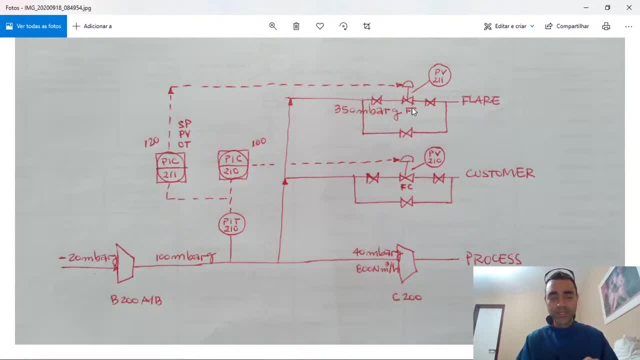 the action of the valve is the opposite. the action of the valve is the opposite because it is a fail opening, because it is a fail opening, because it is a fail opening and there is a mathematical uh equation, and there is a mathematical uh equation, and there is a mathematical uh equation that we can do. 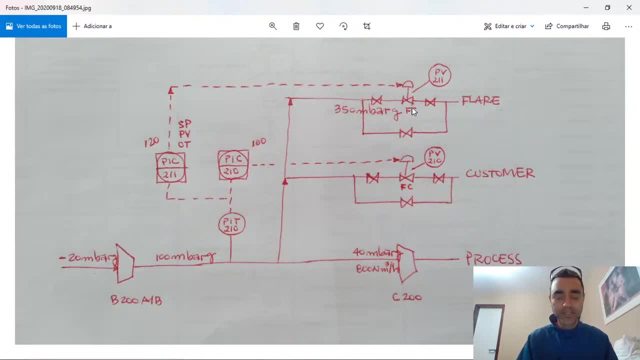 that we can do that. we can do that the valve actuate at the same way that the valve actuate at the same way that the valve actuate at the same way, for instance. we could add, for instance, we could add, for instance, we could add one: 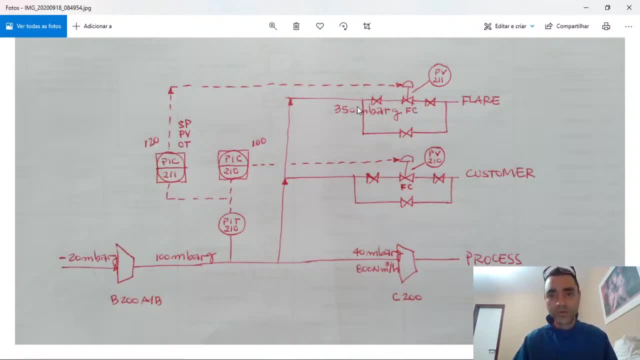 one one. minus the the signal of the controller. minus the- the signal of the controller. minus the- the signal of the controller and a control valve fail. open control and a control valve fail. open control and a control valve fail. open control valve: valve valve would be actuated like a fail close. 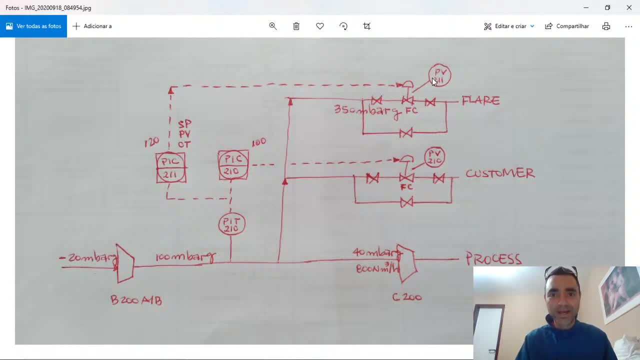 would be actuated like a fail close would be actuated like a fail close. let's, let's, let's. it seems to be uh i, so it seems to be uh i, so it seems to be uh i. so, okay, okay, okay, let's do an example, and sorry, i don't. 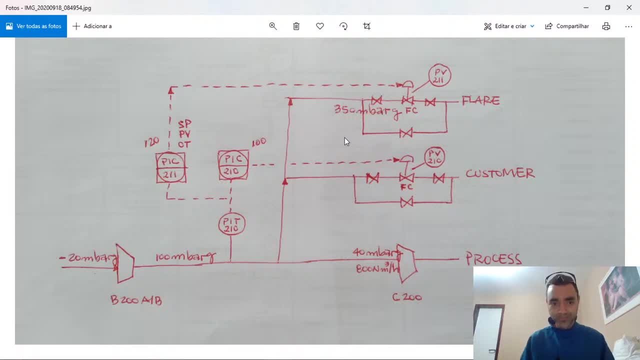 let's do an example, and sorry i don't. let's do an example and sorry i don't have uh have uh have uh anything to to write to you, anything to to write to you, anything to to write to you, but but but if the controller sends a signal of 20. 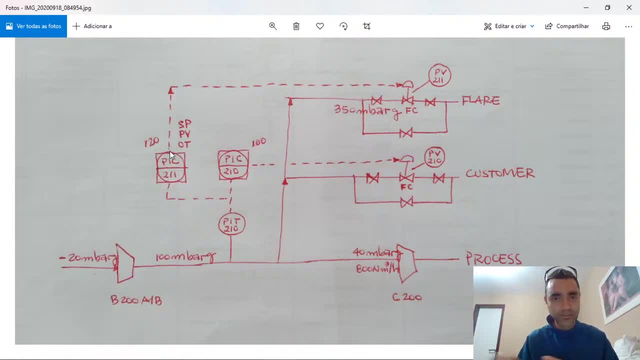 if the controller sends a signal of 20. if the controller sends a signal of 20, let's think about percentage and not. let's think about percentage and not. let's think about percentage and not milli, milliampere, milli, milliampere. 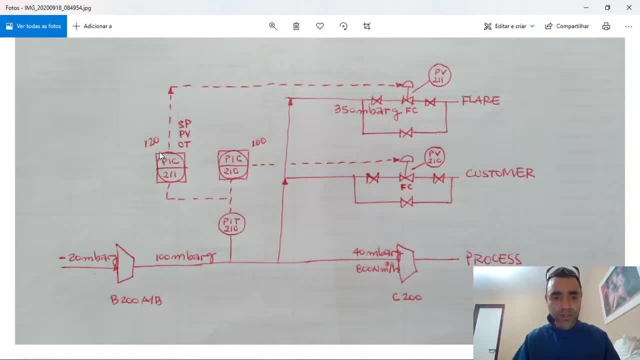 milli milliampere. if the, if the, if the in a fail close valve. if i say the in a fail close valve. if i say the in a fail close valve. if i say the controller sends 20 to the, the controller sends 20 to the, the. 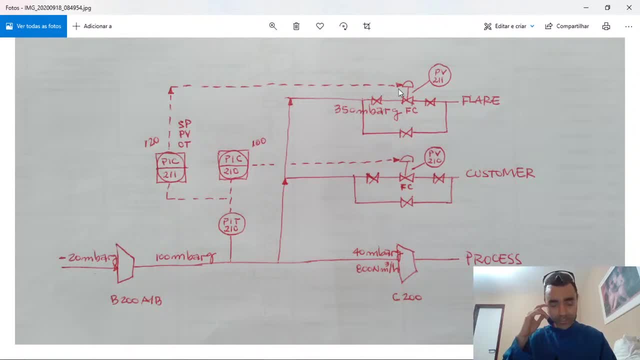 controller sends 20 to the the fail close valve, it will open 20. fail close valve: it will open 20. fail close valve: it will open 20. if it sends 50, it will open 50. if it sends 50, it will open 50. 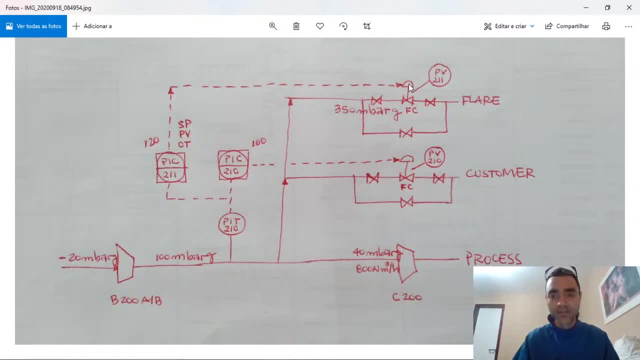 if it sends 50, it will open 50 and if and if and if it sends 100, it sends 100, it sends 100, the valve will be full open- 100 open. the valve will be full open- 100 open. the valve will be full open, 100 open. but if we are talking about 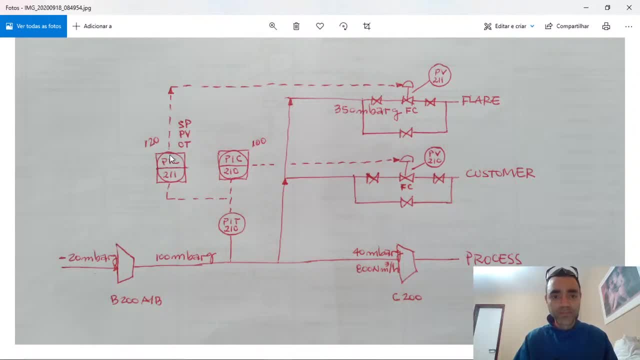 but if we are talking about, but if we are talking about: fail open valve, fail open valve, fail open valve: uh 20, 20 of the signal, uh 20, 20 of the signal, uh 20, 20 of the signal means that the valve, means that the valve. 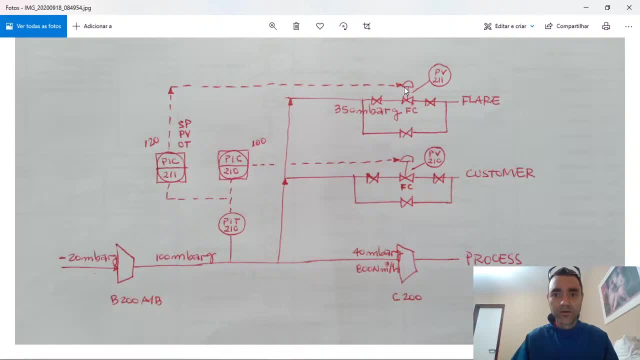 means that the valve is 20, is 20, is 20 closed or closed, or closed or 80 percent open. why because when i have 80 percent open? why because when i have 80 percent open? why because when i have 100 percent, 100 percent. 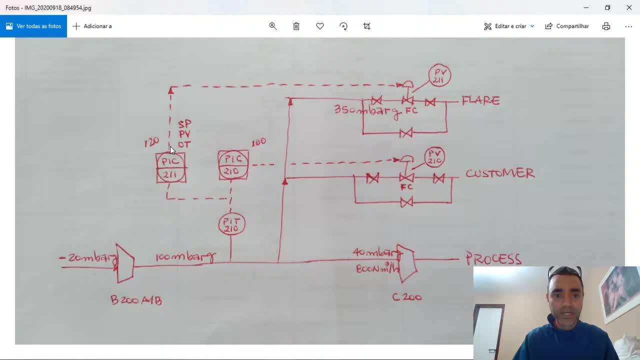 100 percent. it is, it is. it is zero opening. and when i have zero from the zero opening, and when i have zero from the zero opening, and when i have zero from the controller, it is controller, it is controller, it is 100 percent, 100 percent. 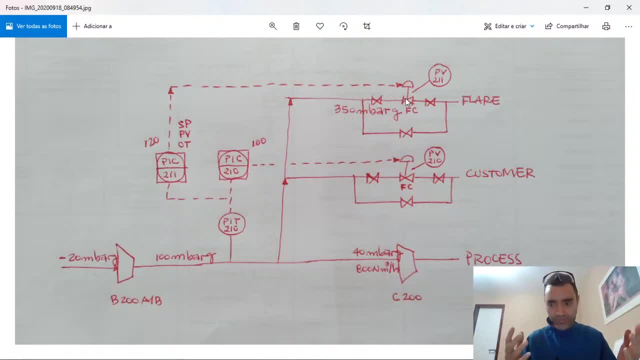 100 percent. so to prevent this kind of of so, to prevent this kind of of so, to prevent this kind of of information, it's information, it's information, it's due to, due to, due to, to prevent the operator or to prevent the. to prevent the operator or to prevent the. 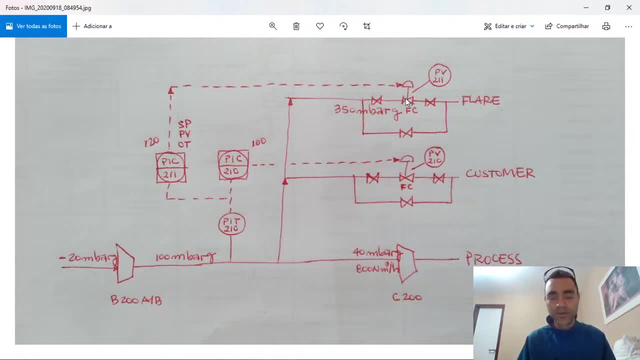 to prevent the operator or to prevent the process engineer from process engineer, from process engineer, from thinking that, oh, it is a fail. close thinking that, oh, it is a fail. close thinking that, oh, it is a fail, close fail. open valve: i need to to fail. open valve: i need to to. 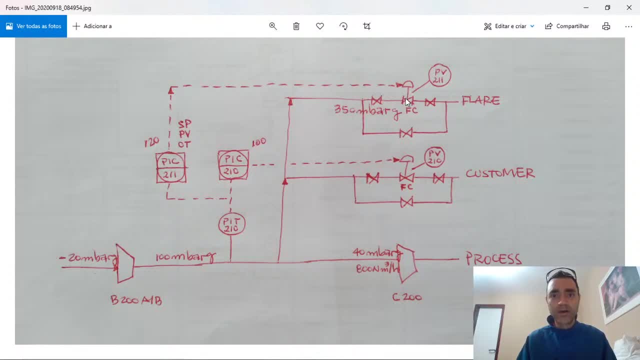 fail open valve. i need to to to think at the opposite. what the think at the opposite, what the think at the opposite, what the automation guys, automation guys, automation guys can do to solve, that is can do to solve, that is can do to solve. that is 100. 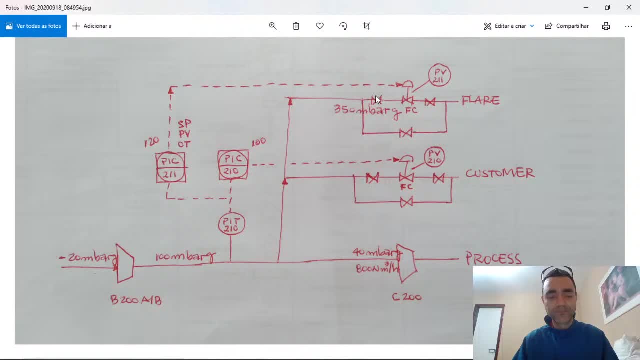 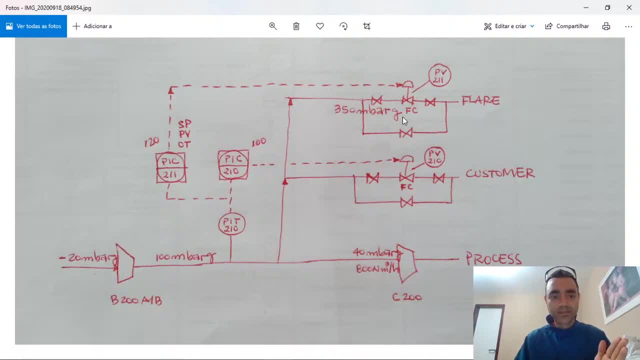 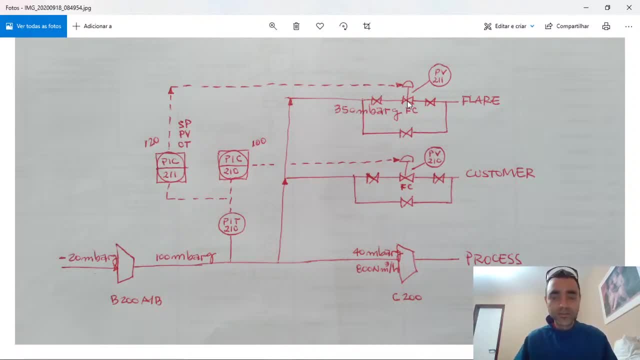 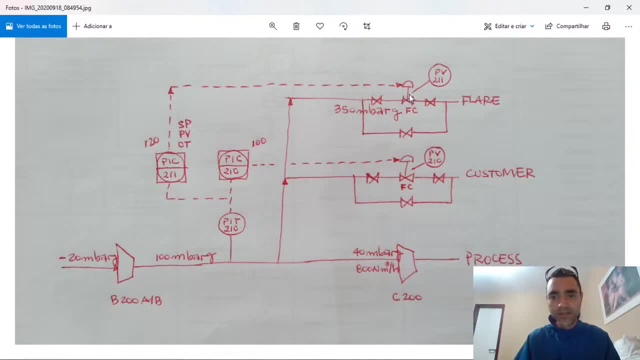 when i have, when i have uh, uh, uh, when i see, when i see, when i see the devolve, the devolve, the devolve, 20 percent opening, it doesn't matter for 20 percent opening. it doesn't matter for 20 percent opening. it doesn't matter for me if it is a fail. close of a fail. 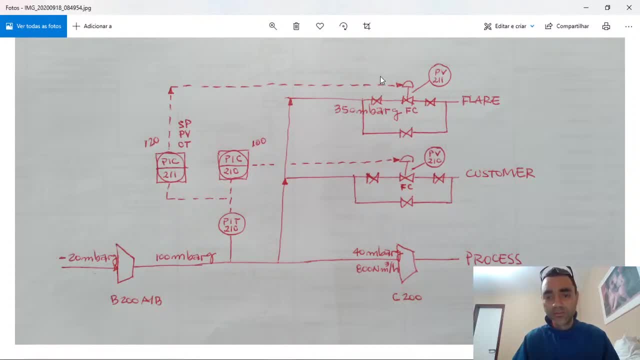 me if it is a fail, close of a, fail me. if it is a fail, close of a fail opening. if i see 20 percent to the to opening, if i see 20 percent to the to opening, if i see 20 percent to the to devolve, i i know that it is 20 percent. 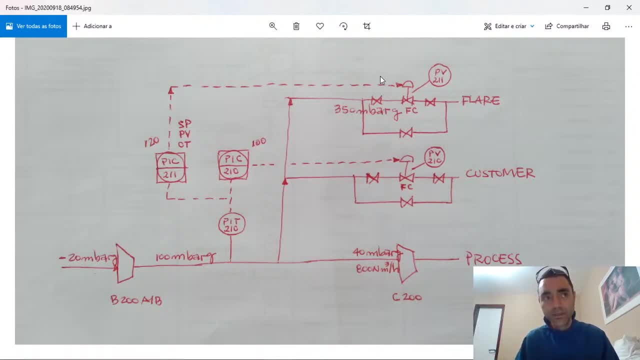 devolve i i know that it is 20 percent devolve i. i know that it is 20 percent opening and for us that are doing opening, and for us that are doing opening, and for us that are doing the verification of the system, the process, the verification of the system, the process. 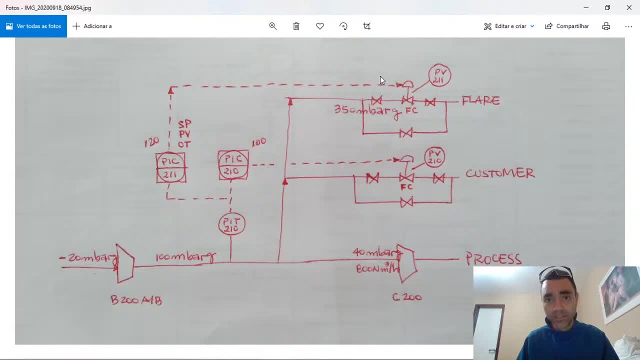 the verification of the system, the process engineer, the operators, what? what engineer the operators? what? what engineer the operators? what? what matters for us? matters for us, matters for us, in fact, in summary, what matters for us, in fact, in summary, what matters for us, in fact, in summary, what matters for us, process engineers and operators, is no. 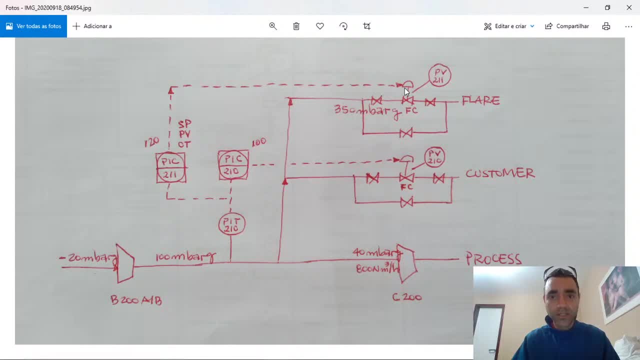 process engineers and operators is no. process engineers and operators is no. the opening of the valve and not, and not the opening of the valve and not, and not. the opening of the valve and not, and not. the signal that goes to the valve, the. the signal that goes to the valve, the. 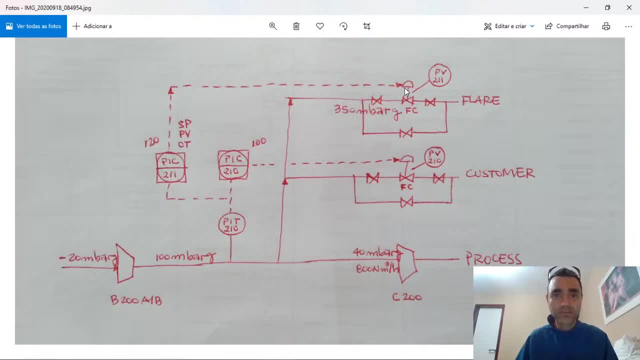 the signal that goes to the valve. the signal that goes to the valve is it is signal that goes to the valve, is it is signal that goes to the valve, is it is important to the instrumentation guy, important to the instrumentation guy, important to the instrumentation guy into the automation guide because they 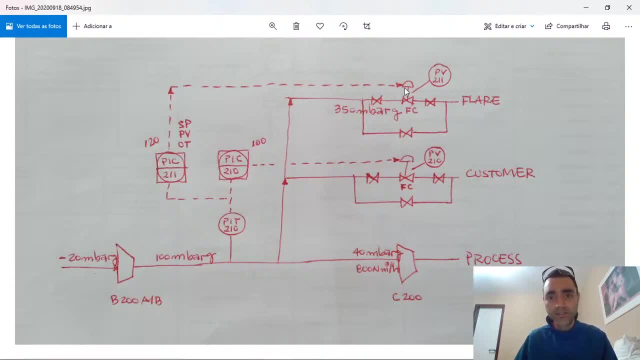 into the automation guide. because they into the automation guide? because they they can evaluate if the valve is. they can evaluate if the valve is. they can evaluate if the valve is the actuator and the controller is the actuator and the controller is the actuator and the controller is working properly. 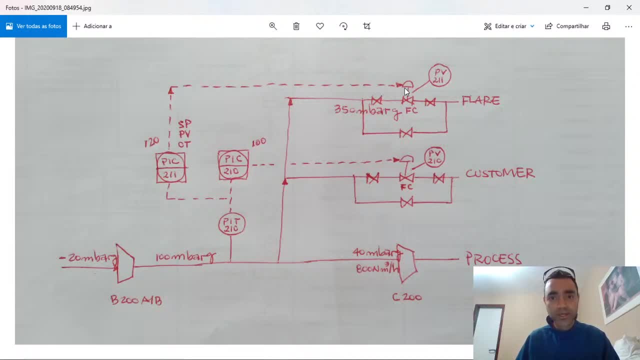 working properly, working properly. but once that is finished is commissioned. but once that is finished is commissioned. but once that is finished is commissioned, and, and, and read to, to run, read to, to run, read to, to run what, what, what, we? we don't care about that, we process. 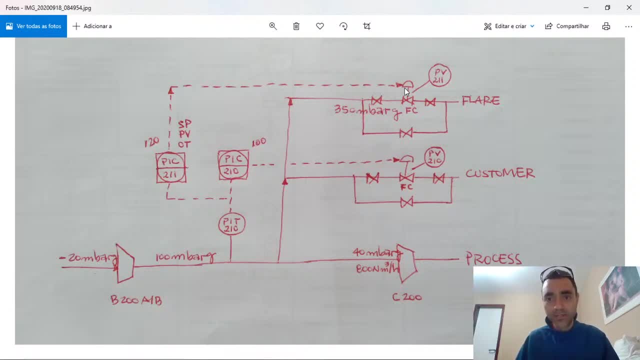 we, we don't care about that. we process. we, we don't care about that. we process engineer and engineer and engineer and and operators don't don't care about that and operators don't don't care about that and operators don't don't care about that. what we want to know is: the valve is. 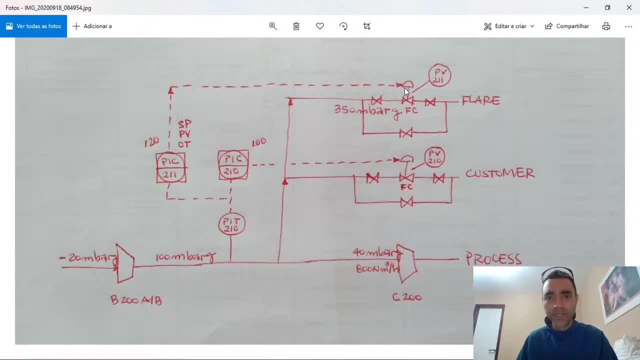 what we want to know is the valve is. what we want to know is: the valve is 20% opening, it's 40% opening, 60 and 20% opening, it's 40% opening, 60 and 20% opening, it's 40% opening 60 and something like that, because with this we 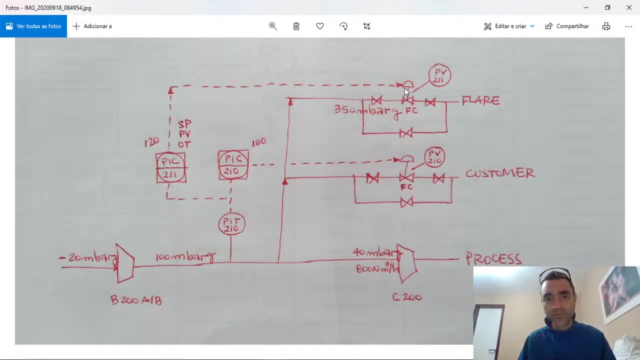 something like that, because with this we. something like that, because with this we can associate, can associate, can associate, uh some process values. what when the uh some process values? what when the uh some process values? what when the the valve is too much too much closing the valve is too much too much closing. 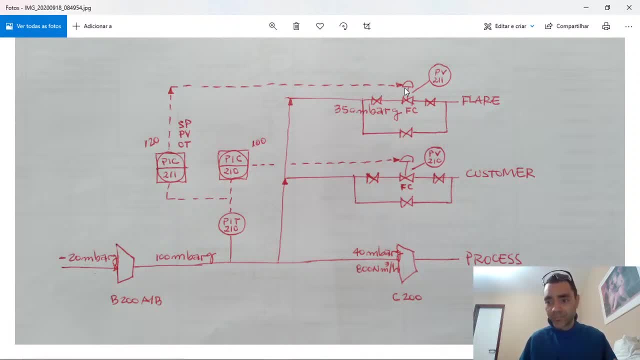 the valve is too much, too much closing, too much open, we can associate too much open, we can associate too much open. we can associate something like that: ah, thank you, everton, thank you. ah, thank you, everton, thank you. ah, thank you, everton, thank you. so everton is a automation guy and i 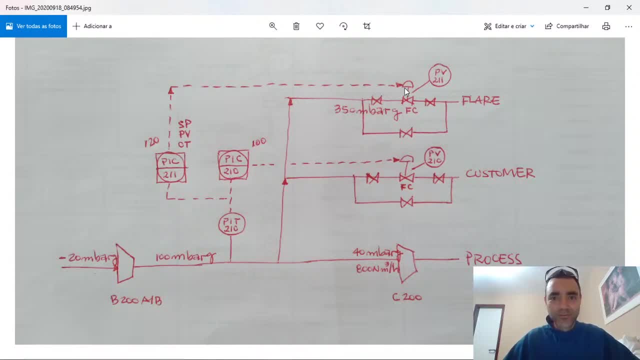 so everton is a automation guy and i so everton is a automation guy and i should take care to not, should take care to not, should take care to not say something wrong here because for say something wrong here, because for say something wrong here, because, for sure, my friend, please correct me and 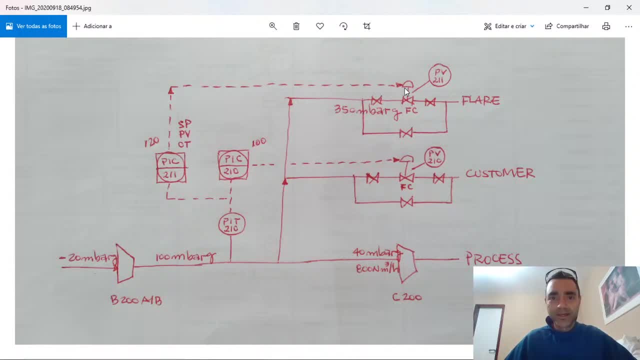 sure my friend please correct me, and sure my friend please correct me. and in the future i, i will invite, in the future i, i will invite, in the future i, i will invite everton to talk to me with in the live, everton to talk to me with in the live. 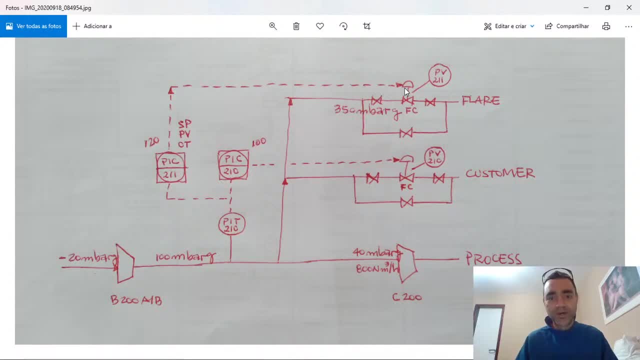 everton to talk to me with in the live sessions and there we will be able to sessions and there we will be able to sessions and there we will be able to talk more about this kind of subs and talk more about this kind of subs and talk more about this kind of subs, and will be very nice. so, everton, i'm using 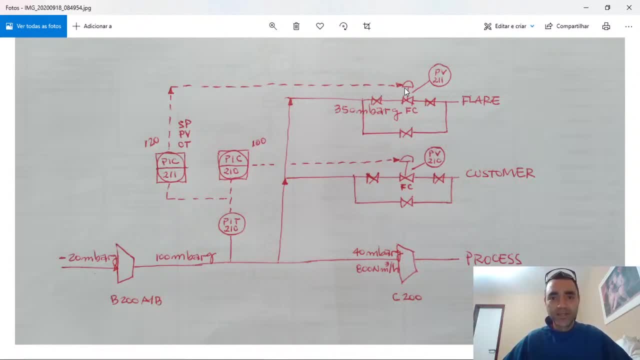 will be very nice. so, everton, i'm using will be very nice. so, everton, i'm using this live session to invite you to be a this live session, to invite you to be a this live session, to invite you to be a guest of my, in my, in process. 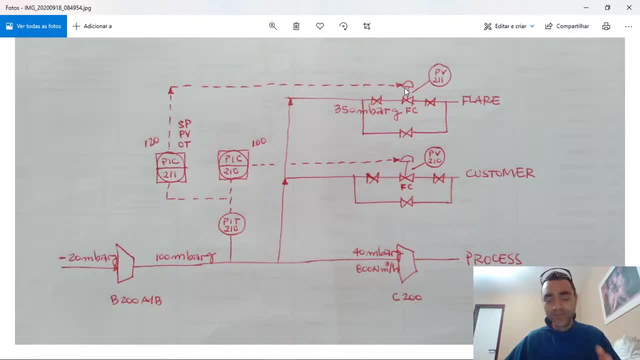 guest of my in my in process, guest of my in my in process interviews and i hope you accept my interviews and i hope you accept my interviews and i hope you accept my invitation. you don't need to answer invitation. you don't need to answer invitation. you don't need to answer right now, but consider that okay and i 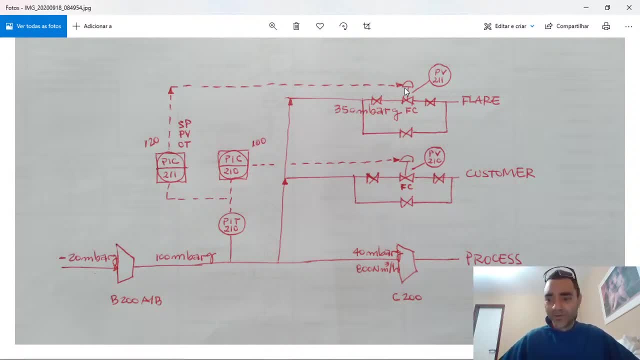 right now, but consider that okay. and i right now, but consider that okay. and i have a, have a, have a. uh, a relative here also, allison cardoso. uh, a relative here also, allison cardoso. uh, a relative here also. allison cardoso is a relative of mine, so, allison, please, 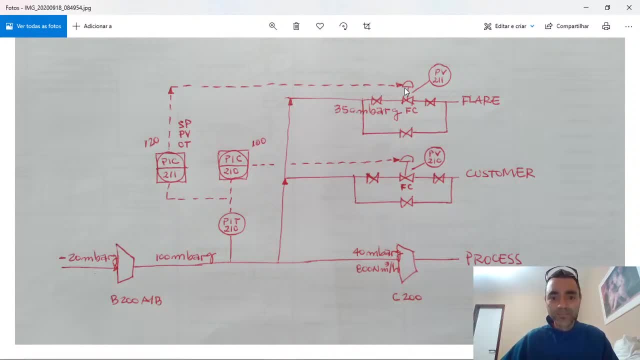 is a relative of mine, so, allison, please, is a relative of mine. so, allison, please, thank you for being with me right now. thank you for being with me right now. thank you for being with me right now. so, guys, what we have seen up to this, 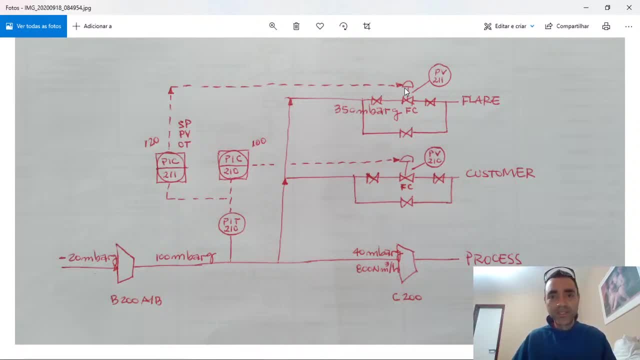 so, guys, what we have seen up to this, so, guys, what we have seen up to this point, point, point- is that the? the controller can be. is that the the controller can be? is that the the controller can be, uh, direct action or reverse action? uh, direct action or reverse action? 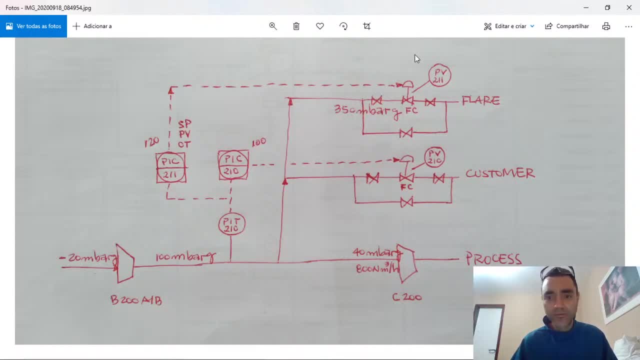 uh, direct action or reverse action, and we can. we have seen that the and we can. we have seen that the and we can. we have seen that the control valve fail position. control valve fail position. control valve fail position can be feel close, feel open, but there are. 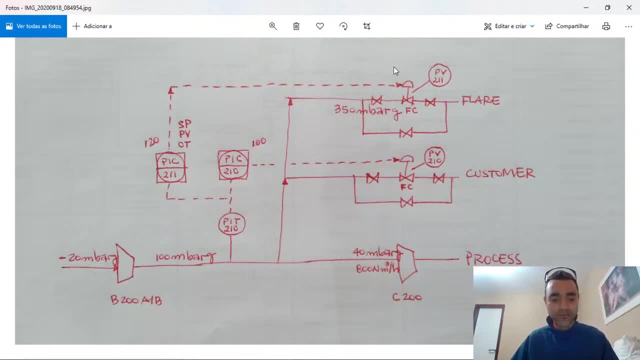 can be feel close, feel open, but there are can be feel close, feel open, but there are others types of fail position, like a others types of fail position, like a others types of fail position, like a fail, stop or fail and it will fail, stop or fail and it will. 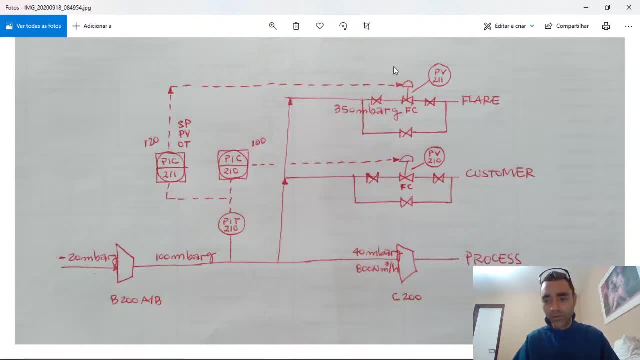 fail, stop or fail, and it will, closing but not automatically, and closing but not automatically, and closing but not automatically. and slowly, slowly, slowly, and something like that and something like that and something like that, and another important inform, and another important inform, and another important inform, another important thing that you, you should. 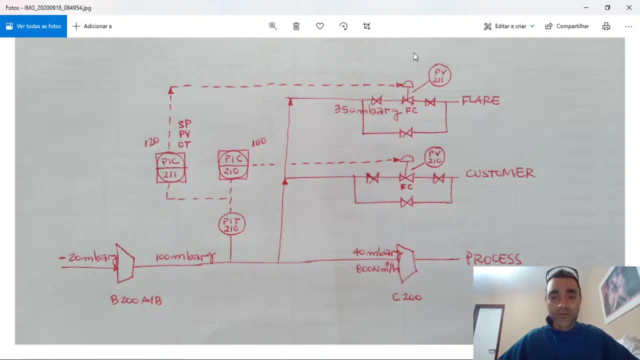 another important thing that you, you should, another important thing that you, you should know, know, know, is how to calculate the cv of the valve, is how to calculate the cv of the valve, is how to calculate the cv of the valve. and i receive a question related about. 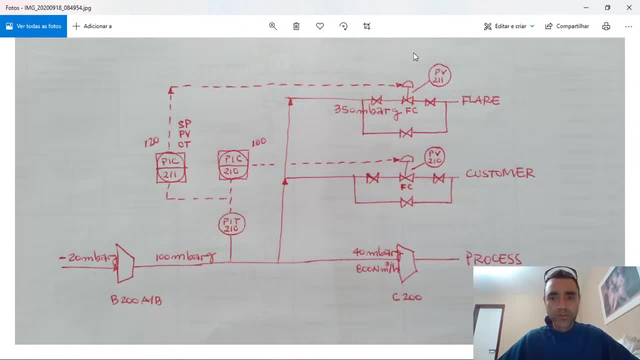 and i receive a question related about, and i receive a question related about that, that that to today or tomorrow, i'm not so sure. to today or tomorrow, i'm not so sure. to today or tomorrow, i'm not so sure. and from a student, from my training: 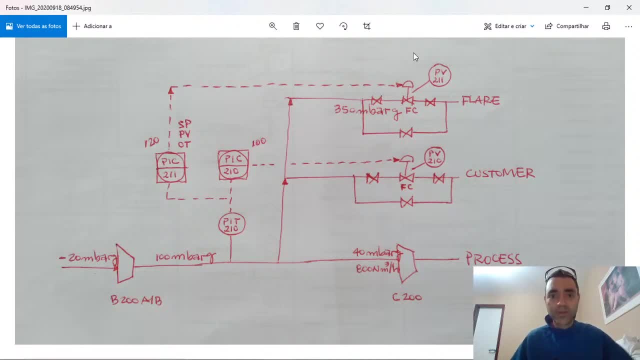 and from a student from my training and from a student from my training program program program. and when we we do the process simulation and when we we do the process simulation and when we we do the process simulation, we, we, we, we need to do the process simulation with. 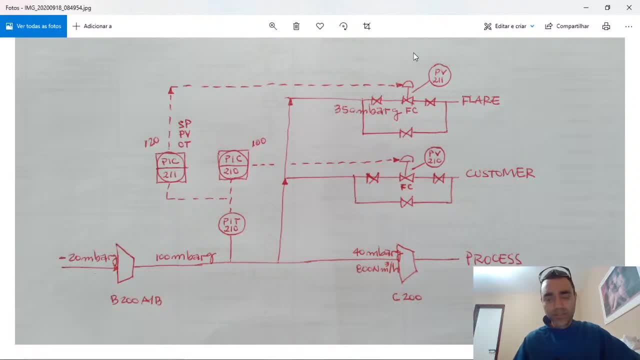 we need to do the process simulation with. we need to do the process simulation with the design conditions, the design conditions, the design conditions and the design conditions can be the and. the design conditions can be the and the design conditions can be the average or can be the maximum capacity. 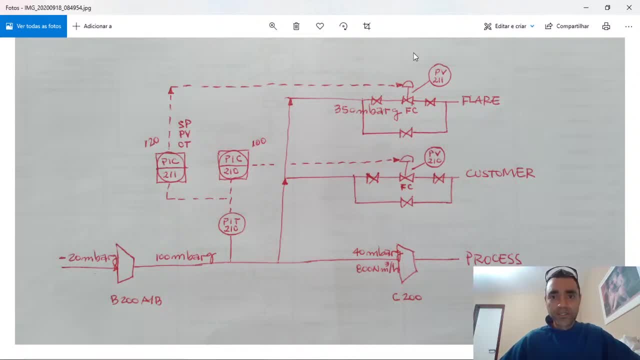 average or can be the maximum capacity. average or can be the maximum capacity, depending, depending, depending on the purpose of your process, on the purpose of your process, on the purpose of your process, simulation, but what matters is that for simulation, but what matters is that for simulation, but what matters is that for cv calculation, we should consider the 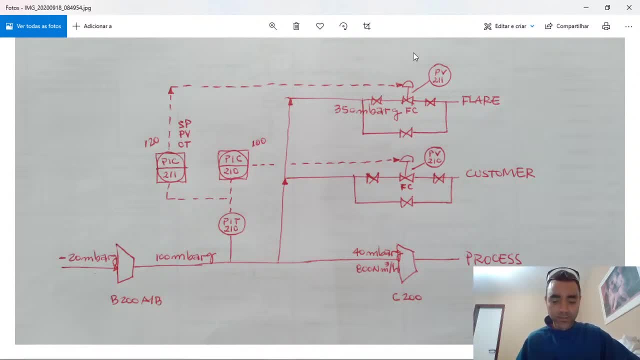 cv calculation. we should consider the cv calculation. we should consider the maximum maximum, maximum value at operations. so let's suppose value at operations. so let's suppose value at operations. so let's suppose that in the average i will, that in the average i will, that in the average i will. i will have a flow here of 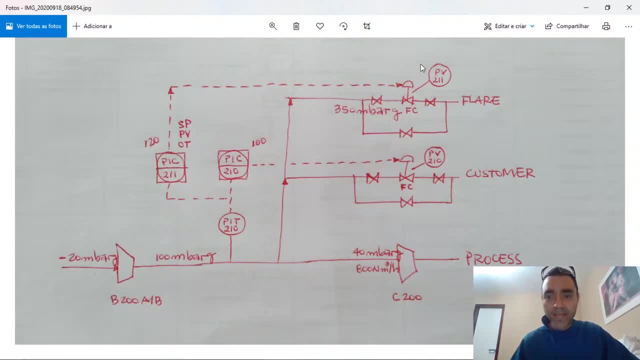 i will have a flow here of: i will have a flow here of 800 normal cubic meters per hour. 800 normal cubic meters per hour, 800 normal cubic meters per hour passing through dpv to the flare, passing through dpv to the flare, passing through dpv to the flare, and but i know that is possible, that i 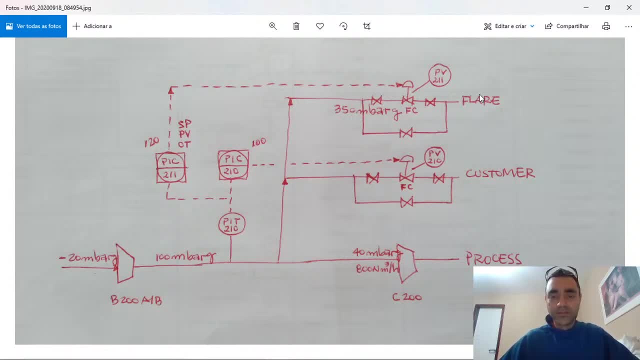 and, but i know that is possible that i and, but i know that is possible that i can have- can have, for instance, 1200, for instance 1200, for instance 1200. so i will calculate the cv of this valve. so i will calculate the cv of this valve. 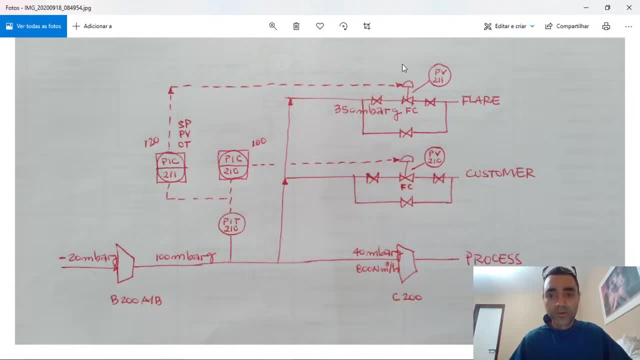 so i will calculate the cv of this valve based on 1200 normal cubic meters, based on 1200 normal cubic meters, based on 1200 normal cubic meters and not in 80 100, 80 and not in 80 100 80. 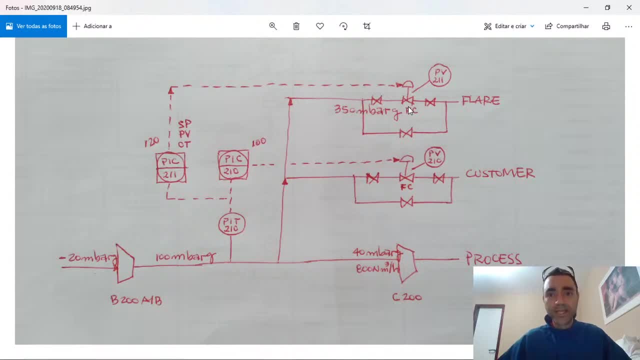 and not in 80, 100, 80, 100 normal cubic meters and we'll we'll do 100 normal cubic meters and we'll we'll do 100 normal cubic meters and we'll we'll do that because we need to evaluate the that, because we need to evaluate the. 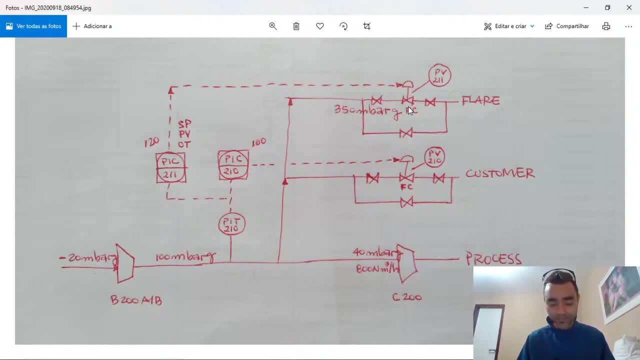 that because we need to evaluate the range of operation of our control valves. range of operation of our control valves, range of operation of our control valves, so depending on the type of the control, so depending on the type of the control, so depending on the type of the control valve. 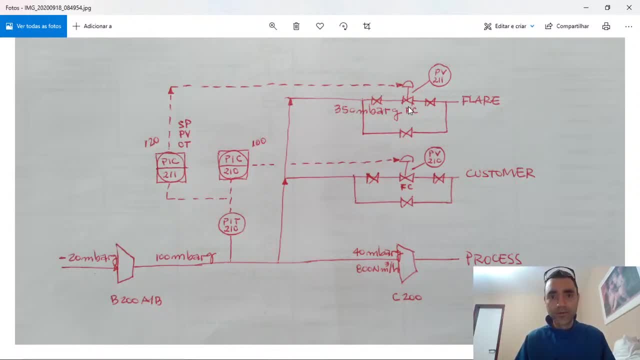 valve valve. it will have a best range of. it will have a best range of. it will have a best range of operations and if it is a globe type, it operations. and if it is a globe type, it operations. and if it is a globe type, it will be. 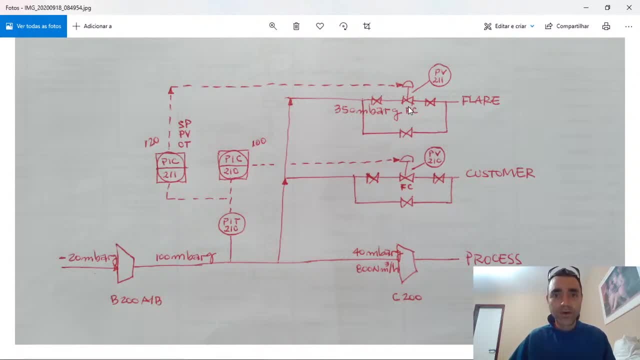 will be will be one one, one range. if it is a ball type, one one, one range. if it is a ball type, one one, one range. if it is a ball type, it will be another range, and if it is a, it will be another range, and if it is a. 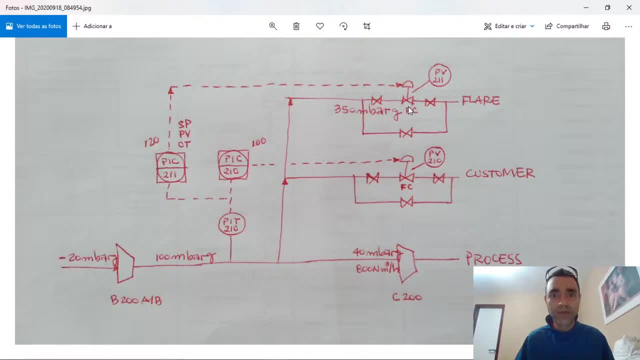 it will be another range. and if it is a butterfly valve, butterfly valve, butterfly valve, each kind of valve will have its own. each kind of valve will have its own. each kind of valve will have its own characteristics, characteristics, characteristics. so what we usually set at the the 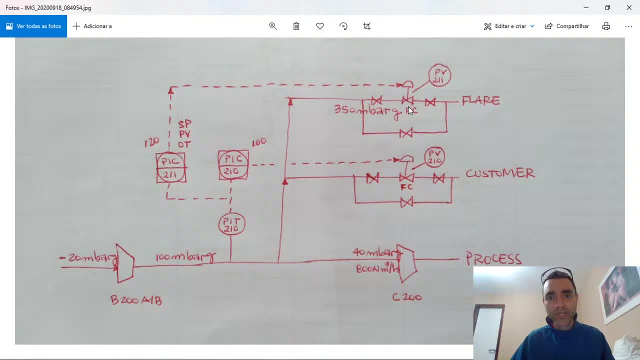 so what we usually set at the the. so what we usually set at the, the program and the, the best program and the, the best program and the the best estimate. in fact, a control valve is use estimate. in fact, a control valve is use estimate. in fact, a control valve is use, the supplier, the supplier. 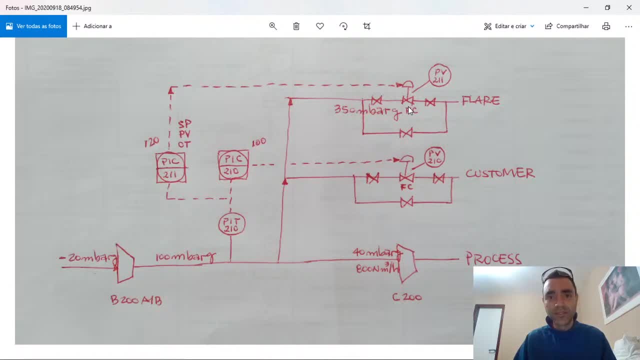 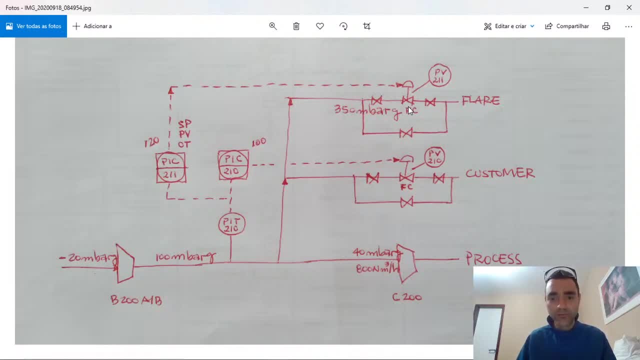 and with that we can predict, and with that we can predict the, the, the, the size of the control valve, and it is the size of the control valve. and it is the size of the control valve and it is important to, important to important to predict or to estimate the size of the. 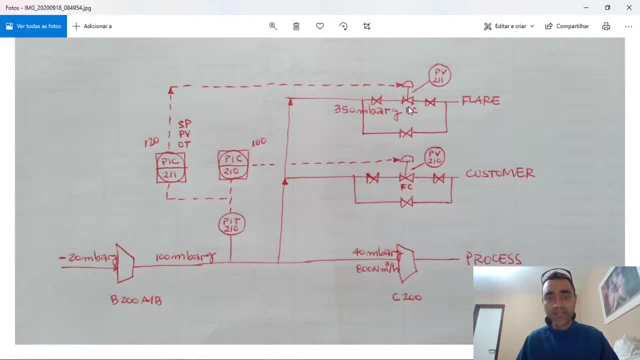 predict or to estimate the size of the predict or to estimate the size of the control valve, control valve, control valve. because with that at the preliminary, because with that at the preliminary, because with that at the preliminary stages of the stages, of the stages of the, the, of the, the project, we can the, the pipe. 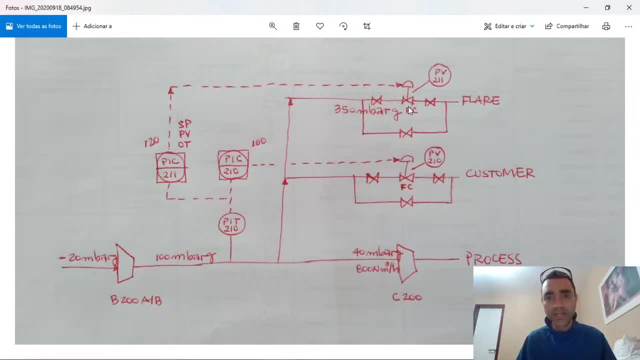 the of the the project. we can the the pipe. the of the the project. we can the the pipe. engineer can verify. engineer can verify. engineer can verify the fittings that must be added to the. the fittings that must be added to the. the fittings that must be added to the pipeline. pipeline, pipeline, and it much, much often the, and it much, much often the, and it much, much often. the size of the control valve is smaller, size of the control valve is smaller, size of the control valve is smaller than the pipe size, than the pipe size, than the pipe size and. 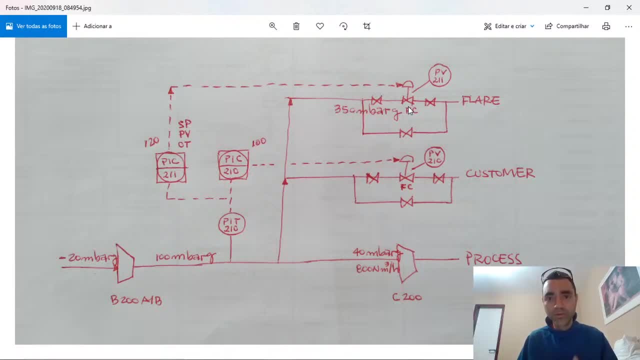 and and talking about control. if we are talking, talking about control. if we are talking, talking about control. if we are talking about insulate in, about insulate in, about insulate in isolation valves- usually it is the same isolation valves. usually it is the same isolation valves. usually it is the same size of the the pipeline. 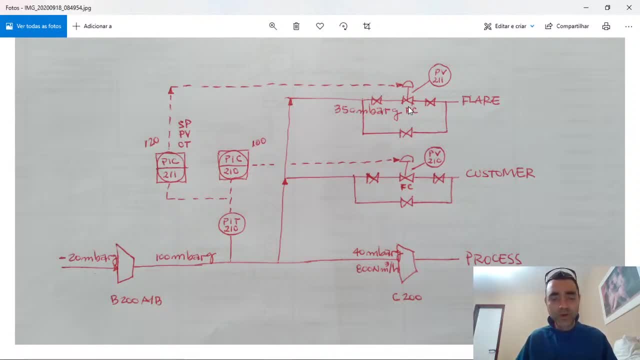 size of the, the pipeline, size of the, the pipeline. so if i calculated a, so if i calculated a, so if i calculated a four inches pipeline, and i did four inches pipeline, and i did four inches pipeline and i did the, the preliminary sizing of the control, the, the preliminary sizing of the control. 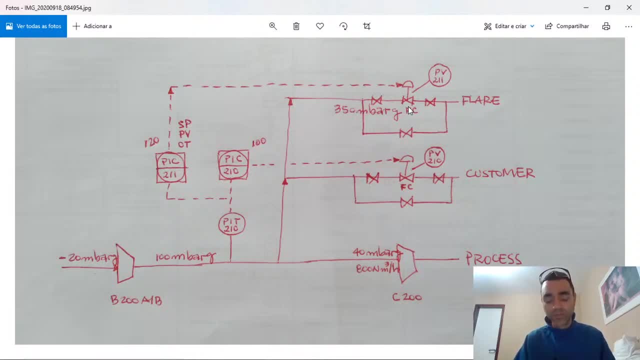 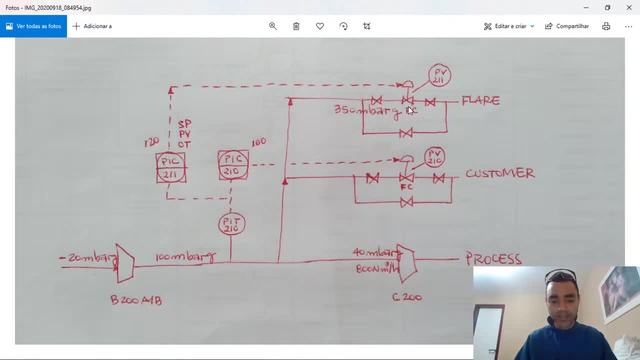 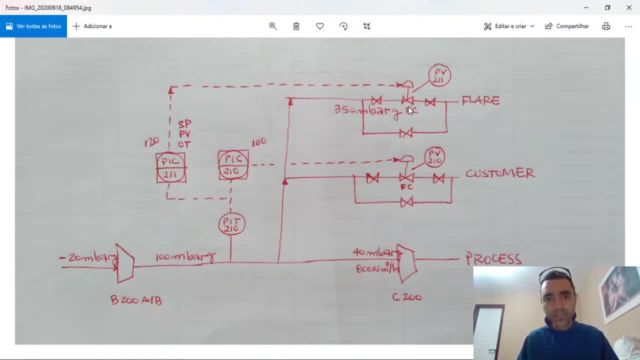 valve because a control valve, a six valve because a control valve, a six inches control valve. inches control valve, inches control valve- uh, globe six inches control valve is uh globe six inches control valve is uh globe six inches control valve is. he has a different, different price than 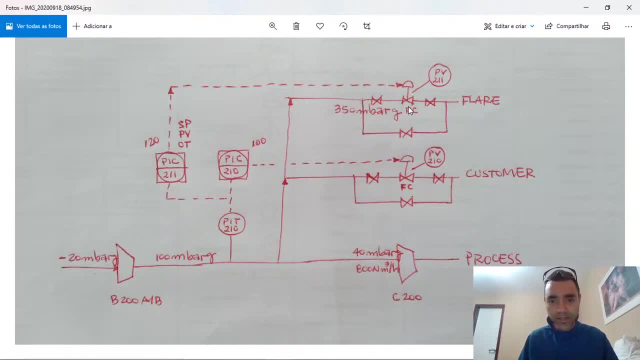 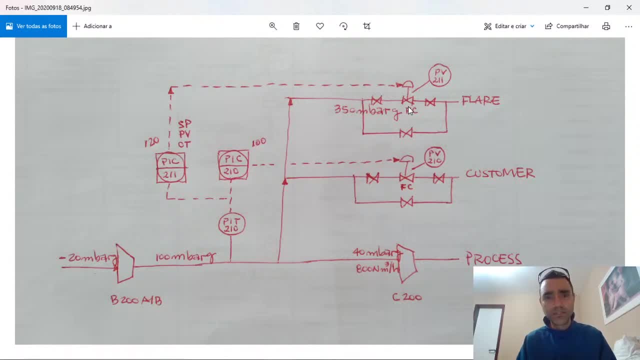 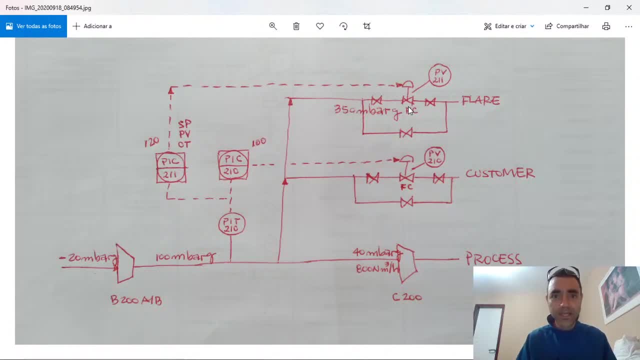 it's, it's more, it's more likely to do that in the basic engineering, that in the basic engineering, that in the basic engineering and in the detail engineering can be a, and in the detail engineering can be a, and in the detail engineering can be a revision on that, and 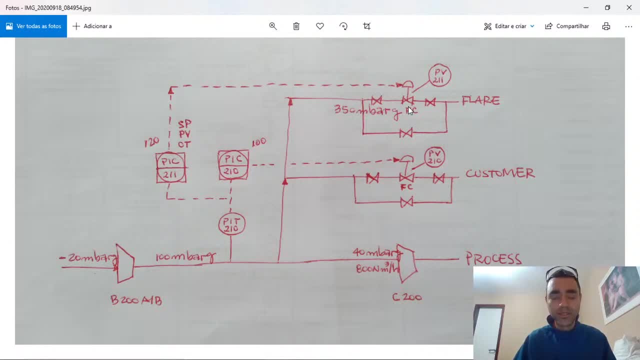 revision on that and revision on that. and do the push the purchase and the do the push the purchase and the do the push the purchase and the delivering to the field, delivering to the field, delivering to the field. so so so, my field, my, my, my field, my, my. 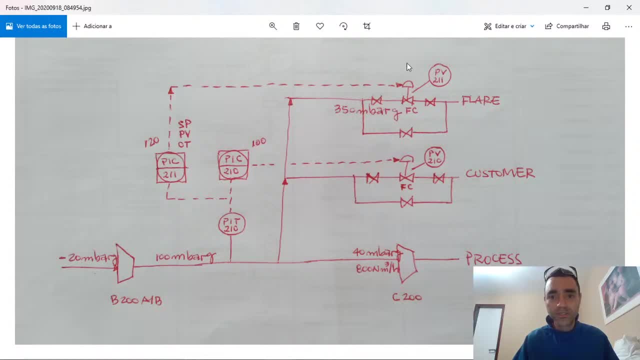 my field, my, my, my tip here, or my information here to you, my tip here, or my information here to you, my tip here, or my information here to you about dcv sizing is about dcv sizing is about. dcv sizing is one: consider the maximum. one consider the maximum. 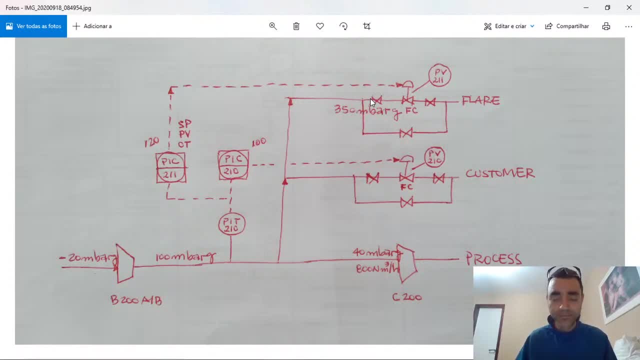 one consider the maximum operating operating flow that you can operating operating flow that you can operating operating flow that you can have, have, have, and you will add also the, and you will add also the and you will add also the normal flow that is expected and you will be. 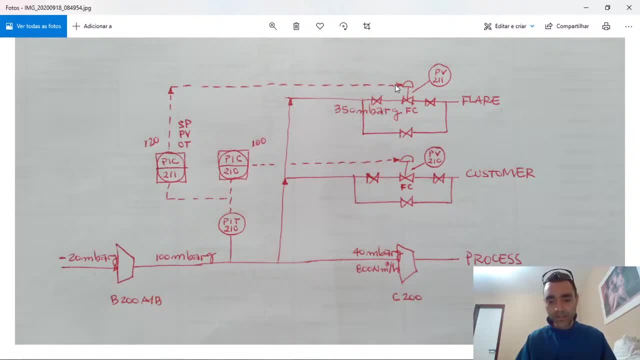 normal flow. that is expected and you will be normal flow. that is expected, and you will be able to see able to see able to see the, the graph, the, and if the, the, the, the graph, the, and if the, the, the, the graph, the, and if the, the points of operation that you expected. 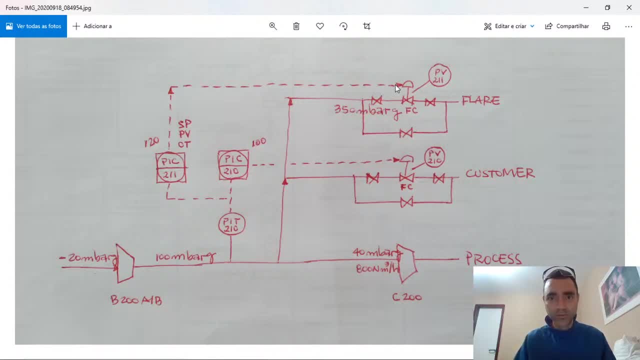 points of operation that you expected, points of operation that you expected expected to have is between the range of expected to have is between the range of expected to have is between the range of control of the valve, control of the valve, control of the valve, and another another. 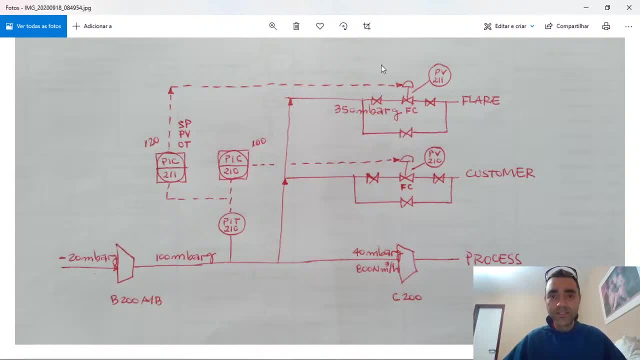 and another, another and another another. information that is important here. information that is important here. information that is important here: during your cv sizing is about the during your cv sizing is about the during your cv sizing is about the noise and noise, and noise, and and the noise is. 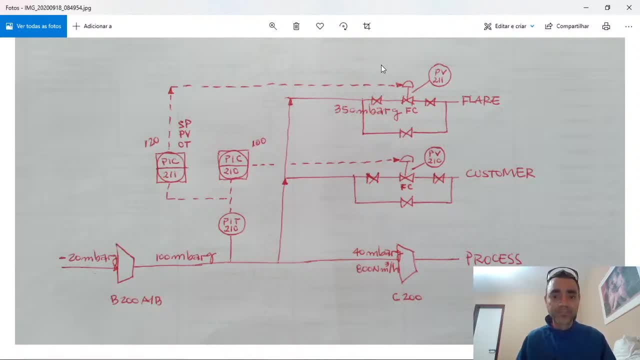 and the noise is, and the noise is related to the, related to the, related to the mac number, mac number, mac number, and i received today another question and i received today another question and i received today another question related to this subject and related to this subject, and. 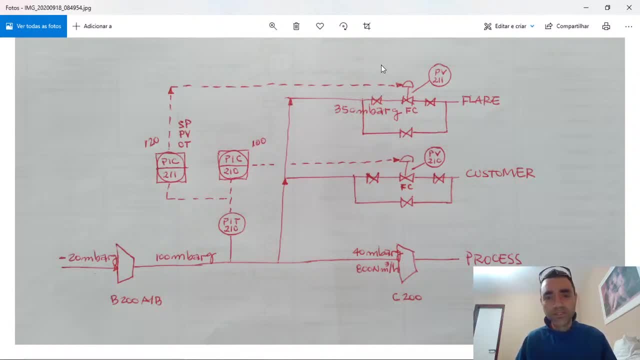 related to this subject and it it it talked to, talked to, talked to the. the question was the. the question was the. the question was: the question was the. the question was the question was: if the, if the, if the choke choke condition is choke choke condition is choke choke condition is is good or not, or if it's bad. i think 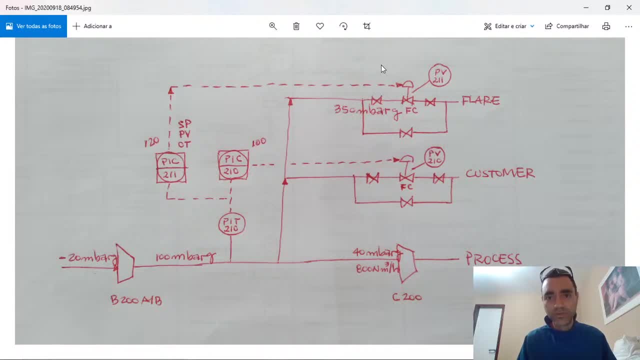 is good or not, or if it's bad. i think is good or not, or if it's bad. i think that it was something like this, that it was something like this. that it was something like this is the choke condition at the control. is the choke condition at the control. 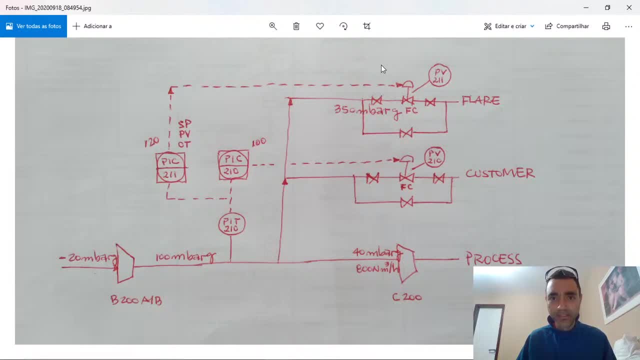 is the choke condition at the control valve. bad valve, bad valve, bad, bad, it's not bad, it is bad, it's not bad, it is bad, it's not bad. it is a condition of the process. when you a condition of the process, when you a condition of the process when you have a big differential pressure. have a big differential pressure, have a big differential pressure, the, the, the, and considering that you have a fixed and considering that you have a fixed and considering that you have a fixed orifice size, orifice size. orifice size when you reach the choked condition it. when you reach the choked condition, it. 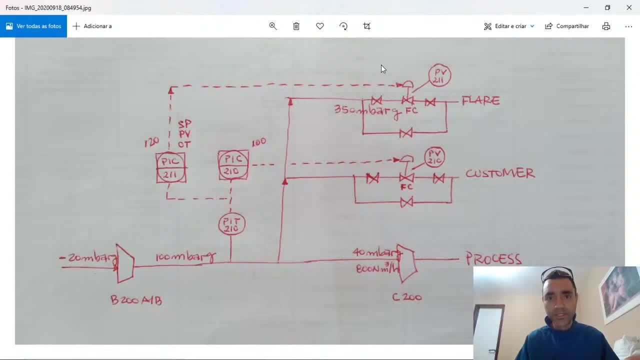 when you reach the choked condition. it means that, even though you means that, even though you means that, even though you you increase the press, the the pressure, you increase the press, the, the pressure, you increase the press, the the pressure drop, drop, drop, you will not have more flow through the. 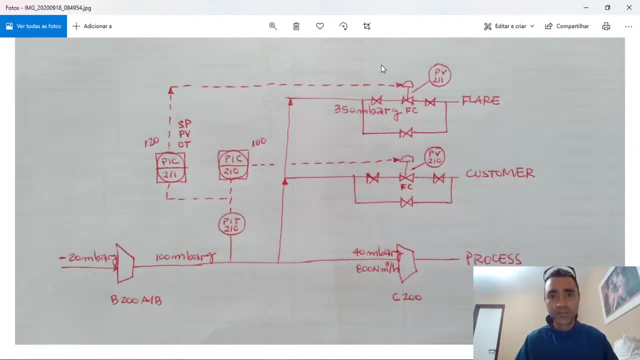 you will not have more flow through the. you will not have more flow through the, through the orifice, because it through the orifice, because it through the orifice, because it it reached the choked conditions, it reached the choked conditions, it reached the choked conditions and what is? 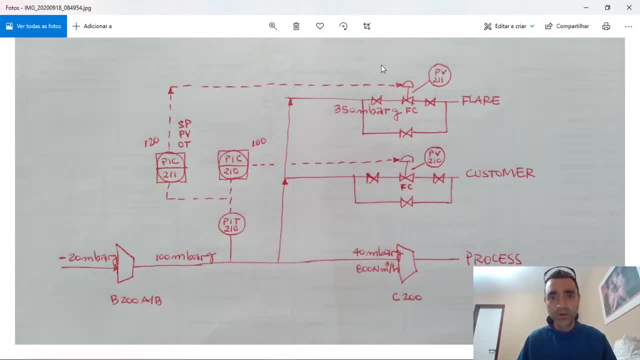 and what is and what is important in the valve is that you important in the valve, is that you important in the valve is that you prevent having no, prevent having no, prevent having no noising and it is related to the mac: noising and it is related to the mac. 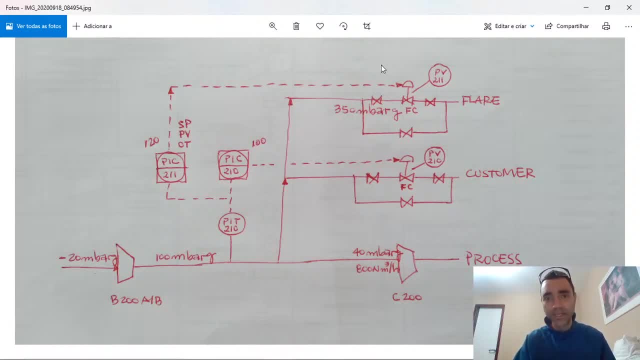 noising and it is related to the mac number, because if the mac number, because if the mac number, because if the mac numbers and the mac number is related numbers and the mac number is related numbers, and the mac number is related to the, to the, to the, the speed of sound, if you have a, 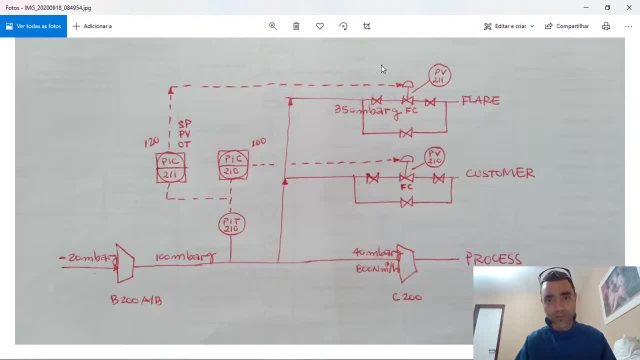 the speed of sound if you have a, the speed of sound if you have a too big mac number. you will have too big mac number, you will have too big mac number, you will have noise, very noise, and you will have noise, very noise, and you will have 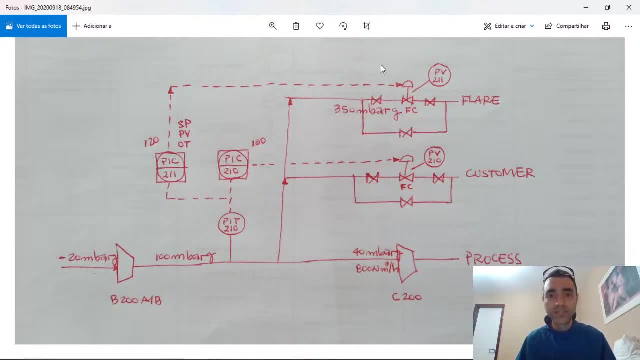 noise, very noise, and you will have also vibration in the valve and that also vibration in the valve, and that also vibration in the valve, and that vibration can, vibration can, vibration can can lead to uh to the can lead to uh to the can lead to uh to the to your control valve broke and or not. 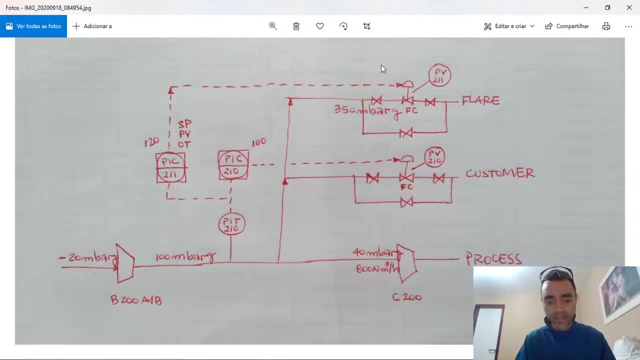 to your control valve broke and or not, to your control valve broke and or not. control, control, control. uh not do the the kind of control that uh not do the the kind of control that uh not do the the kind of control that should be, should be, should be done, and what is? 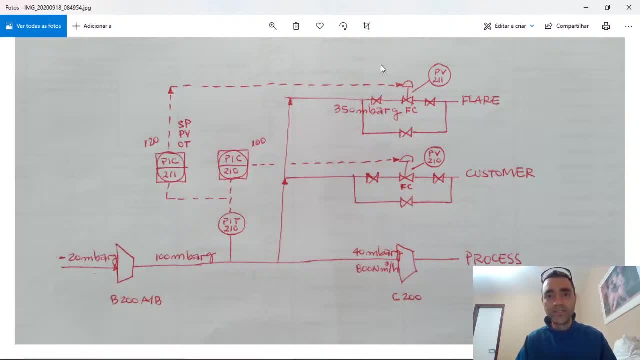 done and what is done and what is we can do in this in this case, is we can do in this in this case, is we can do in this in this case is increase, increase, increase the the orifice of the valve or the the orifice of the valve or. 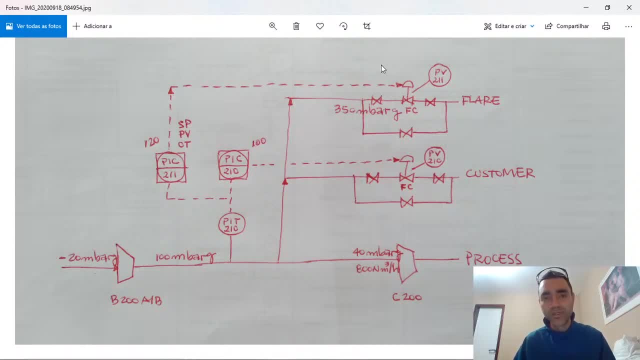 the, the orifice of the valve, or change the type of the valve to reduce. change the type of the valve to reduce. change the type of the valve to reduce the, the mac number, and with that to the, the mac number, and with that to the, the mac number, and with that to reduce the vibration and with that to 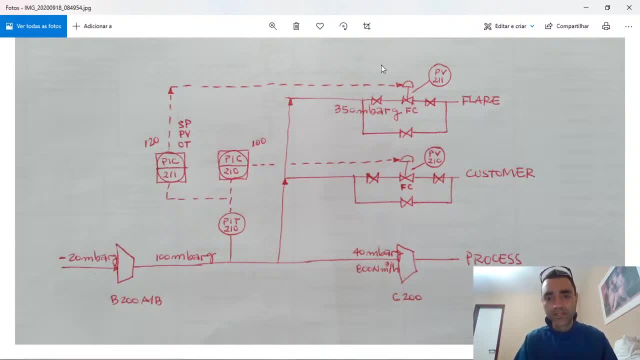 reduce the vibration and with that to reduce the vibration, and with that to reduce, reduce the, reduce the, reduce the. the noise of the system. so what? the noise of the system? so what? the noise of the system? so what we, we, we, we do during the, the sizing of the. 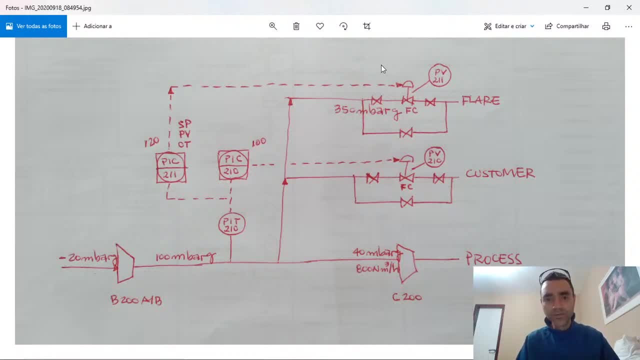 we do during the, the sizing of the, we do during the, the sizing of the control valve, control valve. control valve is to to inform the process conditions, is to to inform the process conditions, is to to inform the process conditions and to the supplier, and we can use that. 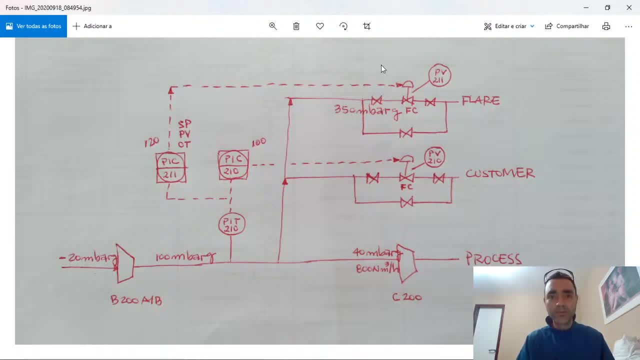 and to the supplier, and we can use that. and to the supplier, and we can use that in the in the supply software, in the in the supply software, in the in the supply software and we need to evaluate if the results. and we need to evaluate if the results. 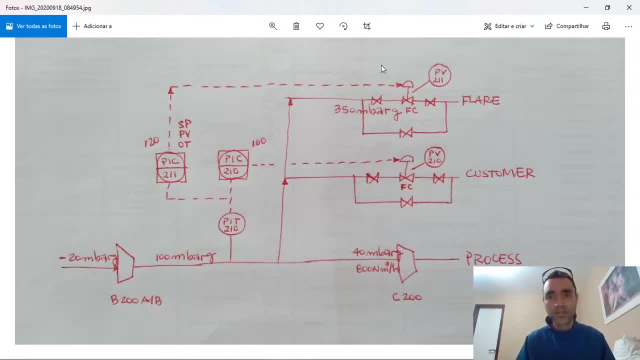 and we need to evaluate if the results from that conditions and, of course, that from that conditions and of course that from that conditions and of course, that conditions, conditions. conditions includes the. the fluid includes the. the fluid includes the. the fluid, the properties and the process conditions. the properties and the process conditions. 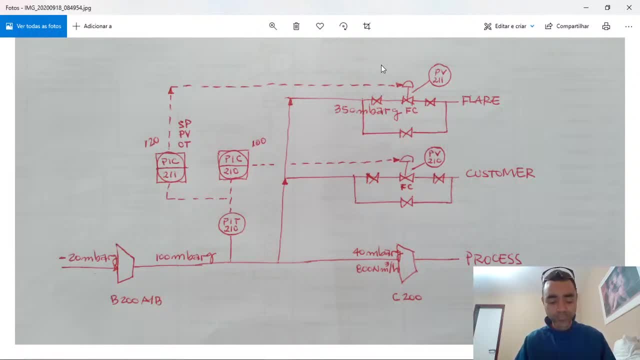 the properties and the process conditions in process conditions, is flow in process conditions, is flow in process conditions, is flow pressure and temperature. all of these pressure and temperature, all of these pressure and temperature, all of these will result in a cv calculated, will result in a cv calculated. 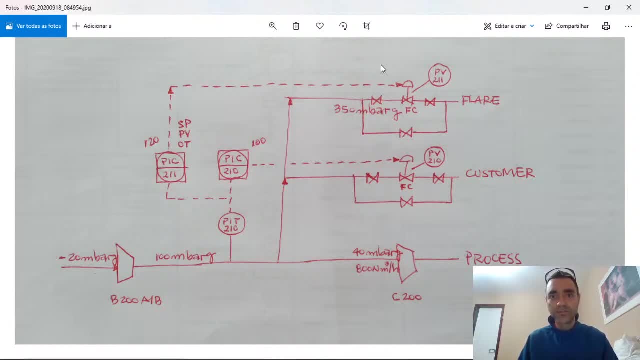 will result in a cv calculated and, and, and. most often, this view calculated is not. most often this view calculated is not. most often, this view calculated is not the cv, the cv, the cv that will be installed in the field. that will be installed in the field. that will be installed in the field because, as we have in the 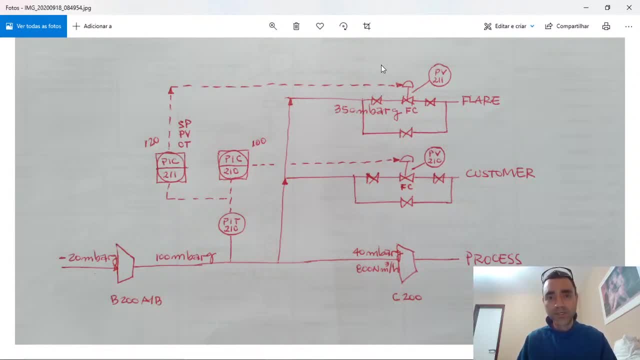 because, as we have in the, because, as we have in the, we have the same to the, we have the same to the, we have the same to the control valves: the- the suppliers do control valves, the the suppliers do control valves, the the suppliers do standards control valves. so there is a 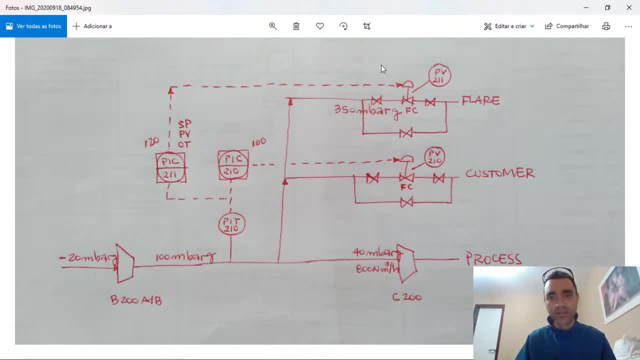 standards control valves. so there is a standards control valves, so there is a, a set, a set, a set of control valves that fits a range of of control valves. that fits a range of of control valves. that fits a range of cvs. so cvs, so cvs. so you calculated, for instance, a cv 10. 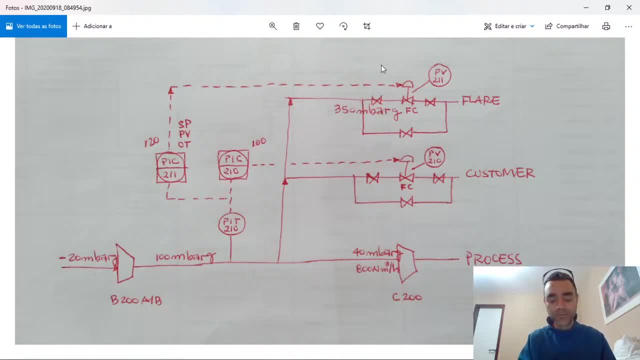 you calculated, for instance, a cv 10. you calculated, for instance, a cv 10 for a process. but if you go to the for a process, but if you go to the for a process, but if you go to the supplier, it only has a cv 12 or cv. 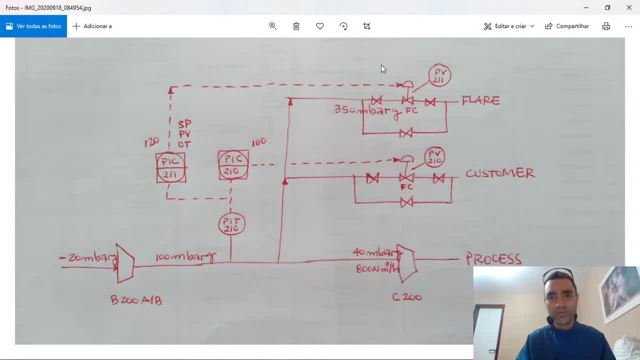 supplier. it only has a cv 12 or cv 15, for instance, and you you will need to buy the cv for uh 12 or 15, of course, evaluating the, the curve of control. and once you you have that you you will have the, the characteristics of the valve, like uh, the noise and the mac how it fits. 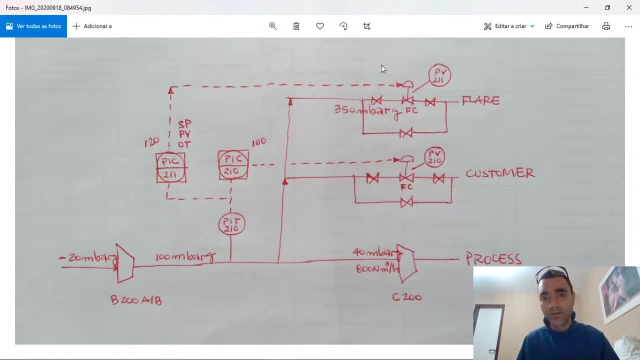 to to your process, and that leads to another subject. but before doing that, nice to have you here. giant, giant carboso is also is also a student of mine in process booster, nice to have you here. and so, uh, we talked about a lot of things, guys, and another another, uh, related to cv. 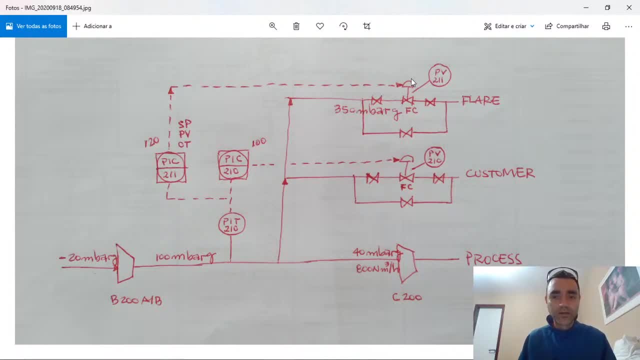 what they have is that one, depending on your process, the, the evaluation of the fail opening position of the valve. that can be an issue, especially if we are talking about pressure pressure valves, because pressure valves means that we need to to control a delta p of a system and in this case i'm releasing the, the pressure. 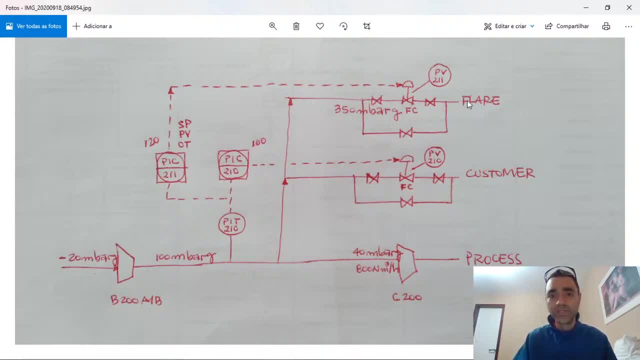 to the, to the flare and it. we could consider that something like a atmosphere. but let's suppose that instead of having the pit at upstream of the pv, we had the pit at downstream of the pv. in this case, we want to control the, the pressure downstream. most often it happens at. 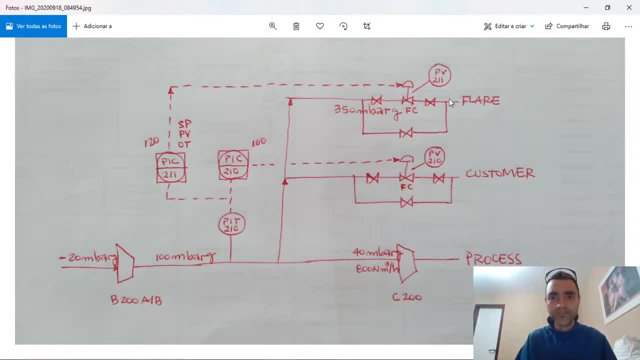 much lower pressure that upstream and in an event that this pv fails, we can over pressurize, over pressurize the downstream of the system. and let's suppose that instead of working with 100 millibar g, i was working with 100 bar g and a downstream of my pv 211. i want. 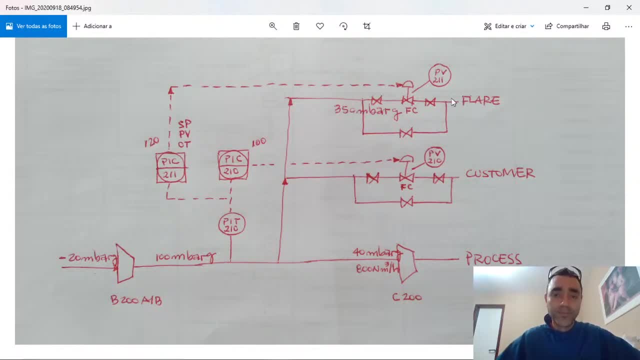 to work with 68 bar g, and it is a example that my my my friend, mohammed hasan, has opened a discussion in lincoln and he was. he would like to to know what is the, what condition he should consider to do the, the, to take the, the mess, mess off of that part of the pv problem. 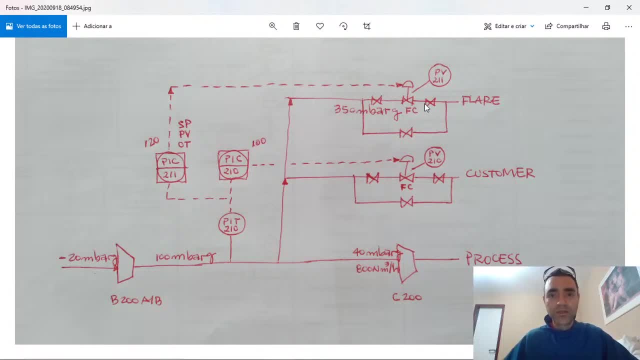 the, the load to the psv that he should add in the system, and he had a series of control valves, i think two control valves in series or three control valves in series, and he had 100 percent, 100 bar at the inlet of the first control valve and in the the end of the process. 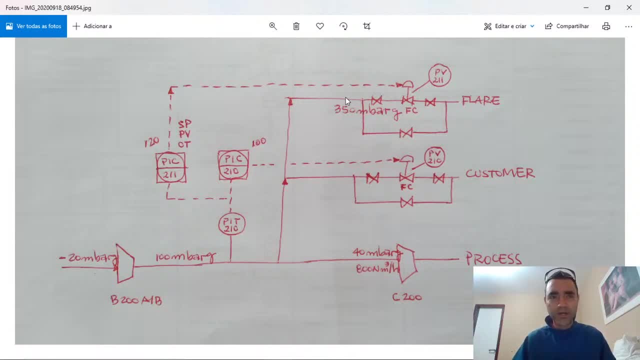 he had a psv with around 15 par g and between the 100 and 15. he was breaking the pressure in order to to get the, the values that he he wanted in the process. so he was discussing how should be calculated the load of the, the psv, and at at 15. 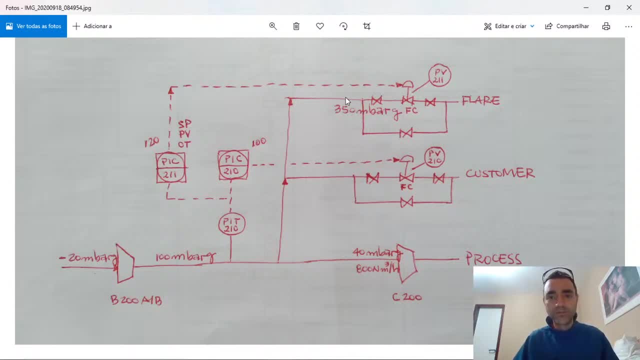 bar g and how should be the schedule of the, the pipeline in in this series? and what i talked to he was that once between the first pspv and the last pv we don't have any psv. he should consider all the system rated to 100 bar g. and why? because if i open this bypass, for instance, i will not have 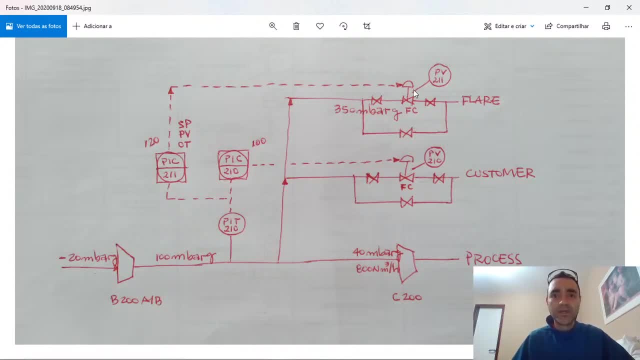 the control valve limitation and if my pv is leaking, i will not have the the control valve limit. i will have the control valve limitation, but i will not prevent the system from over pressurization. and if the, for any reason, the the pid of the controller is not uh right set and we'll talk. about that. it could open too fast and we could have the over pressurization. so what will prevent your system downstream of a control valve to to get overpress, to not rupt because over pressurization is or a psv or, and psv is pressure safety valve and or it can be also a pressure. really. 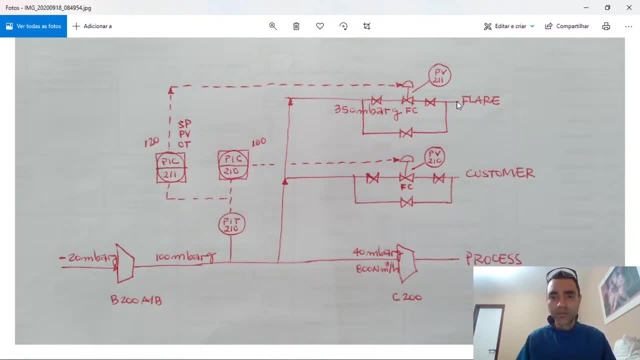 pressure safety device, if you want to, and or the material. and if i rate the material to the, the desire to the maximum pressure of the system, there is no problem. but if my, my material pressure rating is not good, then i will not be able to operate the system. so i will not be able to. 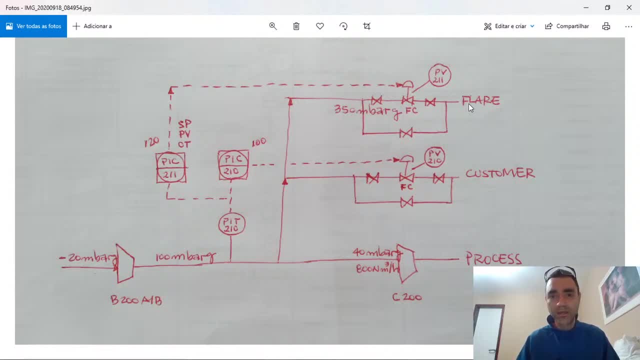 operate the system. so i will not be able to operate the system. so i will not be able to operate the system is below the possible. the maximum uh is is below the maximum available pressure. it is a point to be discussed and evaluated related to process safety. so, returning to the the pressure controller, 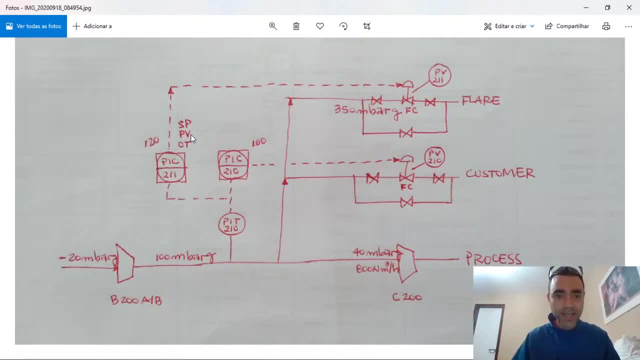 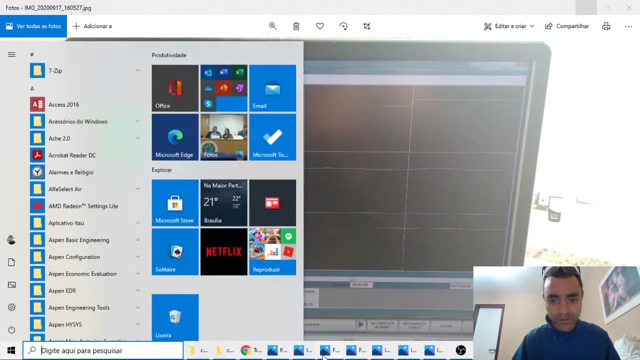 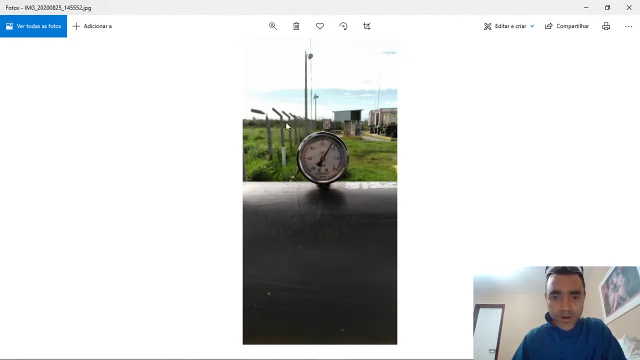 and to, to set the pic, i have three, three main information and before doing that, let me show you some examples here. so here i have, uh, here i have an example of a pressure indicator. so you can see here that i have the information of pressure, and the information of pressure is millibar g. 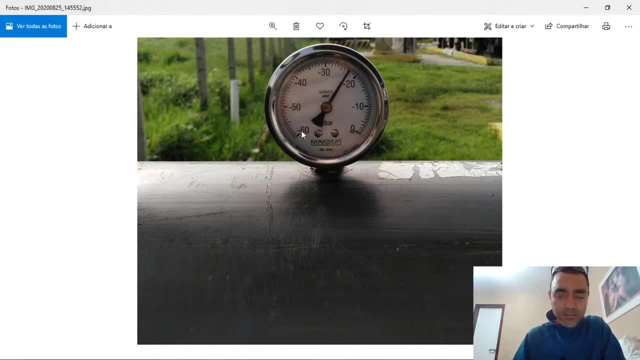 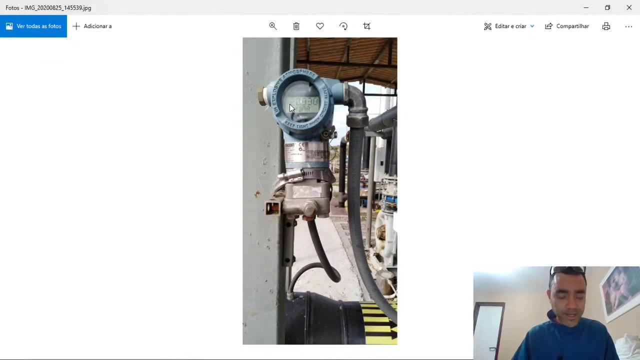 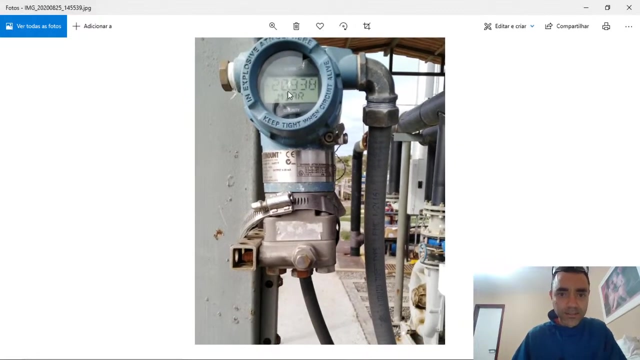 and i can see a range from minus 60 to zero. so this is a pressure indicator and this kind of instrument in the pnid will be identified as pi. it's only a pi. however, i can have a pressure indicator, transmitter a pit, and in this case you can see that i have a pressure indication. it is minus. 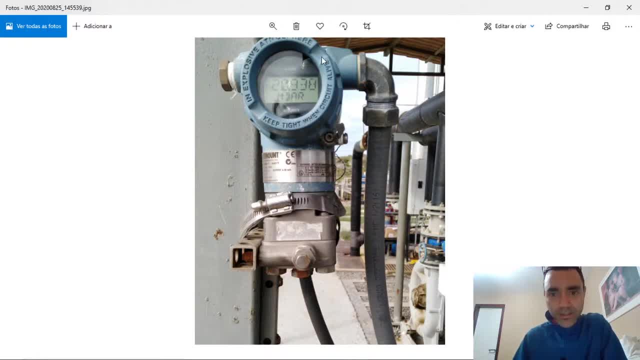 almost 21 millibar g, but i have cables and these cables are for transmitting the information to the plc and also to receive electrical power to, to, to allow the working of this device. so we can see also that it is proper to explosive atmosphere and it is a uh. 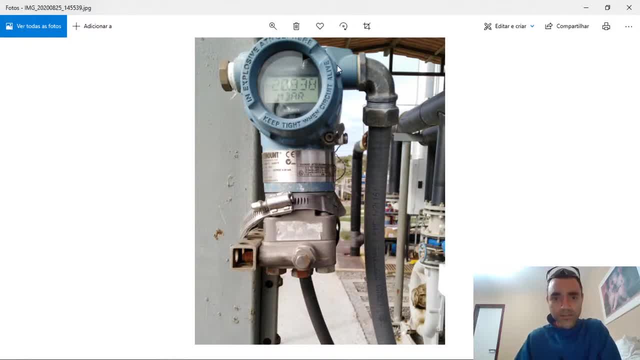 it's special guys, a special kind of enclosure to not to not have any kind of sparkle and uh hollow and some uh uh explosion or other things like that. so that's all what we can have here today: some explosion or a sparkle to a flammable gas and something like that. so what matters here is that. 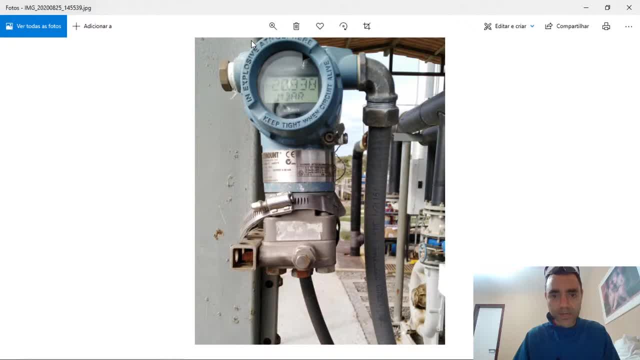 we have a pressure in the pressure measurement, but it is also an indicator and it is a transmitter. and this, this kind of instrument, is able to send the signal to the control room. the other one, the pi or the manometer, is only the operator, is only able to, to read the measurement at the field. you 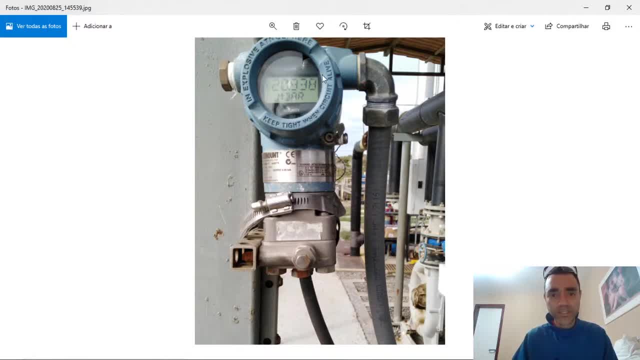 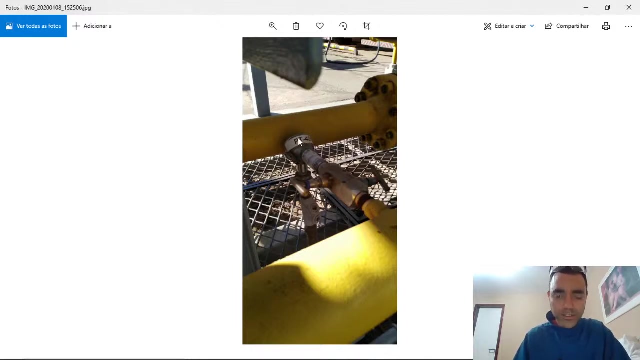 know he, we can read the measurement at the field and also in the control room, because the signal goes to the plc and if we have a supervisory it will get the information and something like that, and finally him. what else matters here is here. i have a pt and it is a pressure measurement device also. 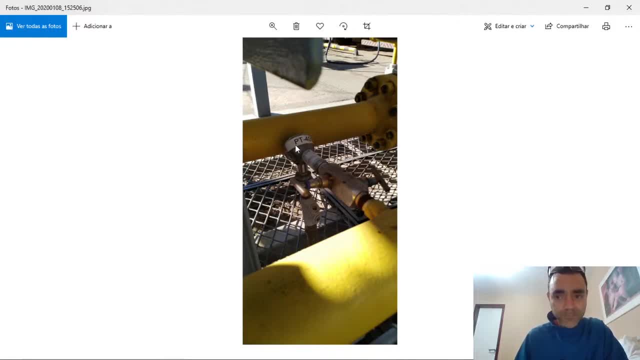 and in this case i don't have the di, that is the indication. i have only the pressure and the transmitter and you can see some cables here- and he has the electrical information to the plc and something like that. so in the, in your piano, id see these three kinds of of information. it can be a PI and it can be a PI in the. 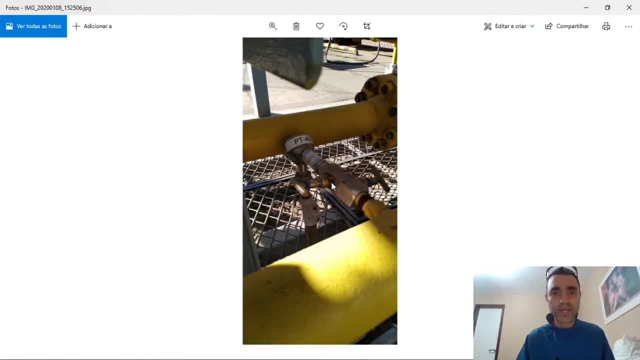 field only, or you can have a virtual PI in the control room and it will be possible to have the PI in the control room or the screen of the control, the screen operation screen, only if you have a pressure transmitter and the pressure transmitter can have an indicator in the field. so in this case is a PIT or it. 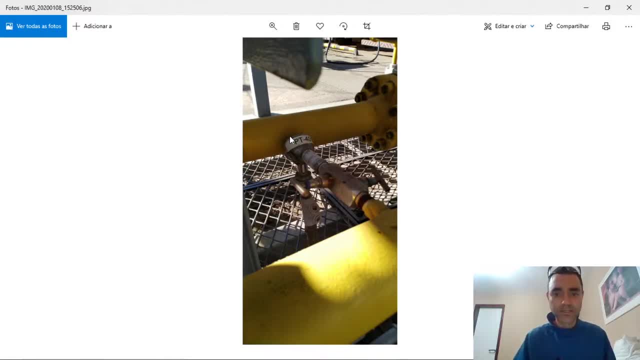 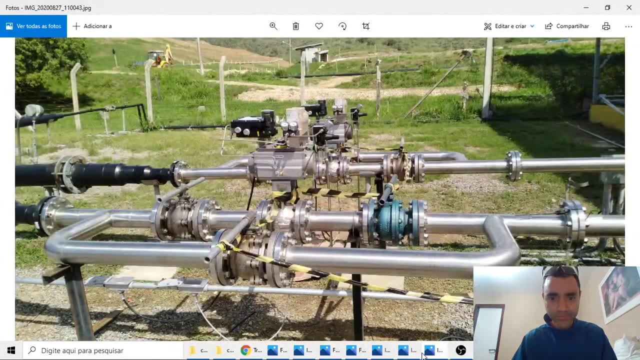 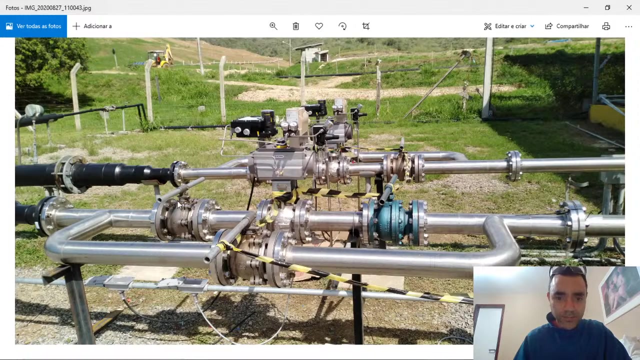 can be only a transmitter and in this case the only. the signal goes to the goes to the PLC, into the control room. here is the system that I showing you. so we have the system that I showing you. so we have the block, the isolation valve, we have the bypass valve in the control. 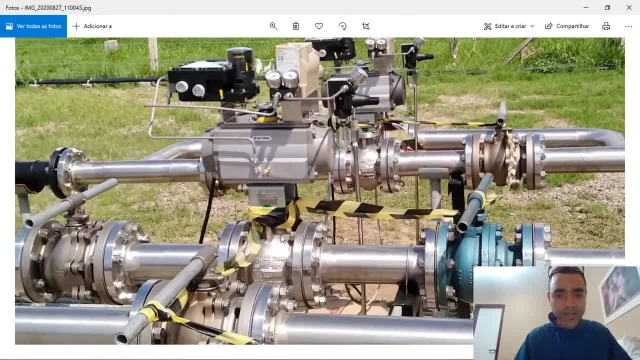 valve and in this case the control valve has a controller and there is the instrument air going to the control valve and in this case it is closed it and we have a positioning, and sometimes we don't have this kind of positioning in the control valve, but we have a reference for the opening. 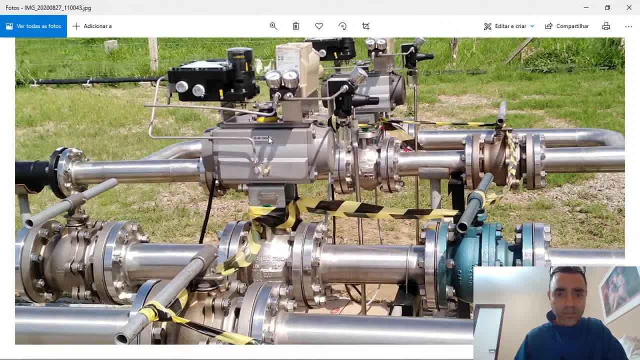 and we can see here, once the, the control valve opens- and it is a kind of segment valve- it will run, it will go to the left or to the right in order to to open more the, the, the orifice they do, the opening of the control valve. 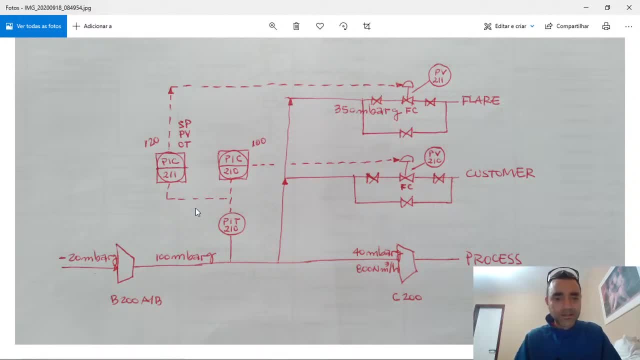 okay, guys. so now, what I want to to show you is the. I will talk to you about the, about the tuning of the control valve. so what is the tuning of the control valve? QUE U Zięc verrán? The settings of PID of your controller, in order that your valve fits to the process. 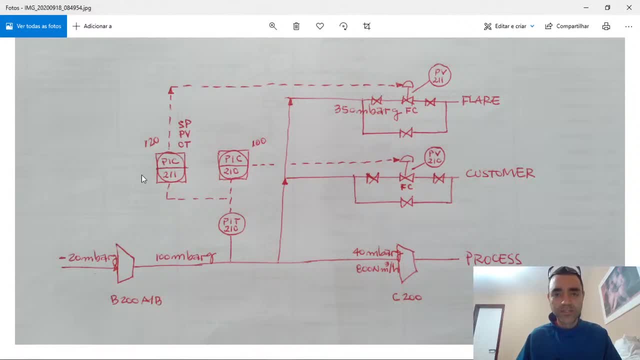 It controls the pressure of the system based on the variation of the pressure, And an example of PID graph you can see in the thumbnail of this live session. There is a graph with different integration numbers and depending on that, we open the valve more, faster or slower. 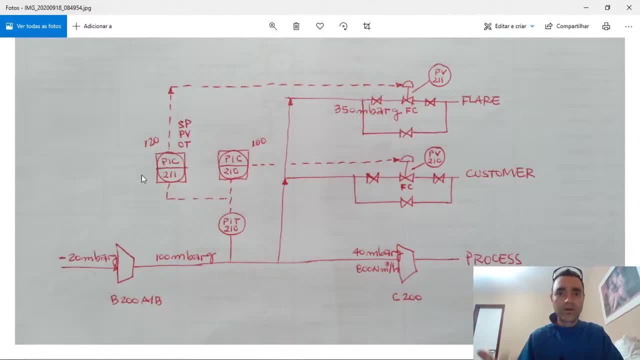 Depending on the proportion we open more or we open less. And to evaluate if your PID settings is ok, You need to know about SP, About PV And about OT. The PV is the set point, It is your target. So in this case I want to 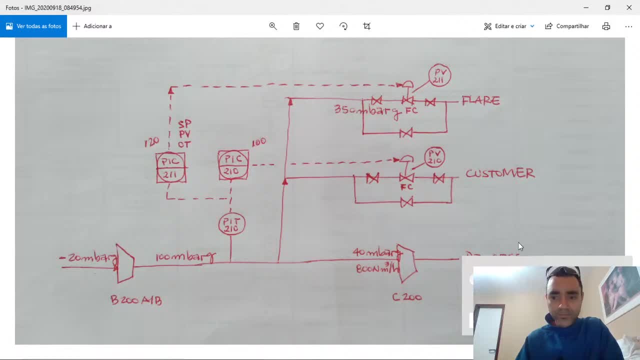 I set my system. I set my system At 120.. So once this valve is opening, I want to reach 120. And I don't want to. I don't want to operate at 130, I don't want to operate at 150, I don't want to operate at 100, I want to get 120. so this is the set point of my controller. however, the, the, the real value that the, the transmitter, is reading, is shown in the PV, and PV is the PID of the system. 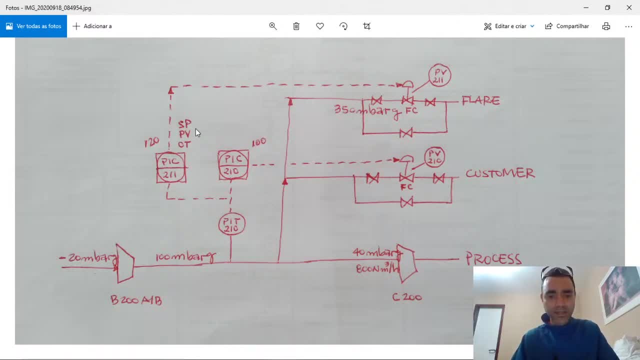 The V is the present value. it means that the instrument is measuring, is measuring the this value. at that time and based on the set point and based on the present value, the controller will define a signal of outputs, It will define an output and that output will will be sent to the controller. 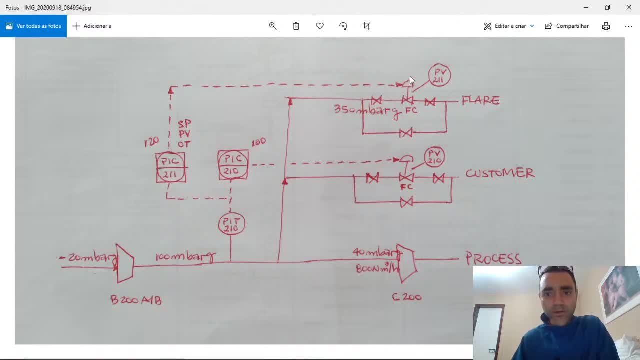 In order that, Opening more or closing more, The PV will get closer to the set point. because, in the end, what we want is that the set point be equal to the The PV. in fact, we want to the PV to be we equal to the set point. and if your process is well tuned in, sometimes it is easier, sometimes it's not so easy. 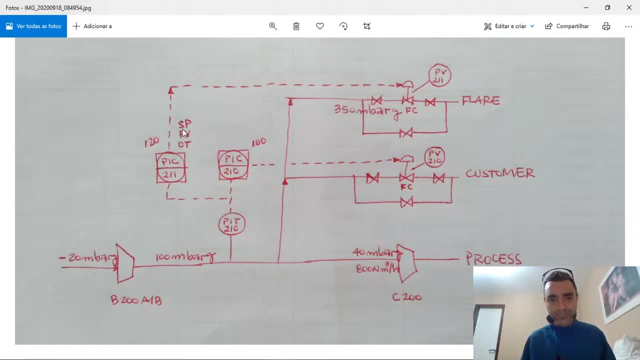 You will get That and your Your. the graph of variables, you will see, will be a straight line if your process is stable, or it will be a solenoid Line, because if it is not so stable or if your tuning is not doing so good, 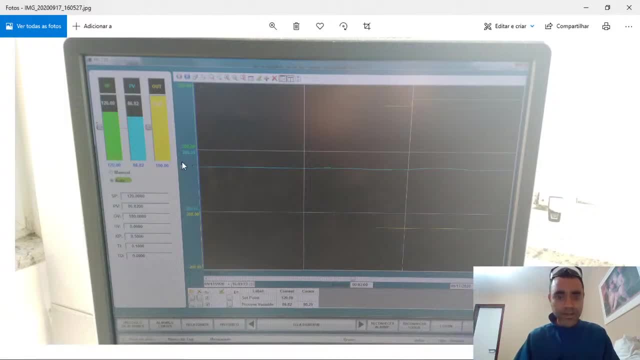 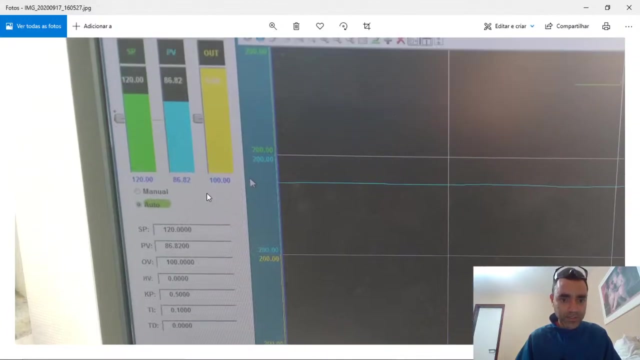 So, Based on that- And this photo is not so Good, sorry- it was Sunny, Sunny, sunny day and the there there are windows behind the control, the screen, so sorry for that, but what we can see here at first is that we have the. 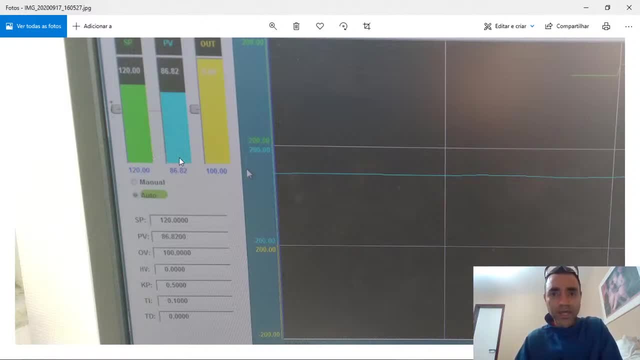 The op. in this case we have options to have the controller at the manual or at automatic. And if I set the control to manual, it means that to open or to close the control valve, I need to define. I needed to define a value of output. 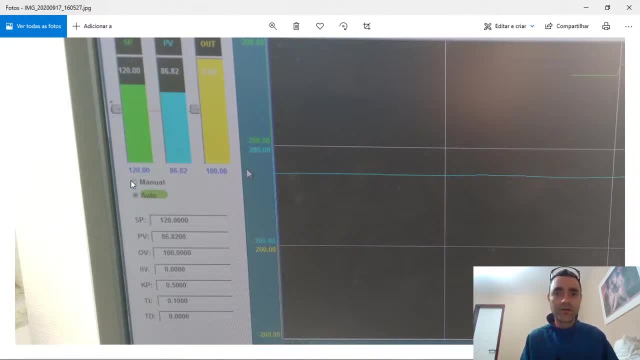 And the, how it is configurated or how it is program. it depends on the, the philosophy of the company. In this company, for instance, they shift or they separate The OV from the Hand value Input. So in this case, here, If I 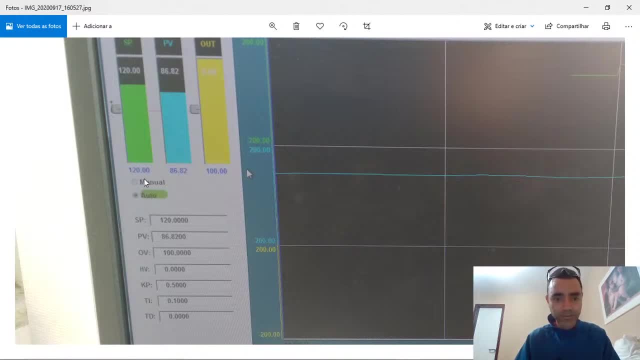 I set my control at manual. What will happen Is that the I will need to define A value at the HV- And HV in this case means hand value- To open or close my My valve, For instance. Let's suppose that I set for manual. 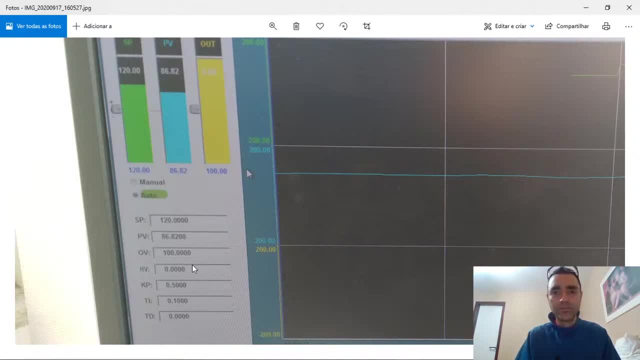 And I want to open the control valve at 25%. So I will would type 25% at the HV And my valve would open 25%. Or if I want to change to 65. I would do the same And something like that. 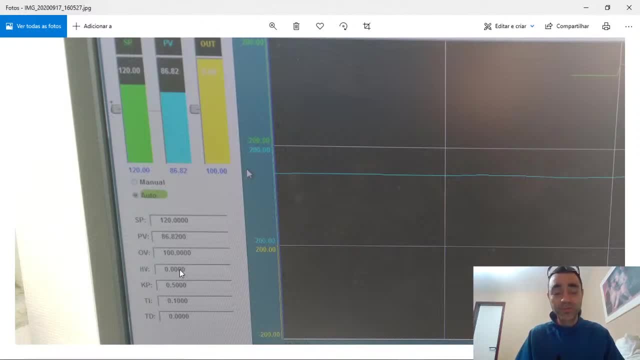 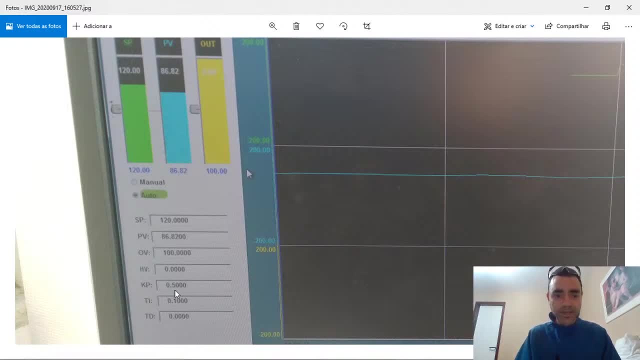 And the derivative of the controller, And It has a calculation And there are methods To do Estimates of this value. But, to be sincere, As a chemical process engineer- I work with plant design- I never did any kind of calculation. 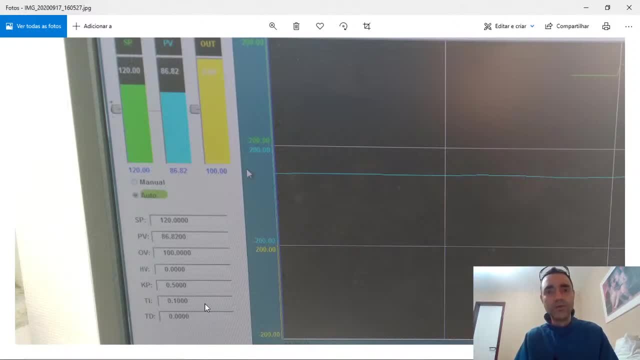 Related to PID. What I do Is add preliminary Information To the control. So in this case We started with 0.5. At the proportional And with 0.1. To the integral, And I saw The behavior. 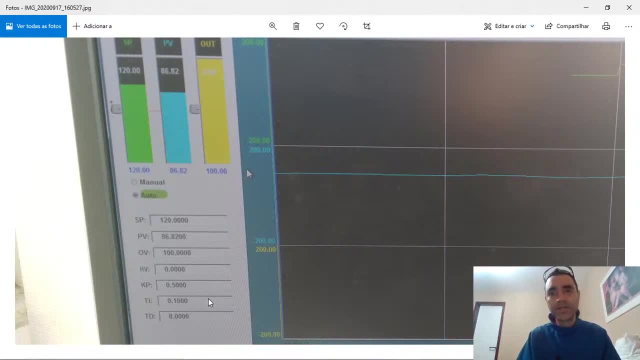 Of the control And I evaluated that For some minutes. Depends on your process. It can be 2 minutes, It can be 10 minutes. So, Based on the variation In the process, I know if I need to increase more. 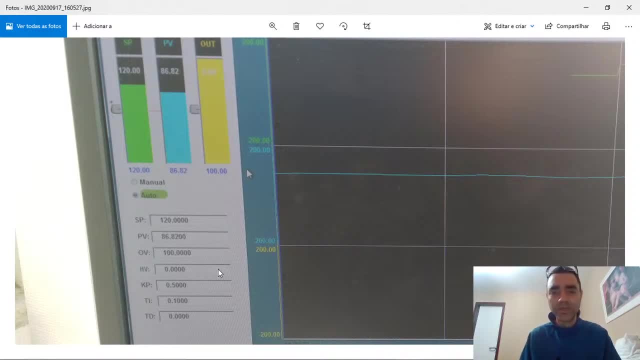 Or if I need to decrease more The information of proportional Integration, And most often You will need to work With these two, With these two Values In parallel. We Have a stable process With your P and I. 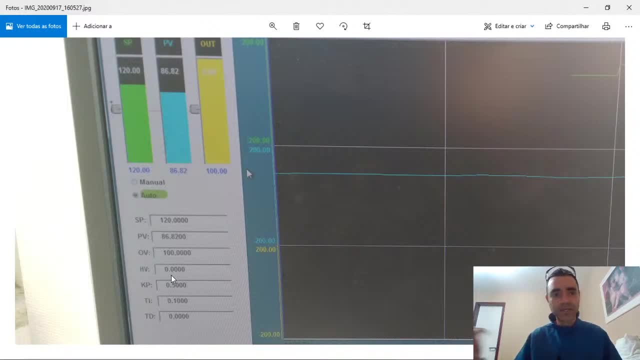 Already set And, for instance, There are disturbance, You increase the plant capacity And you don't have The same kind of control. It is not smooth. You To adjust the process, The controller Again. You need not only change the proportional. 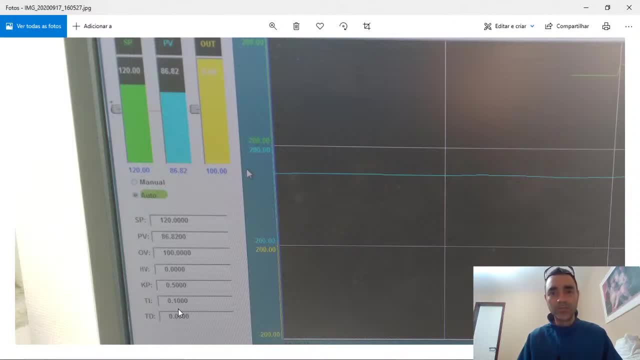 But also the integral, Related One with another. And what I can say About this Is that the proportional Is how big Is the steps Related to the opening your control valve? And, of course, guys, I'm telling you here: 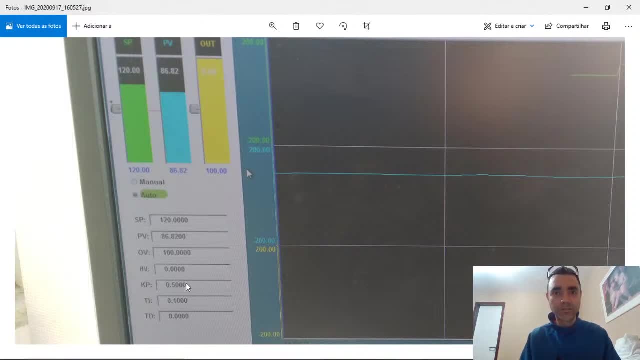 What I see In the practice. I'm not trying to be Scientifically Use terms of Bibliography. I want to show you The understanding that I get from the field, So I think it's much Easier to understand. 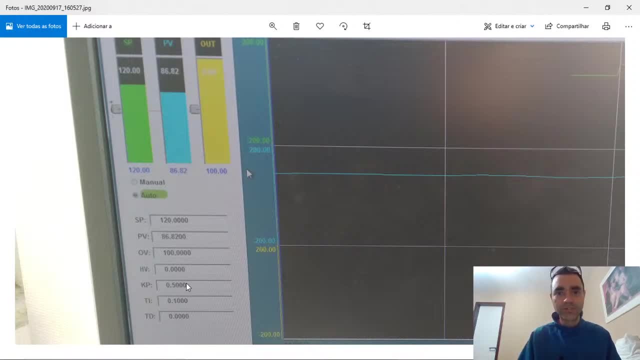 And also much useful, Of course, If you need to do a test, A test, for There is a test In India- I forget the GPA- There is a test. If you need to do a test, You should study The right. 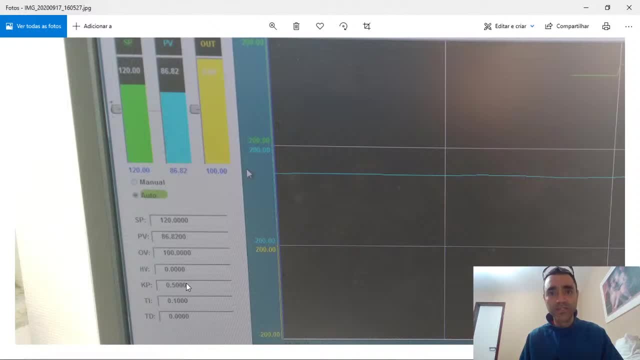 The right answer Or not the right answer, But the expected answer. So it's not What I'm doing here Is explaining to you How it works. So the proportional Will open more Or less Your valve And the integration. 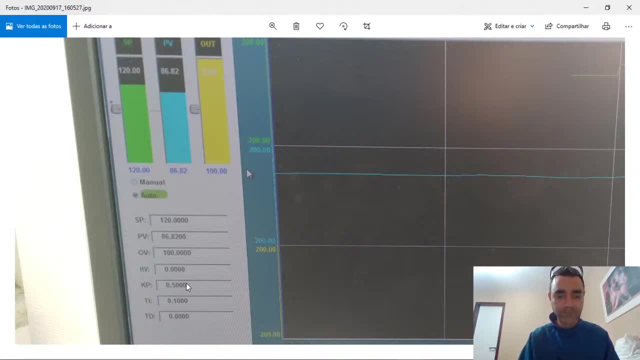 Will define How many Times That will be done By time. So if I have a P Proportional To big, It means that every time That my valve opens Or closes, For instance, If my P is 0.5.. 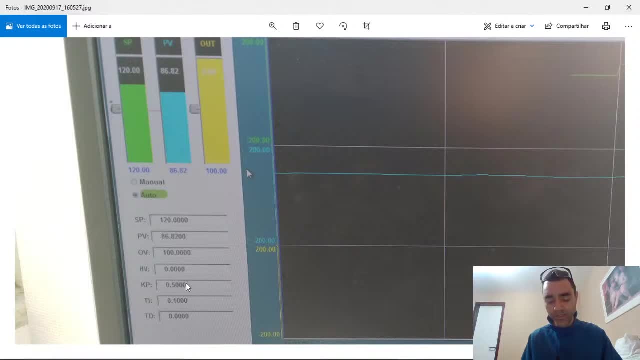 It will open, For instance, 5%, But if I add a proportional of 2. Instead of opening That, it needs to do Actuation. So what is expected Is that with high Proportional Your valve will open. 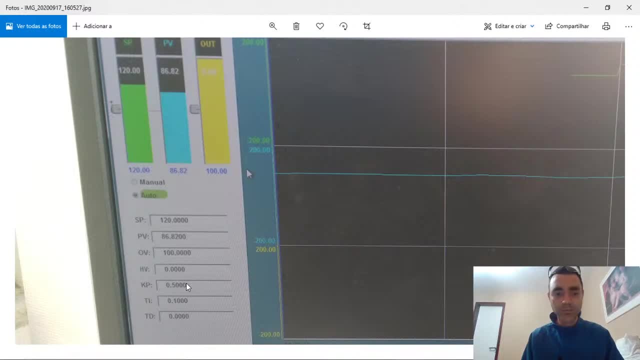 Will do big steps And with low Proportional It will do Small steps. So this is it. The integral Will define how many steps Will be done In a period Of time. So if I decrease The integral, 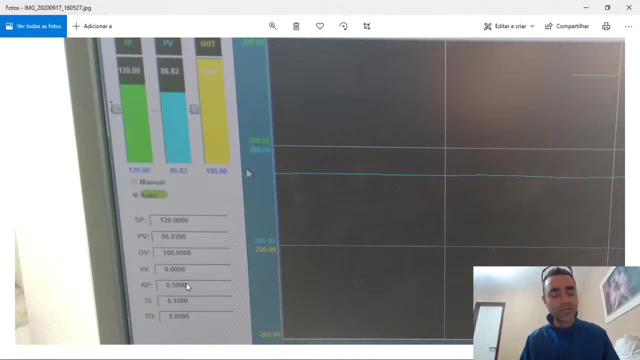 I will do. If I decrease The integral, I will do Less. Everton, Are you still there? This sometimes Is confusing, But if I increase The integral, I will do Actions In a period of time, Or I will do. 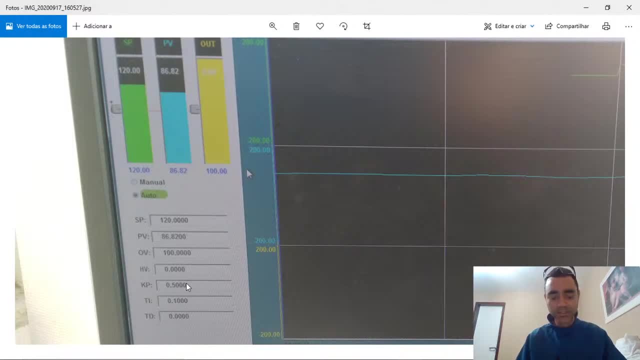 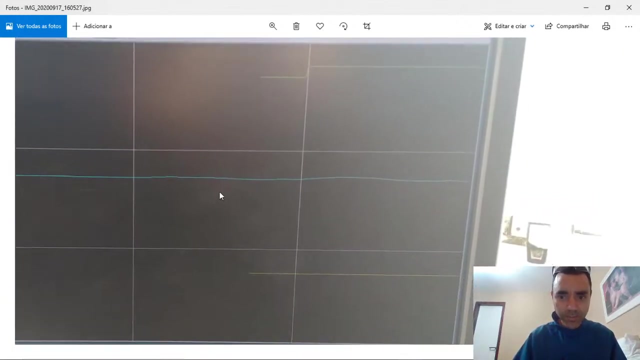 Less actions In a period of time, And this is important Because if you have A curve like this, You need to Change the proportional And the integral In order that it will Open. So What we can see here. 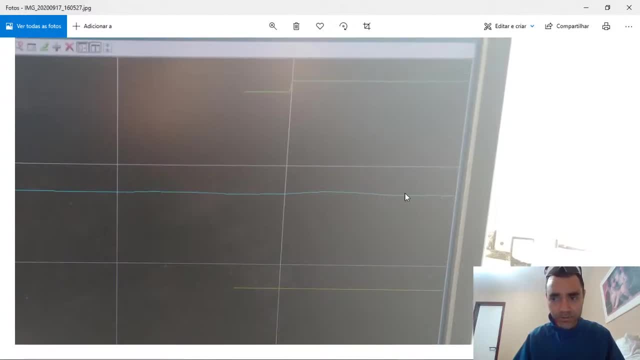 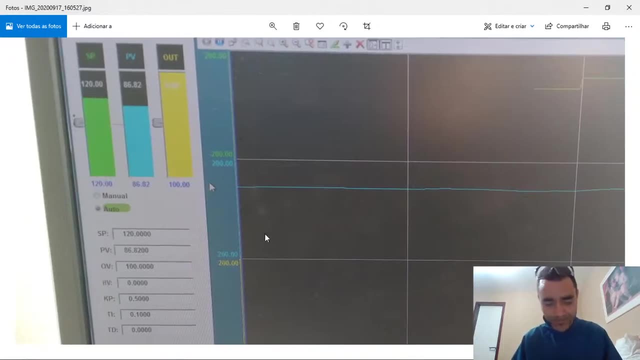 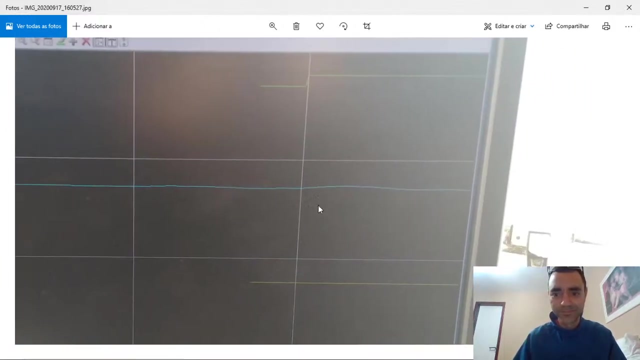 Is. It is not so good Because there is no, No much Nice Everton. Please just confirm to me: If I increase The integral, I will have more actions Or less actions Per time. So I will do. 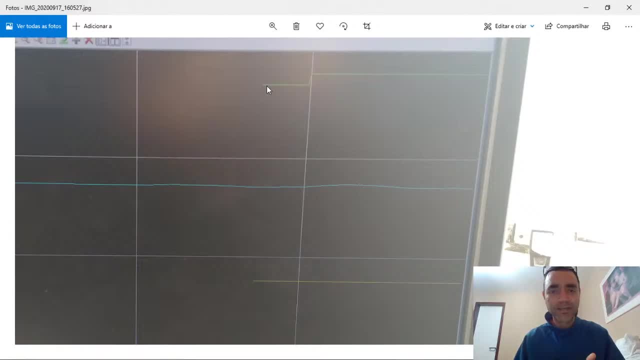 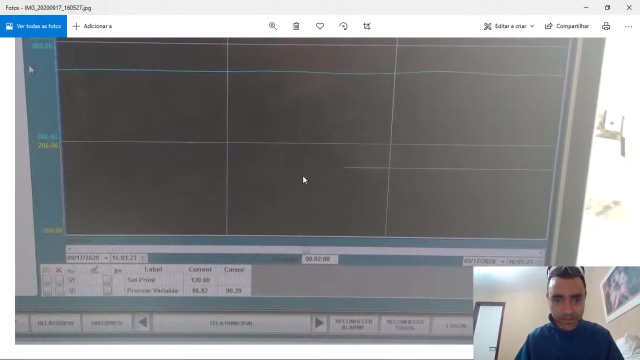 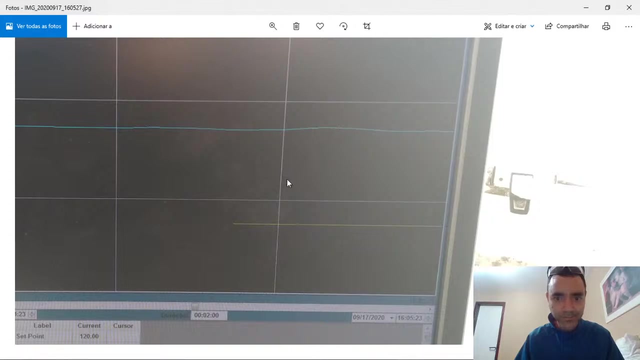 Less. actions In a period of time Is confusing, But if I increase The integral, I will do Actions In a period of time Is confusing, But if I increase The integral, I will have more actions, And it is. 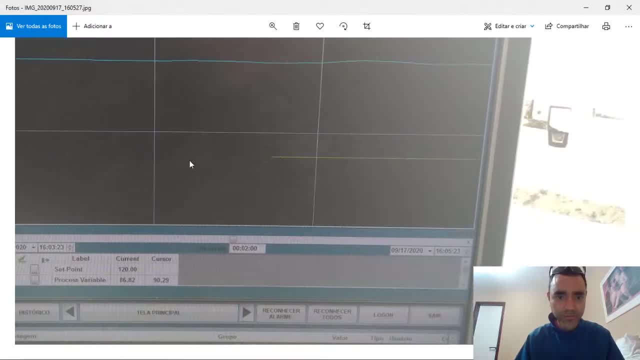 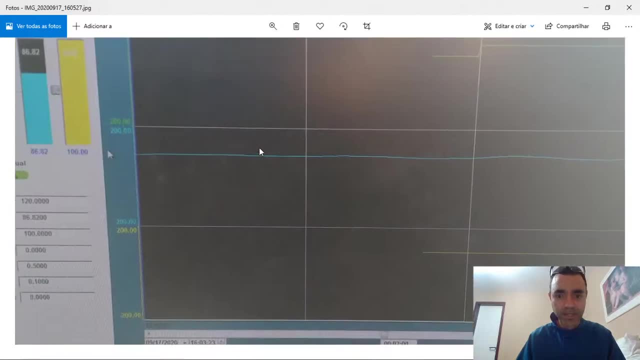 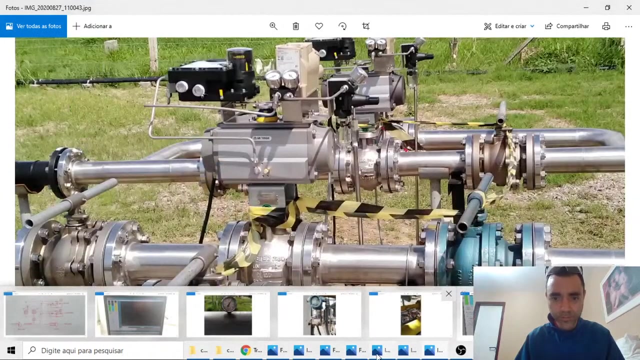 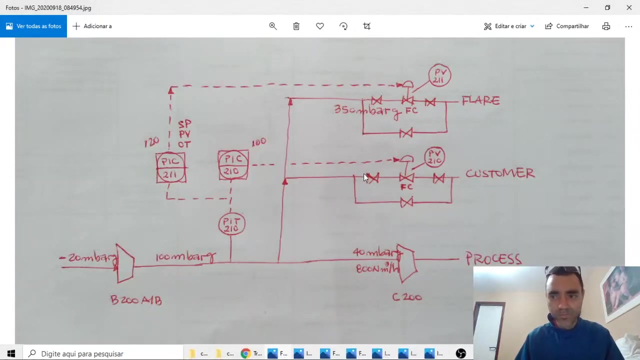 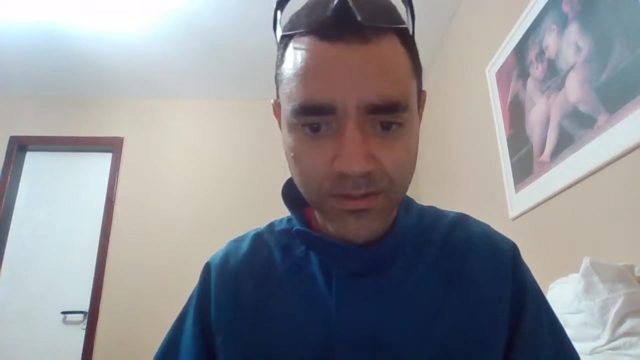 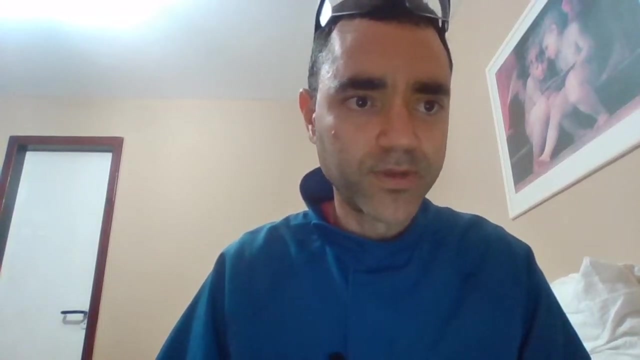 My opening Of my valve Here is not so good To see Because I don't have too much variation, But Let me see If I have Another picture to show you I have. Let me Try to find. 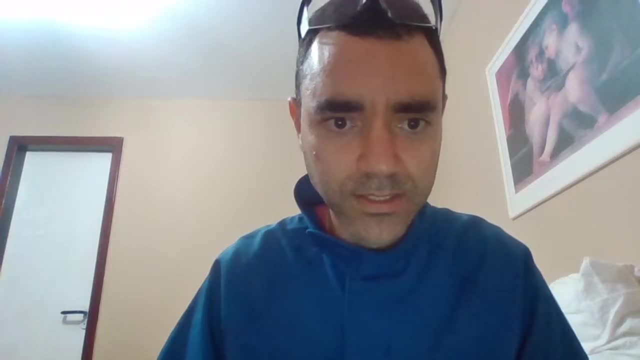 I have a video here That I did In another project. Let me see If I am able to show you, Let me. What is Now This? So I will Let me do One, One, Two. 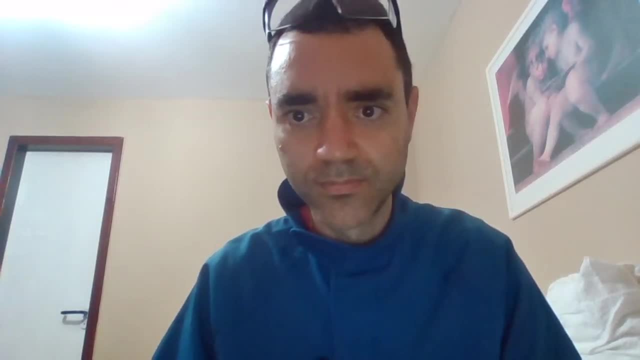 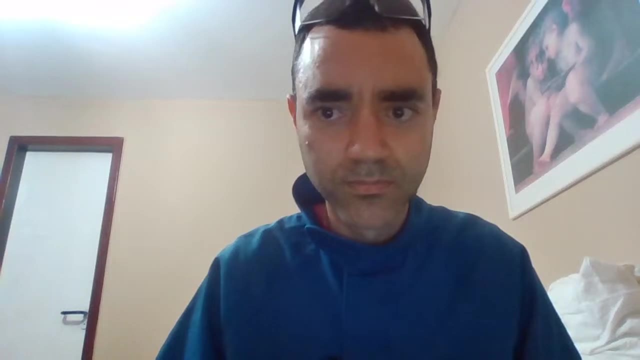 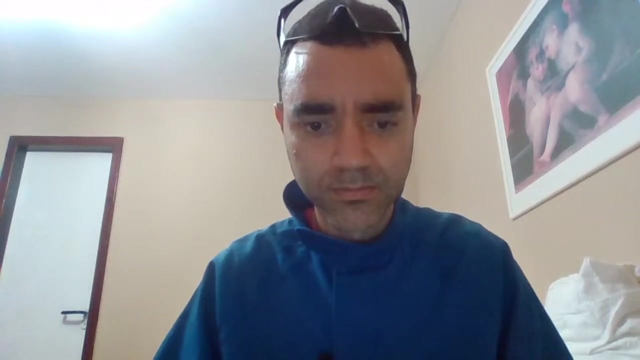 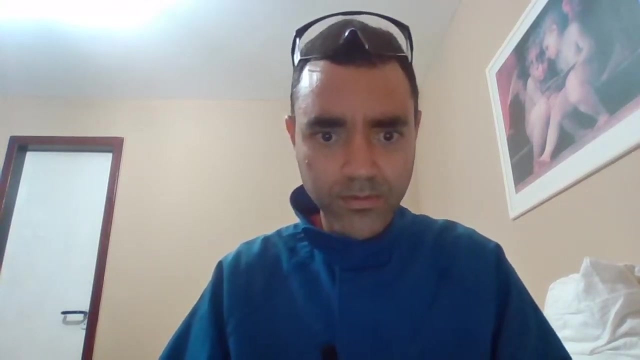 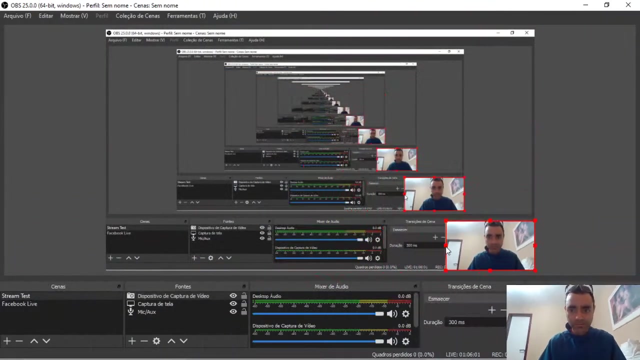 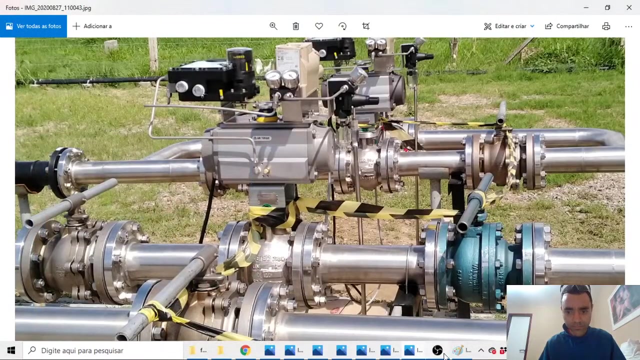 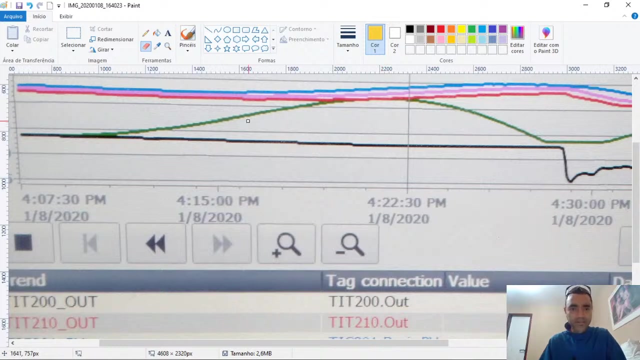 Three And Thank you, Thank you, Thank you. So here, Here I have another graph of controlling. and what, Ah, nice, Nice, What? Everton is saying that if we increase the integral action, the controller will respond faster, So it will do more actions per time. 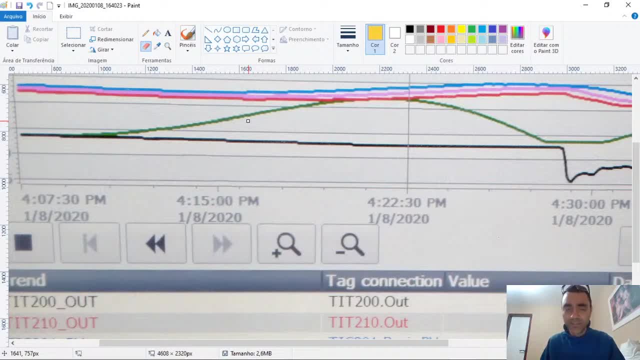 But it depends of the calculation And I have seen that In another commissioning, because Everton is saying that it depends on how is the equation. Depends on the kind of the equation. Normally we have the frequency, But if it's written differently, when we increase the integral we can. 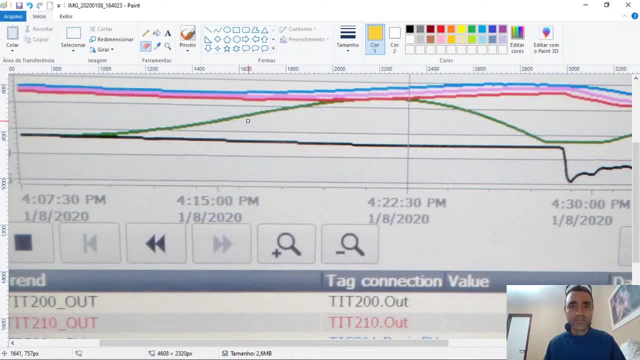 Decreasing the response. So it is something that we need to discuss with the automation guys during the commissioning. But if you don't have an automation guy to talk to you during your plant operation or something like that, what you can do is to define small steps. 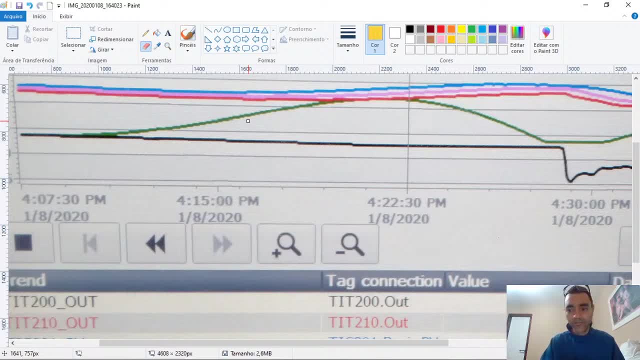 And you do a small step increasing and verify. Or you do a small step Decreasing and you verify, And you will understand if you increase the integral, if it will respond faster or not, Or if you decrease, if it will respond faster or not. 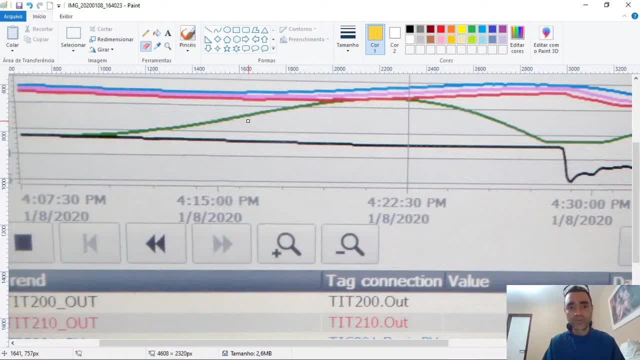 That is the safer way to do that if you don't have the support of the automations, Because the automation guys can link the computer at the system And he can Verify this kind of issues, And usually we process engineers and operators are not able to do that. 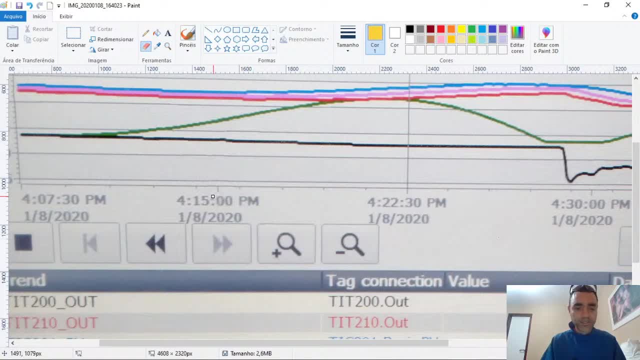 So this is my tip, And here you can see another process, And in this process the OT of my system is the yellow line. Is this line here That is touching the red line? This is a heater, And this heater is responsible to heating up the water system of my process. 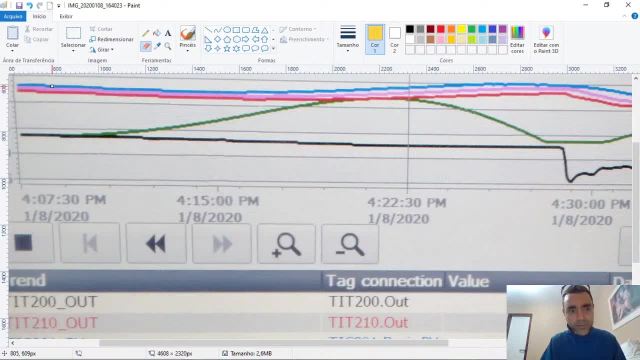 And you can see that we have three lines here And here what's happening is that the temperature is decreasing And when it gets a determinate value, the heater is starting heating up in order to prevent the temperature to decrease more and more And it gets a peak or it gets a highest value. 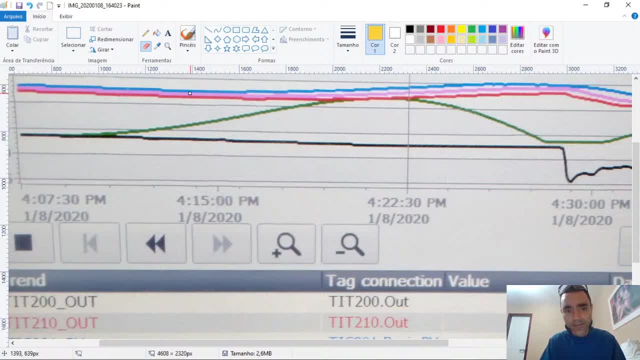 And so it returns in order that I have the modulation of the system And for me, in this case, it is very, very good And I can- I could also work more in this process in order to have a more smoothly, A more straight line. 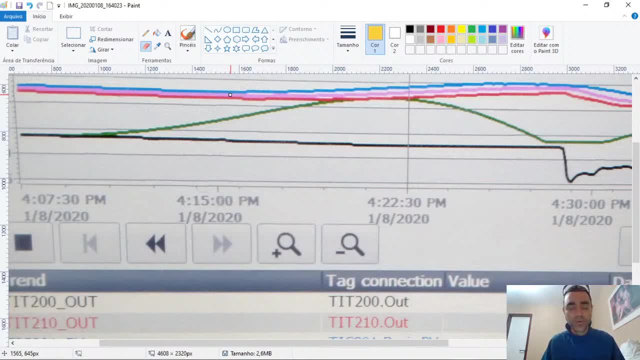 But sometimes you don't need to worry about that. You need to make sure that the minimum values that you're getting and the maximum value that you're getting is at the range of the operations, And if it is at the range of the operations, 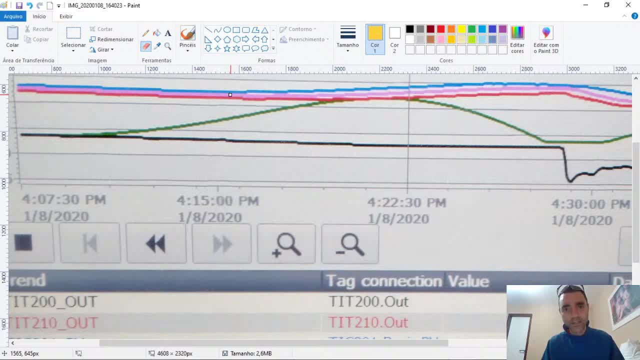 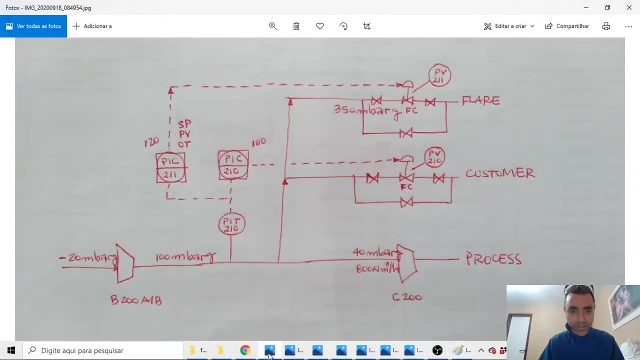 okay, great. If it's not at the range, we need to set up the tuning. Thanks a lot, Everton, And with that guys, I need to know if you have any questions that I can help to clarify. I don't know how long I've been talking. 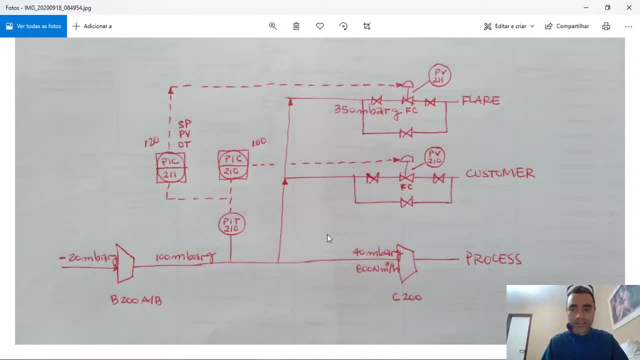 It seems that I've been talking one hour And I'm still with my suit, So I need to take some bath. So if you have any questions, please just let me know. And thanks a lot for the guys that were following me right up to this point. 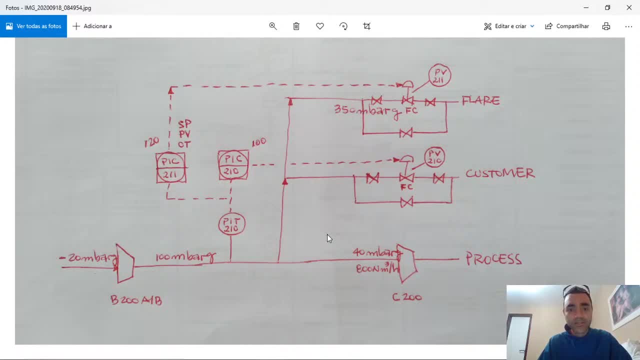 because I know that it is not an easy subject And I don't have too much resources to share with you. It's more talking And A way that I have to share with you my experience without doing a classic teaching. I'm not. 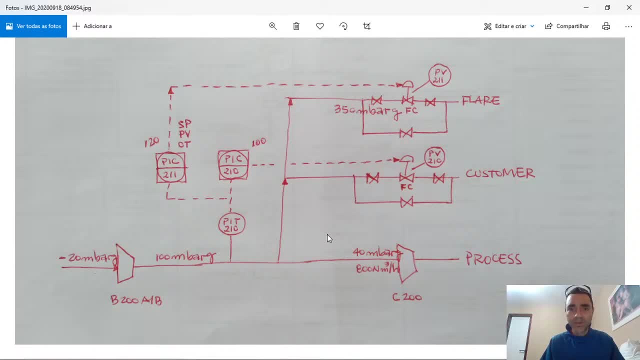 It's not my way of teaching people. I'm not a teacher, although I'm working more to prepare myself better to do classes. I'm not a teacher And I try to share with you what I know from the field and from my experience. 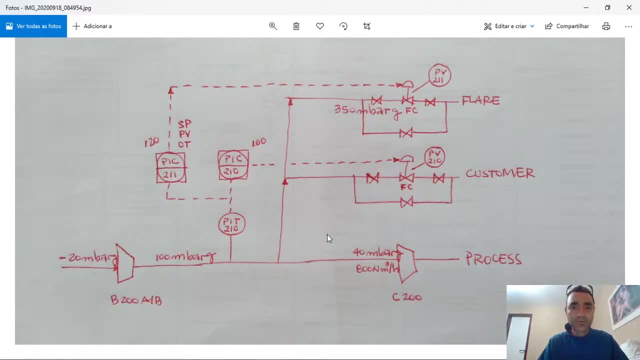 And this kind of live session is to do that. So, guys, I'm very, very tired, For sure. So my dinner was this- I'm not so sure if I have talked to you- The pizza and citrus. If you don't have any question, I'm going. 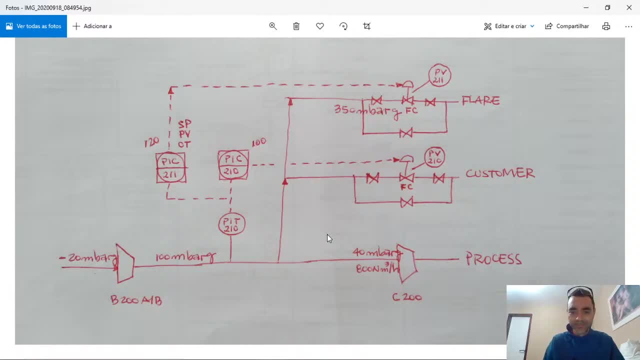 Let me know if you are still there. Thank you, Josmea. You are supposed to do the tuning of your process during the commissioning, because what we do at the first time, we- What is the sequence right? We do the process simulation. 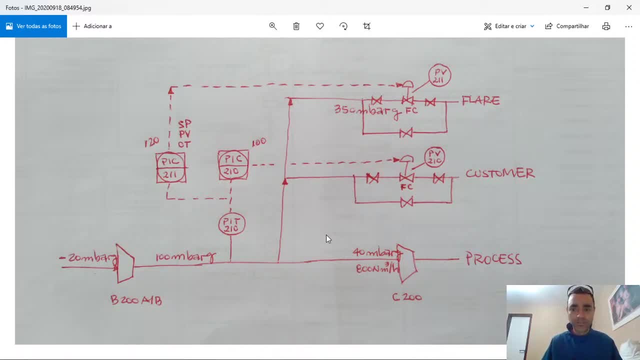 Based on the problem that we have, we do the process simulation And once we do the process simulation, we have the process conditions to define our control valve. We We develop or we fill a process data sheet or a specification data sheet And with that data sheet, 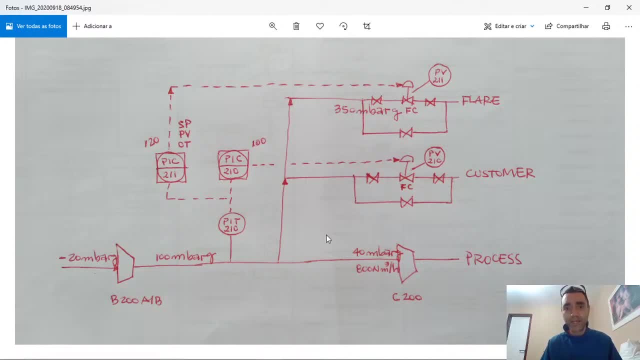 we are able to do the preliminary sizing or preliminary selection of the control valve. Once we do that and the process and the project proceeds, we do the quotation and the procurement team by the control valve It is sent to the field for installation and it is during the construction phase of the project. 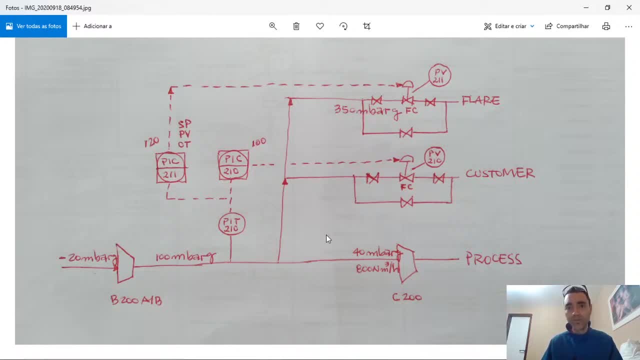 And once it is installed and with all the connections ready like electricity, instrument, air and stuff like that, everything is OK. it's time for commissioning. In the commissioning it starts with defining or verifying if the fail-safe conditions of the valve. 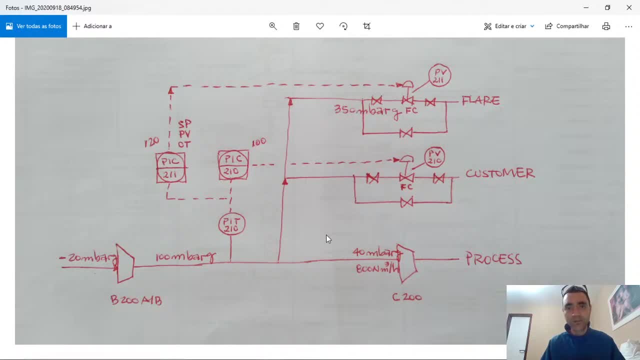 is, was mounted correctly Because, depending on how you set you connect the air supply to the valve, you can change the fail position of the valve, depending on It depends on the supply of the valve, or something like that. So, And once you verify that, 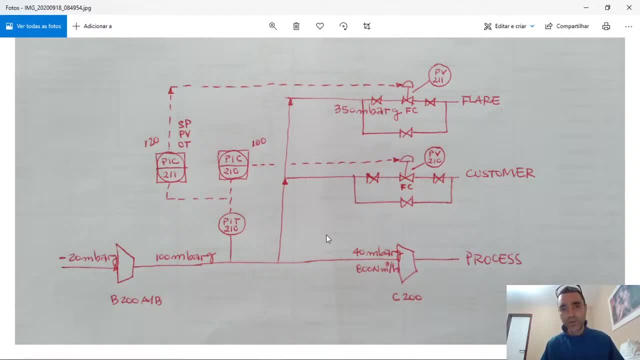 the instrumentation guy and with the support, with the automation guy and with the process. in many cases we verify the zero, the 20%, 25%, the 50%, 75%, 5% and 100% of the valve. So 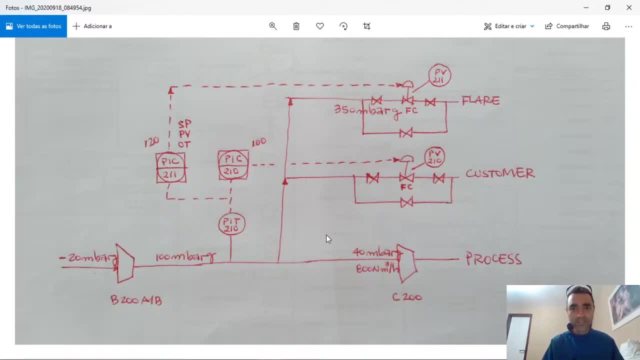 we send an electrical signal that represents these openings and we verify at the field if the valve is opening correctly and closing correctly based on that, And we verify not only the field, but we also go to the control room and verify if the 25% opening 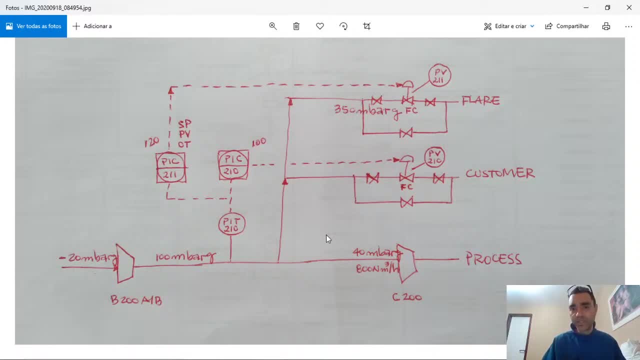 in the control room is 25% opening in the field or something like that. It is the commissioning, because the valve is already installed. OK, So we are doing tests before doing the startup of the plant. So commissioning is it. 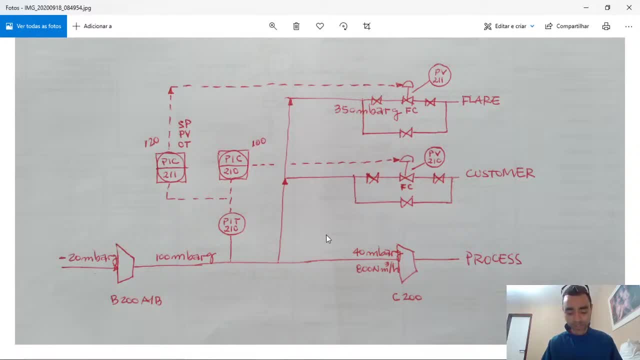 doing verification before the startup of the plant And once we start the And before starting the plant, we add preliminaries values to the PID of the in the controller And we are not sure what will happen because to see the valve actuating, 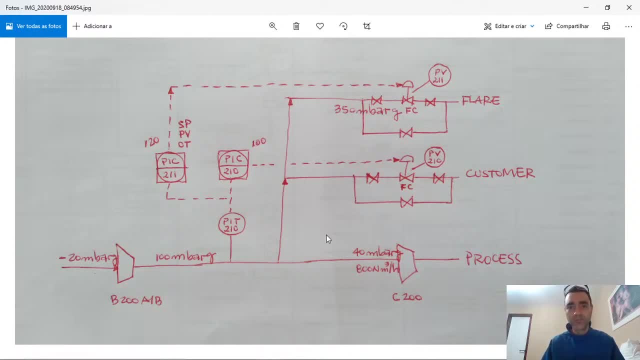 we need to have flow through it. If the valve stops, we are not able to evaluate the PID of the control, Unless that there are software that are able to do that. I never worked with software OK, So I cannot say if that is possible. 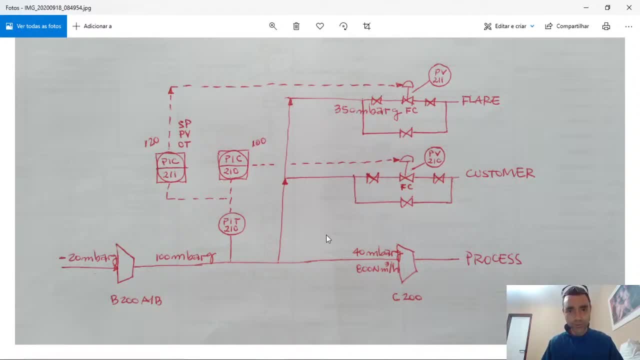 Eventually, with my live session with Everton, we will know that. So when we start the plant and let's talk about the control, The pressure controller that we are talking here- I will evaluate if the operating pressure is at the range that I want to. 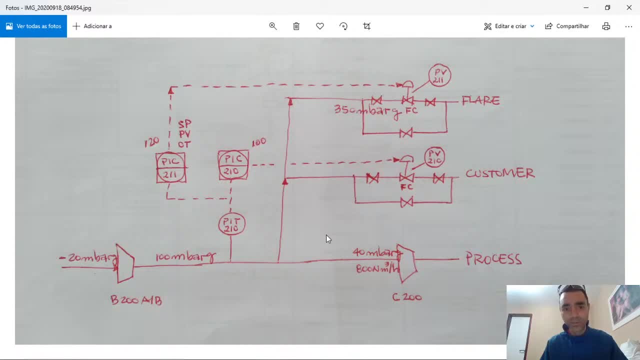 And I set my controller to 120.. And at least my average. My average present value should be 120.. But I don't want too much variation. I don't want a solenoid. I want, I don't want. I cannot use it. 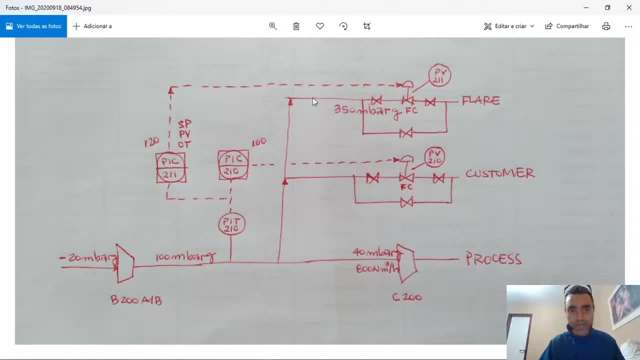 I don't want a solenoid, I want a straight line. And to have this straight line, I will adjust the proportional, I will adjust the integral And in some cases, not pressure, because we use derivative when you have a lower response in your system. 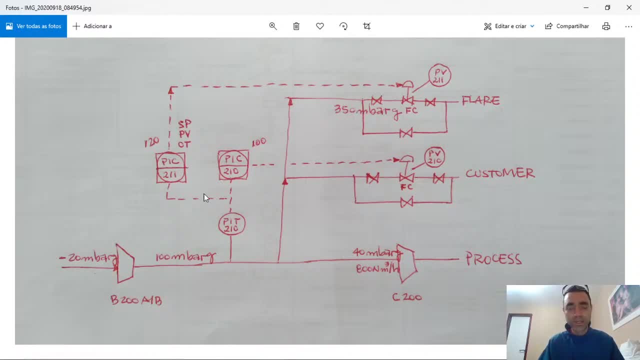 So in many cases we just need the pressure proportional indication. We will adjust that until we have a smooth graph of variables and open. The actuation of the valve is not so important as the present value, So what matters for us is the present value. 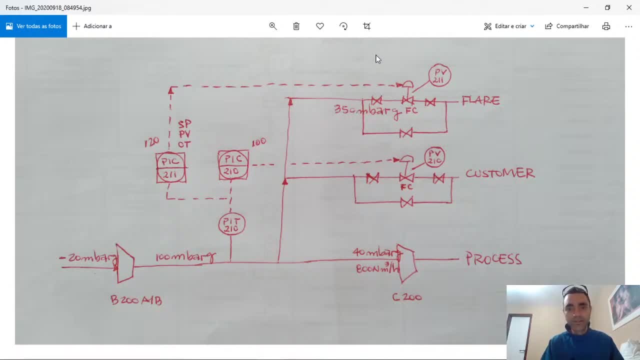 And once we have that, we can, And it is during the startup, because I'm not able to do that if I don't have gas passing through- And in many cases we will not pass a gas- only to do the tuning You will do during the startup. 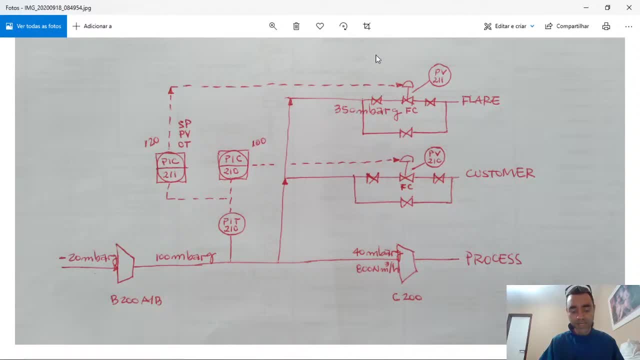 of the plant And most cases we start with low capacity or downsizing, And what It's not downsize that we- I forgot the term that we use- But we start with low capacity and we start doing the tuning of the controllers. 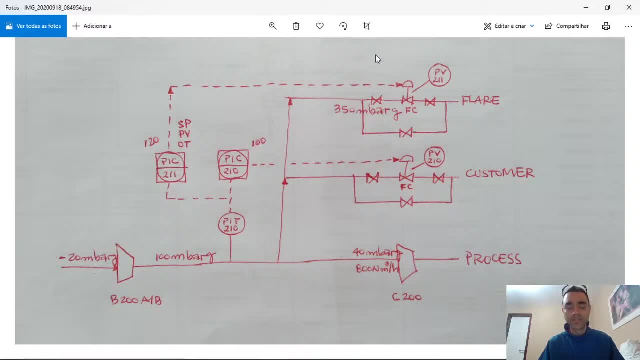 And once we increase the capacity of the plant, sometimes we need to change that until we have 100 capacity and we set the tunings And if we have too much variation, the tuning should be able to support that kind of variation or something like that. 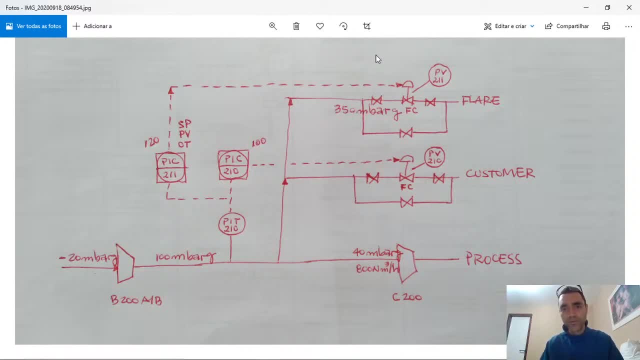 So the tuning, in my point of view, is not Is an activity that begins in the commissioning, but it extends to the startup of the system, because without the startup we are not able to finish that Okay And eventually. 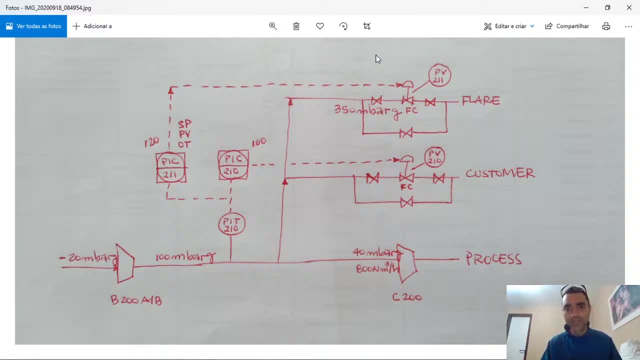 if you are already in a plant that is running. if you change one condition it is possible that you need to change your tuning again. For instance, you run with one pump and now you are running with two pumps in parallel, So the system behavior changes. 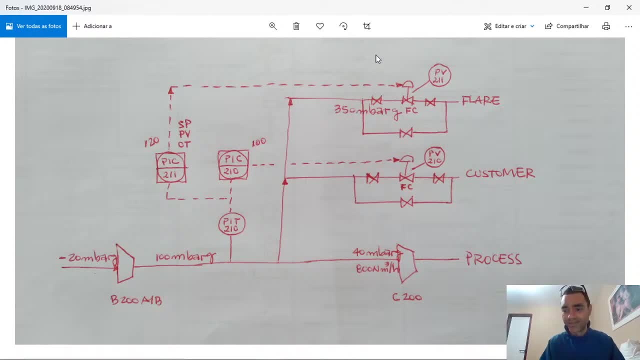 and you need to set your tunings again. Thanks. Thanks a lot for your question And thanks a lot for being with me up to the beginning. And is it by hand or software? Yes, Akshay, All this is as chemical process engineer. 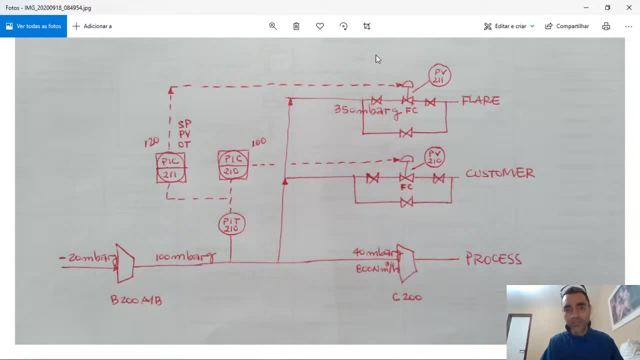 And, as you already know, I worked not only in the office but also in the commissioning in the startup. I always did that by hand. I know that there are softwares that do this kind of calculation. I don't know how expensive it is. 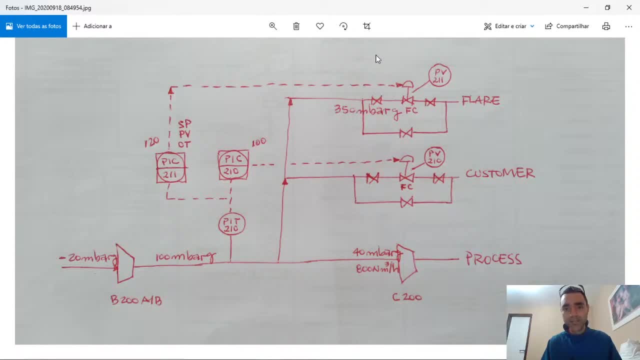 but I believe that. I believe. no, I do that by hand. Okay, So I have worked with small plants and with average plants. I never worked with petrochemical plants, So I, And as the size of the plant increases, 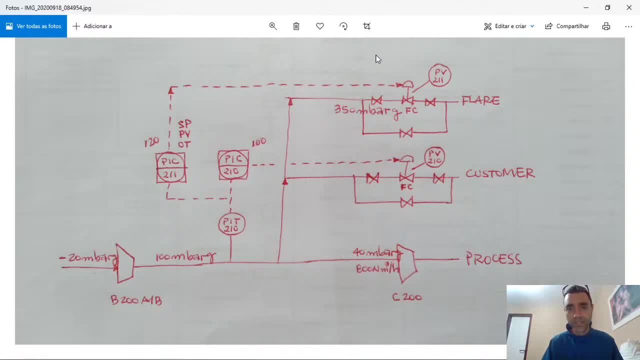 of course, that the money available to do commissioning, to do the startup, increases. So eventually in these big projects you will have capital to buy automation about this. But I always did this by hand And I know that there are. 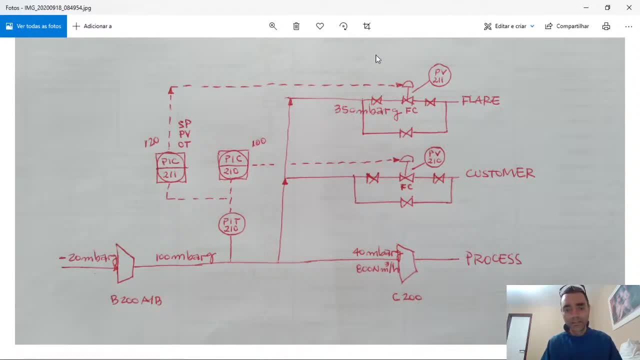 algorithms and the air separation units. has this kind of Oh, Ah nice. Let me read here for people- And Everton is helping us- There is software to PID autotuning. In general, these softwares are expensive and I prefer to calculate the PID parameters. 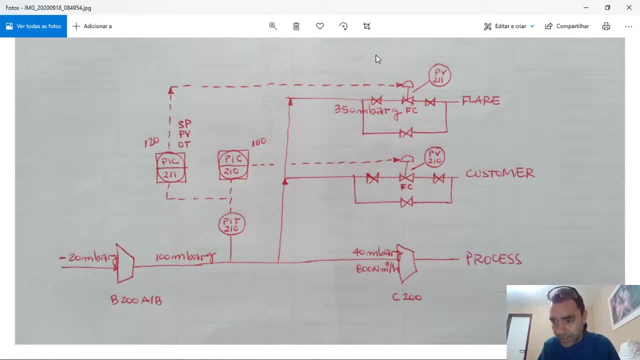 You have to define the first-order dynamic model to calculate the parameters. So this is the way that he does. For a process like this, a first-order dynamic model plus depth time fits very good to a real dynamic response. And once you get familiar, 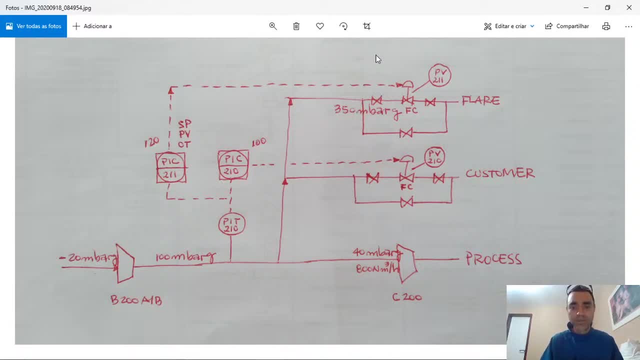 with more and more process you understand what kind of first values can be guessed, And Everton works specifically with automation So he is much more familiar with the calculations and stuff like that. I never worried about this kind of calculation And I do by observation. 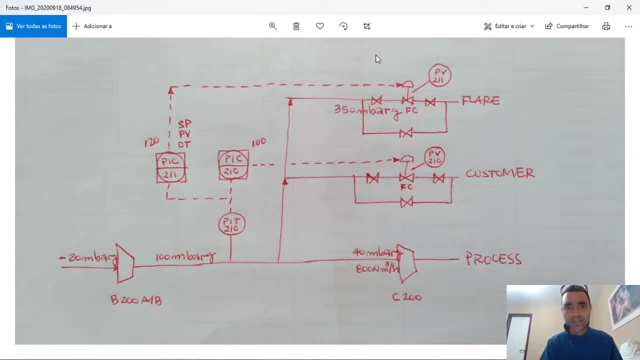 And in fact for me it is the funniest part of the job, because I can change values, I can evaluate the system and I can do correlations. I see that this valve, If this valve opens too fast, I can see the interaction. 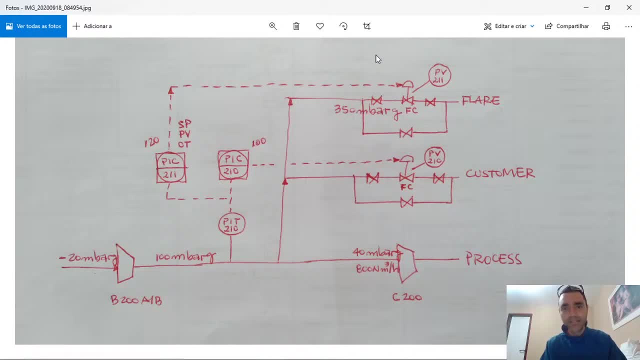 or the impact that it has in other values or other process values. So this is important to the process engineer to understand what is the relationship between one variable and another. If I increase the pressure, what happens with the periods of my gas? or if I decrease the temperature? 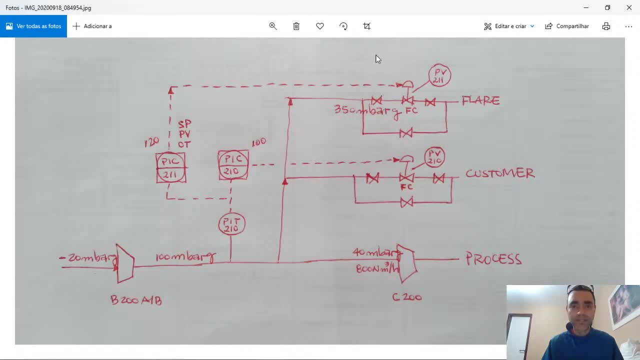 what happens with the pressure and stuff like that. So this is I like to do. This part of the job is very nice, And this is only possible if we go to the field or if you work in an industrial plant. We are not able to do that. 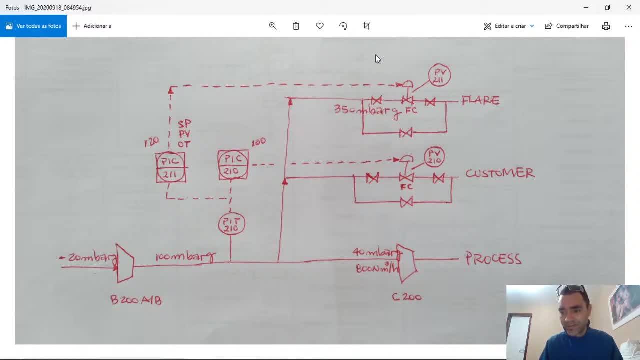 when we are at the office. So, guys, thanks for your interaction and thanks a lot, Everton. We deserve to do a live session to talk specifically about tuning of controls, And I hope that we can do that soon, very, very soon. 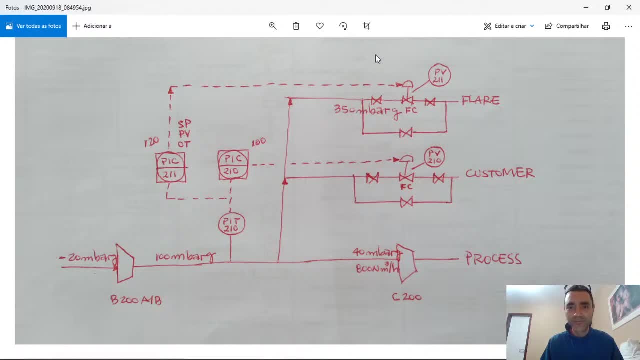 And when I say soon, it's in October, next month, Next October, No, in November. In November I will have a set of schedules open And it will be very nice. And thanks a lot, my friend. Thanks a lot for the audience.